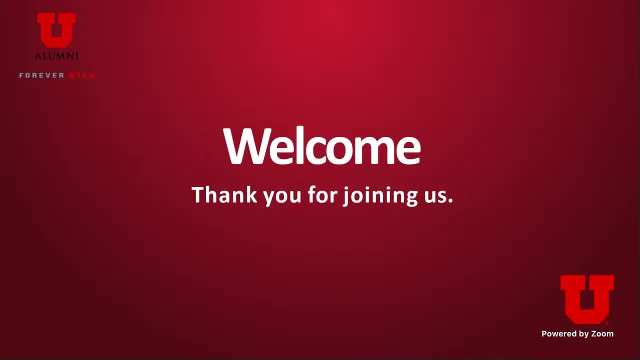 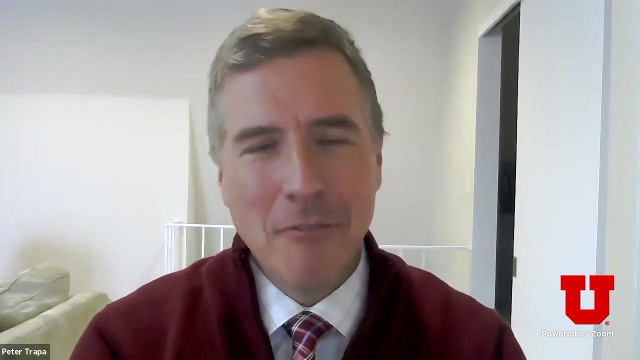 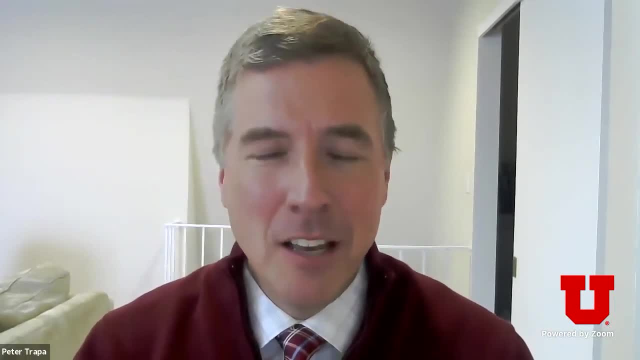 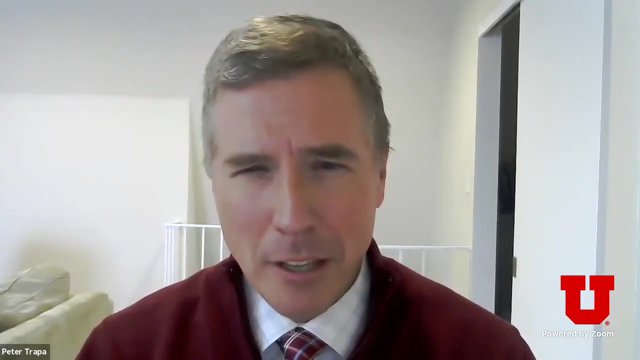 As many of you know, the Frontiers series was conceived over 50 years ago by Pete Gibbs, who was then chair of the Department of Physics here at the? U, And in the intervening years it's featured a number of very distinguished speakers from all over the world, including something like 23 Nobelists. 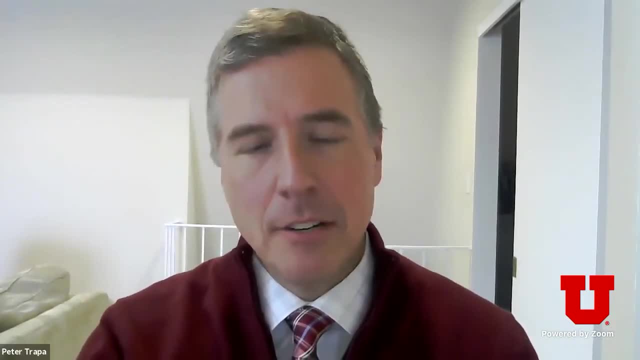 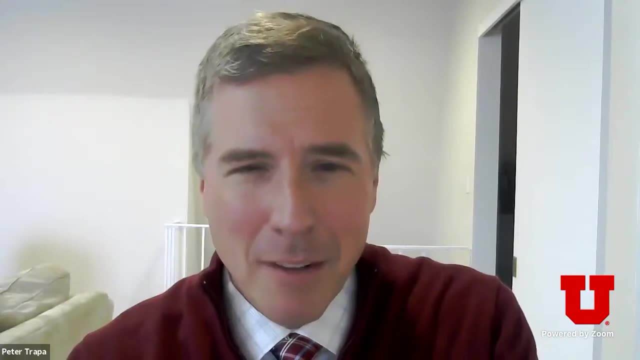 I think have spoken in the Frontiers series. This year we're doing something a little bit different because of the challenges posed by the pandemic. We're partnering with our friends in the Alumni Association and we're focusing on our own researchers in the College of Science. 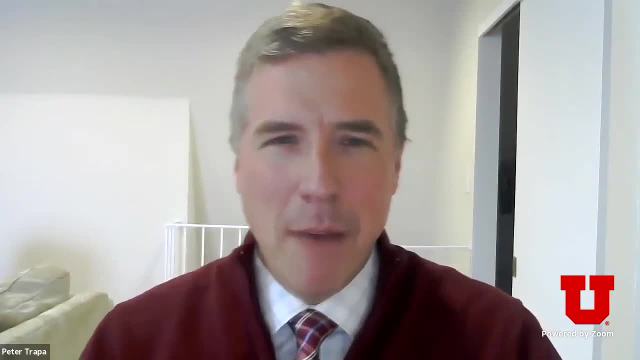 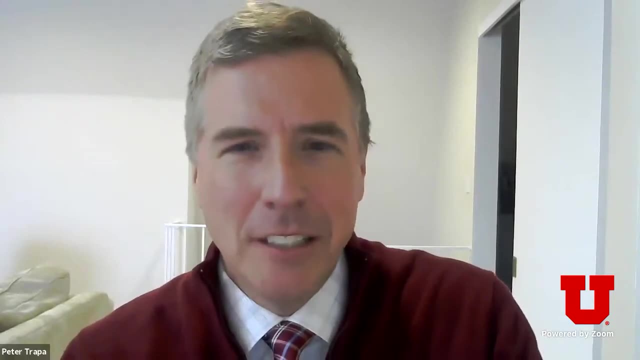 And today we have distinguished Professor Ken Golden from the Math Department, who's going to be talking about modeling sea ice and warming climate. I want to give Ken a proper introduction, But before I do that, I want to tell you a little bit about the format of today's hour. 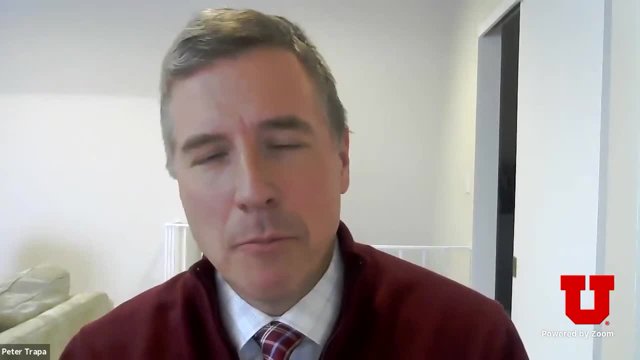 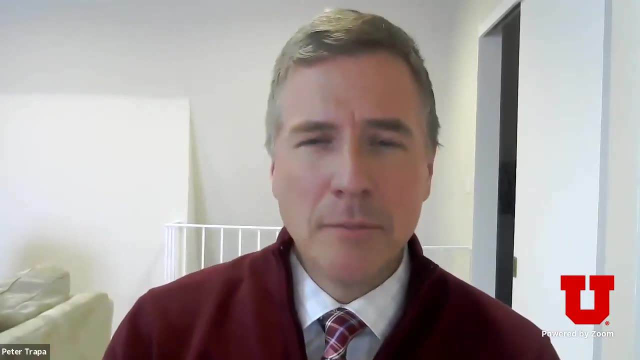 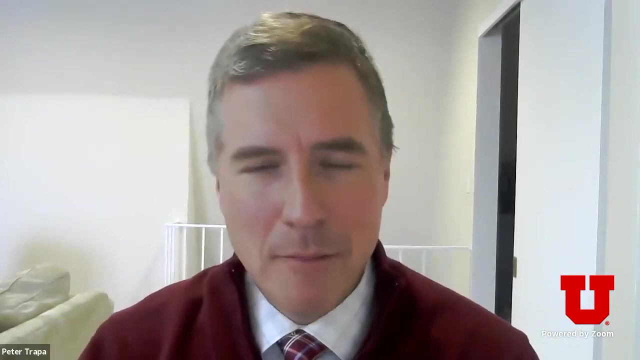 So after I make my introduction of Dr Golden, we're going to play a brief video about six or seven minutes that gives you a nice overview of Dr Golden's work, And then, at the conclusion of the video, I'm going to turn it over to Dr Golden, who's going to make a slide presentation- 25 or 30 minutes. 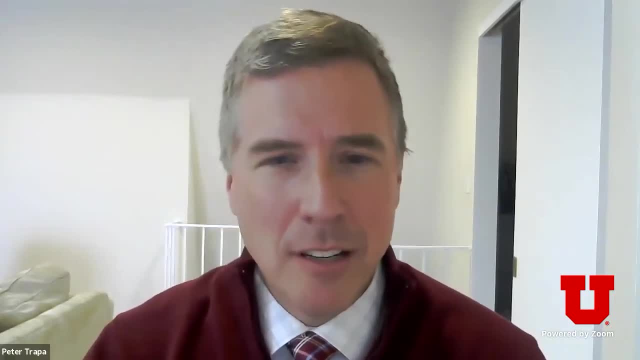 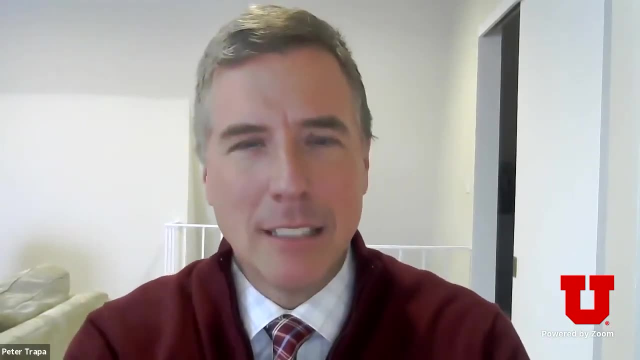 And at the conclusion of that, we'll have a Q&A conversation where we can drill down on a few topics, And then, at the conclusion of that, we'll have a Q&A conversation where we can drill down on a few topics. So, with that format in mind, let me turn to telling you a little bit about today's speaker. 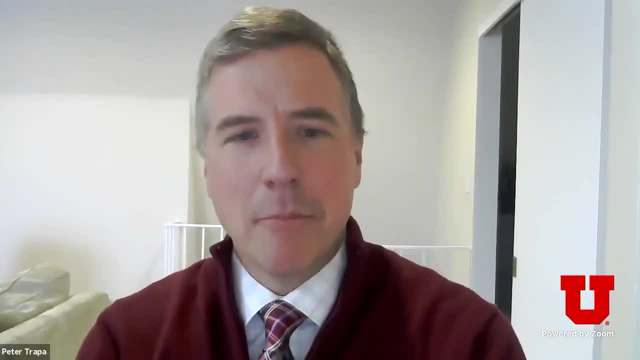 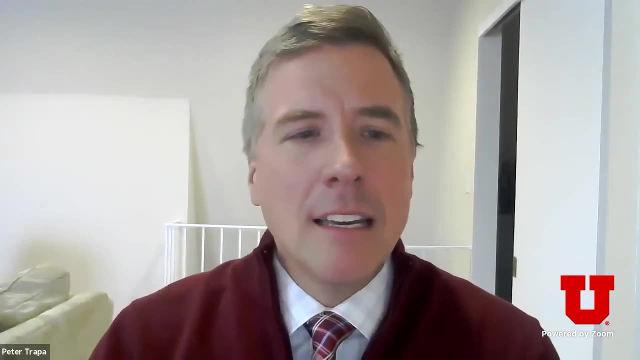 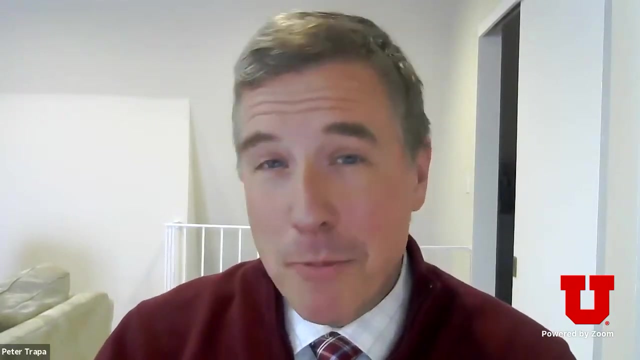 Ken Golden is a distinguished professor of mathematics and an adjunct professor of biomedical engineering here at the U. His research is focused on developing mathematical models of sea ice, and the techniques are inspired by the theory of composite materials and statistical physics. But he's no mere theoretician. 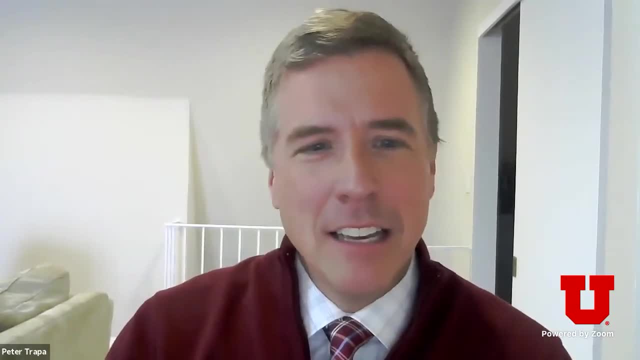 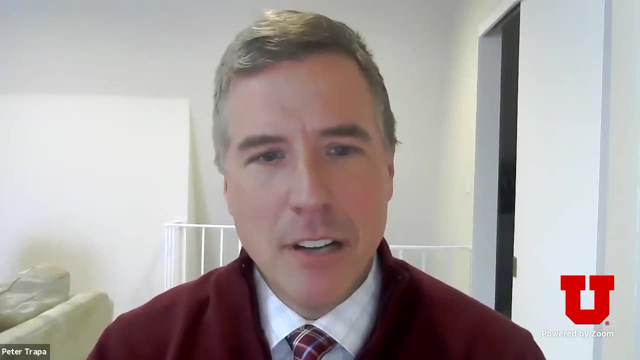 He's traveled 18 times to the Arctic and the Antarctic. He's traveled 18 times to the Arctic and the Antarctic. work has been published in a very wide range of scientific journals. Golden is a fellow of the Society for Industrial and Applied Mathematics. He's an inaugural fellow of the American Mathematical 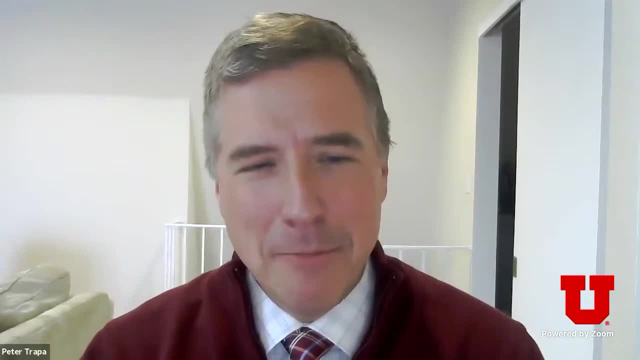 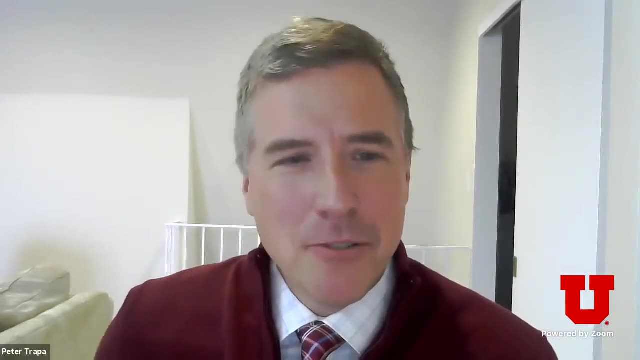 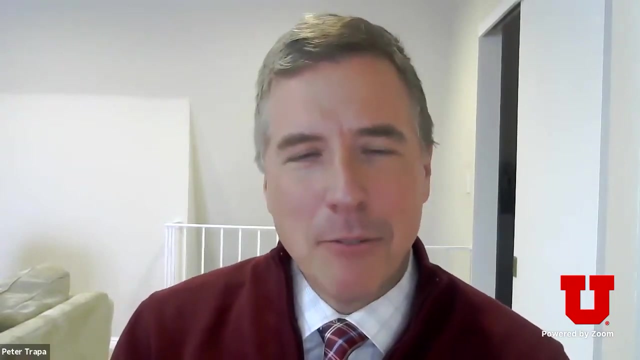 Society, and he holds the unique distinction as being a mathematician who's a fellow of the Explorers Club. This elite group has members that have included Neil Armstrong, Sir Edmund Hillary and Jane Goodall. We'll hear more about Ken's exciting explorations in the Arctic. 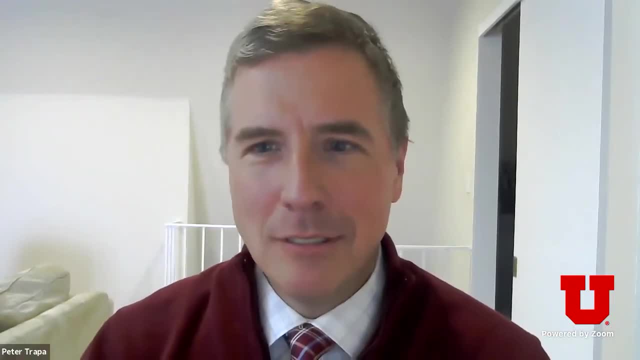 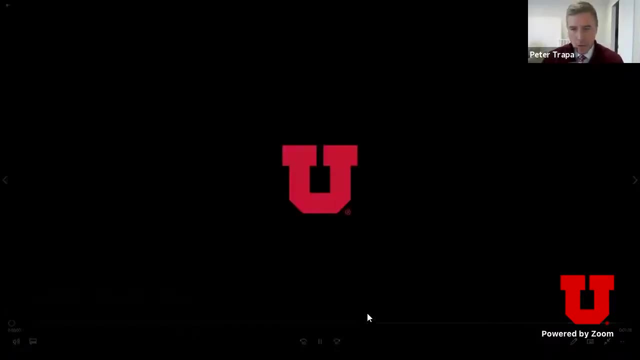 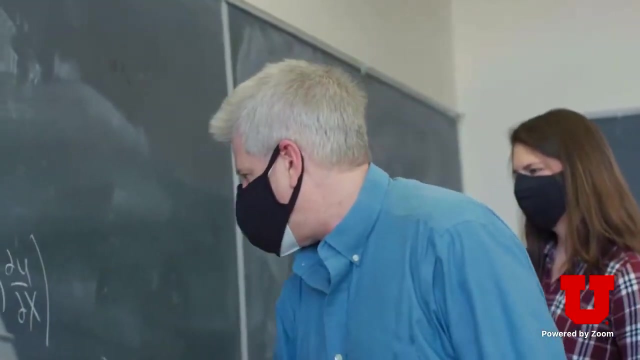 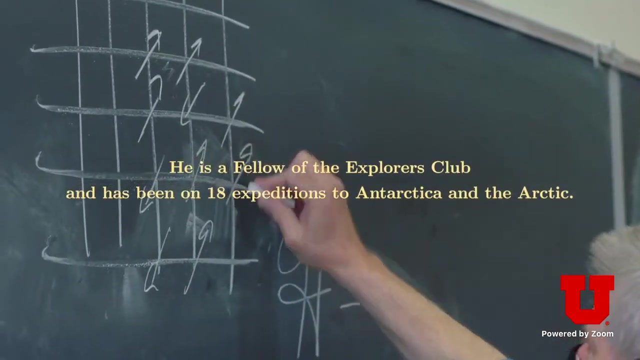 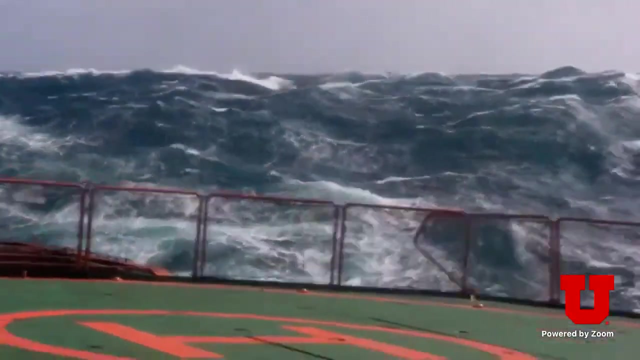 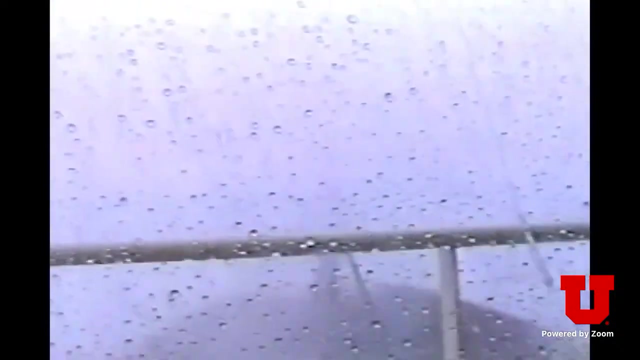 in this video. So, without further ado, let's queue up the video. It's quite a trip down to Antarctica. The Drake Passage is one of the stormiest seas in the world: Very high winds, very high waves, big storms that can last two, three, four days. 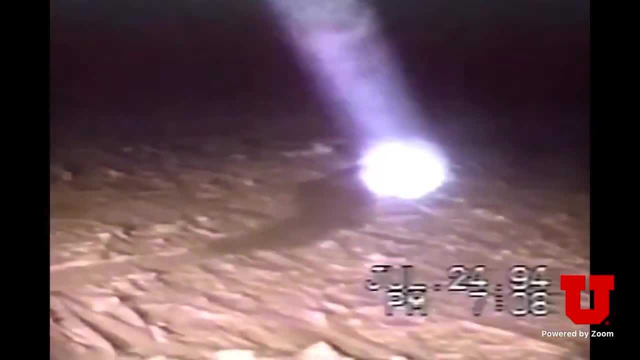 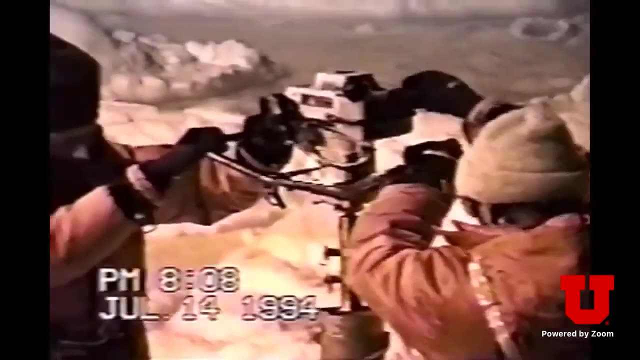 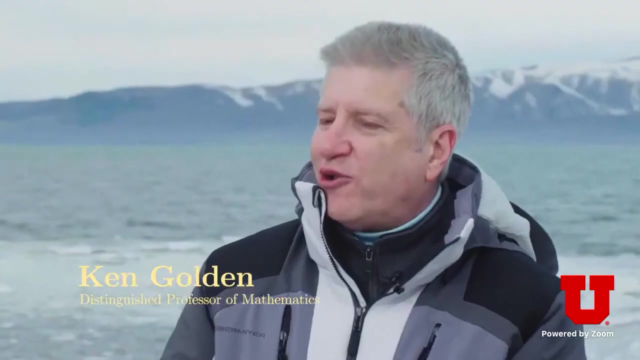 We were going into the Eastern Weddell Sea, There was a very small lead that had been created by the ship and we wanted to do very precise measurements of the thickness of the ice as it fell. So we formed in that lead. The ice was very thin. This is frozen seawater which is laced with fluid. 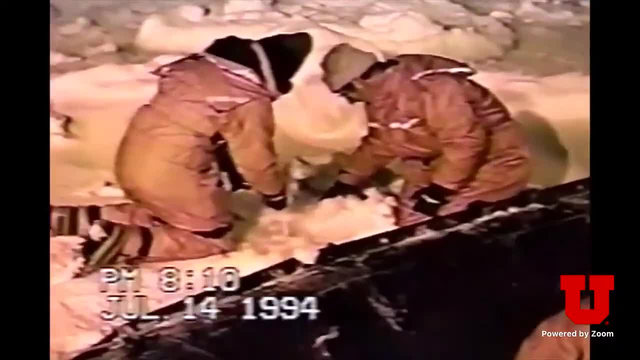 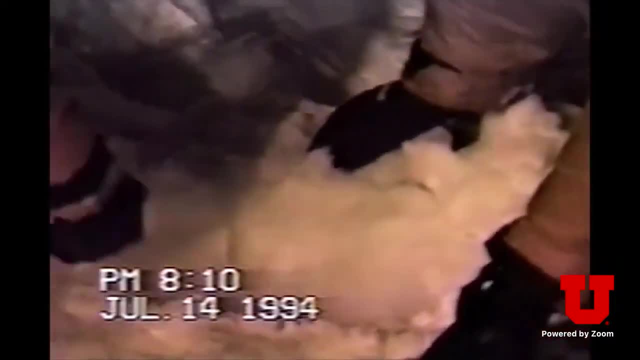 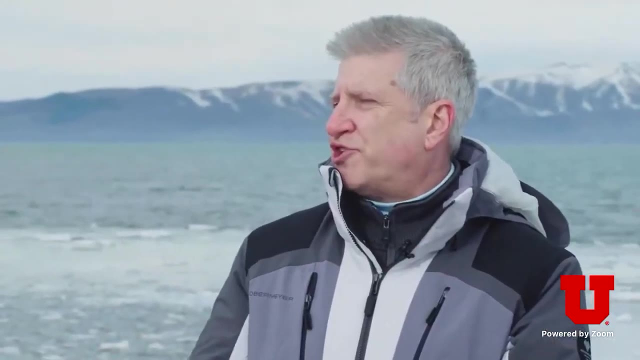 inclusions. It's not just solid ice. The idea was for my colleagues to hold my legs as I laid out on this very thin ice to do the measurement. If you go through, there's two main dangers: You'll die within a minute or two just from the sheer temperature of the water. but the main 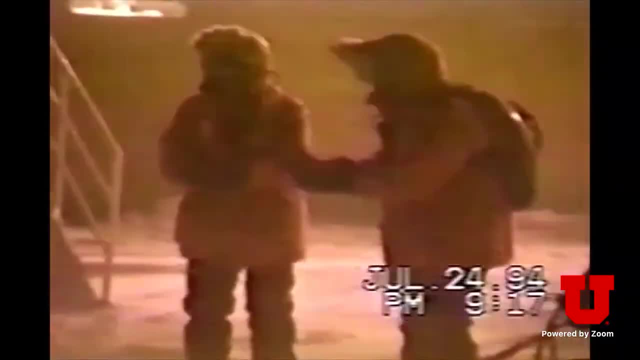 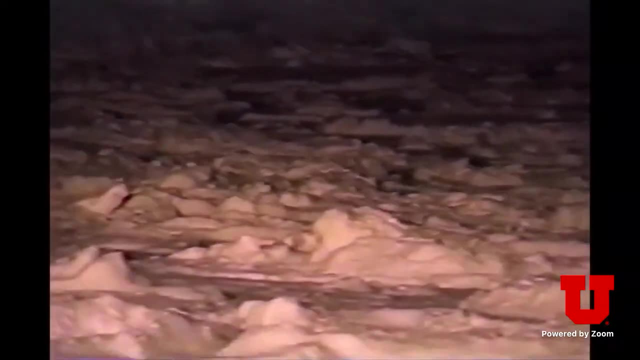 danger in this particular case was that we were in a big storm. The winds were blowing 50, 60 miles an hour. The ice was moving at about one meter per second relative to the water, So if you go through, you're gone. The hole's gone. 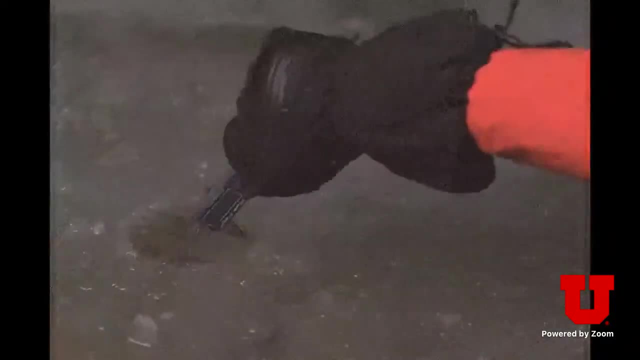 I knew that I was in a very precarious position. Then they slowly pulled me back. Then, when I looked at the instrument, we realized the ice was about seven centimeters thick. In hindsight you realize, well, maybe that wasn't the smartest thing to do. 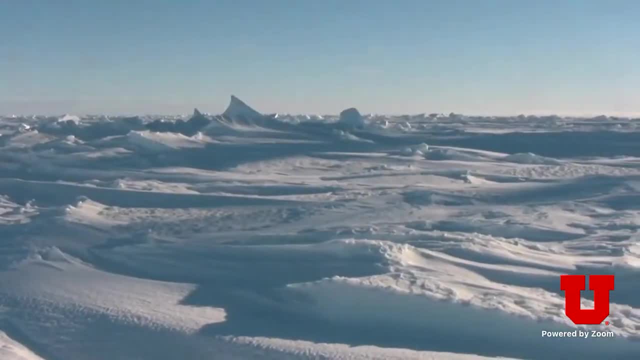 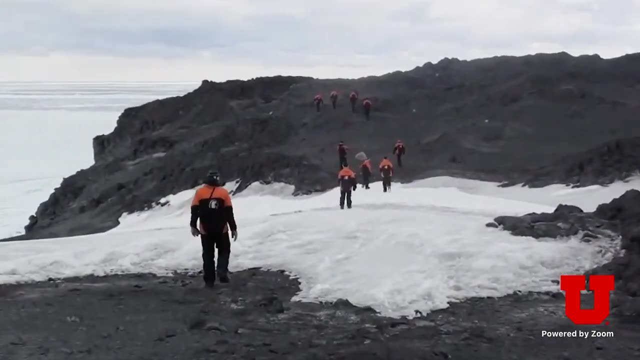 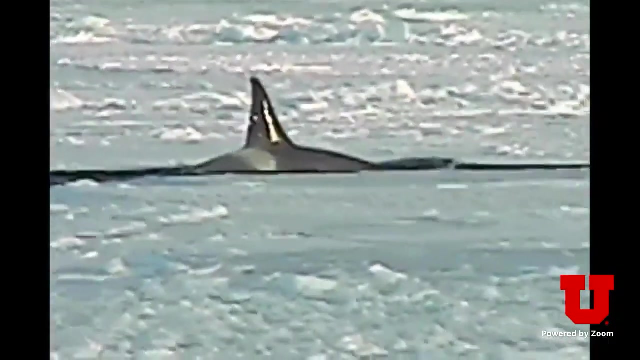 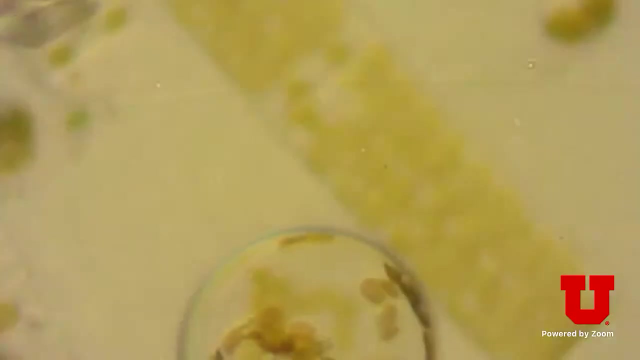 When you get down there, all of a sudden you realize it's like a different world. There are Adelie penguins, emperor penguins, killer whales, minke whales, Weddell seals At the smallest scales. inside the brine inclusions in sea ice there are algae. 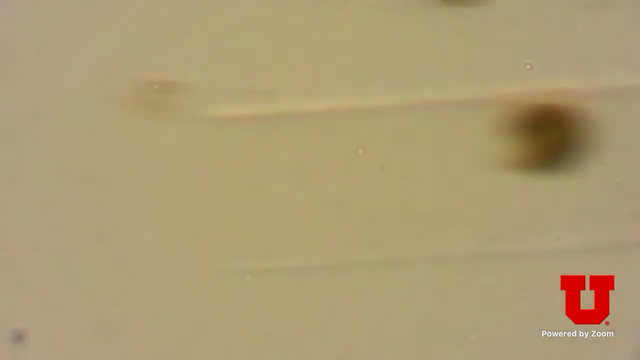 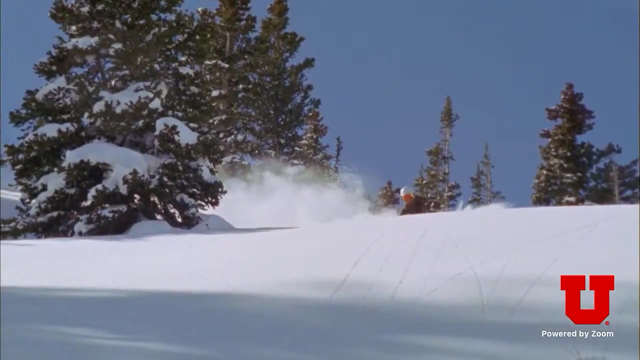 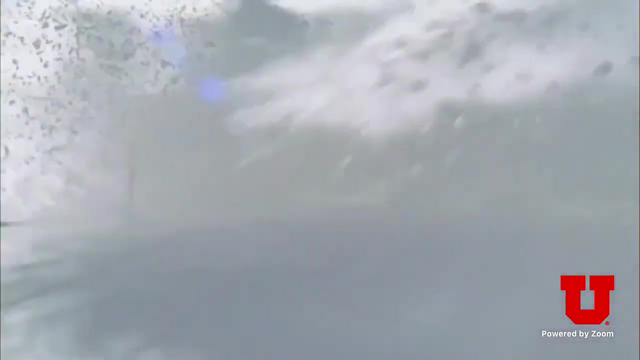 and even viruses and bacteria. It's truly otherworldly. I got interested in sea, ice and climate and questions like that from my love of skiing The first couple of times to Antarctica. I think people viewed me as this unusual mathematician. Let's bring him down there and see what he sees. 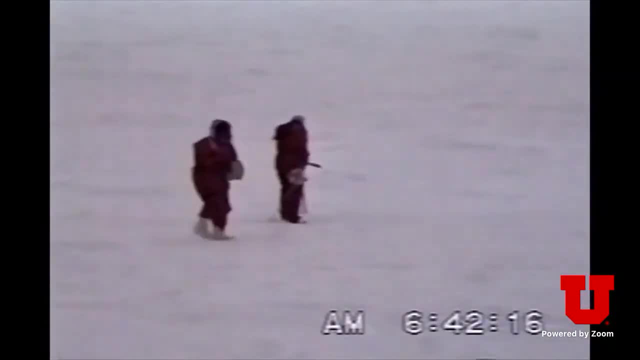 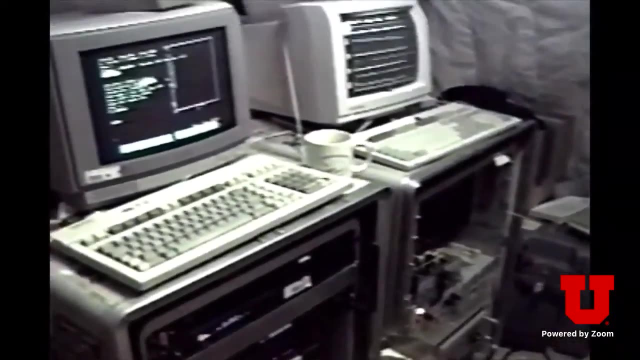 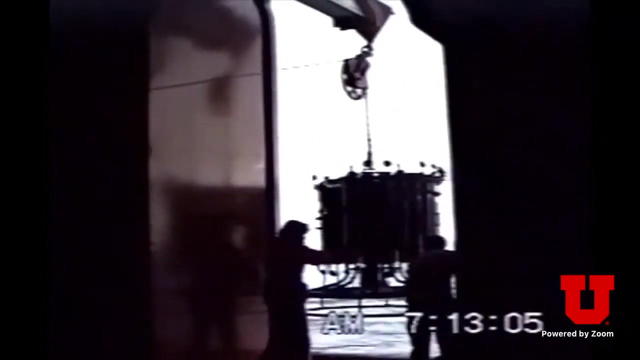 As I got further involved in this, I realized that I wanted to design my own experiments and my own equipment that would be testing my theories. I had to think this through in terms of okay, we're going down to Antarctica, We need to get certain experiments done. However, we must be mindful that well, 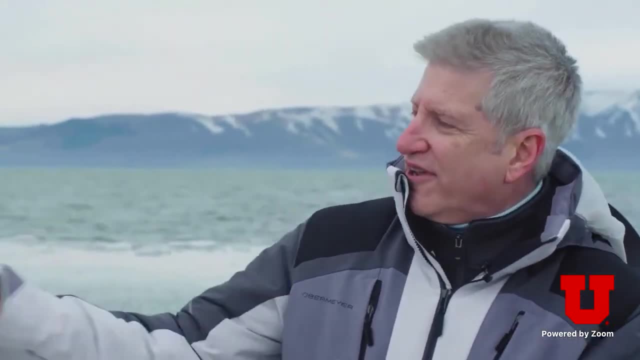 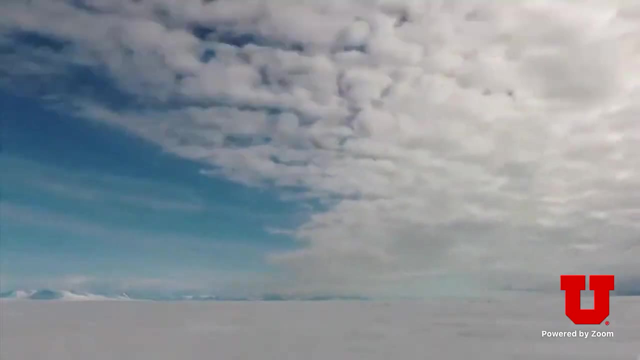 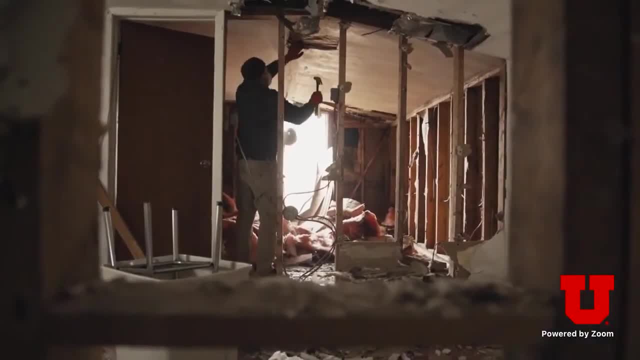 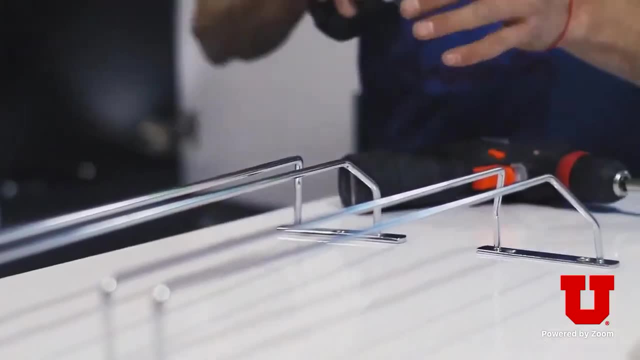 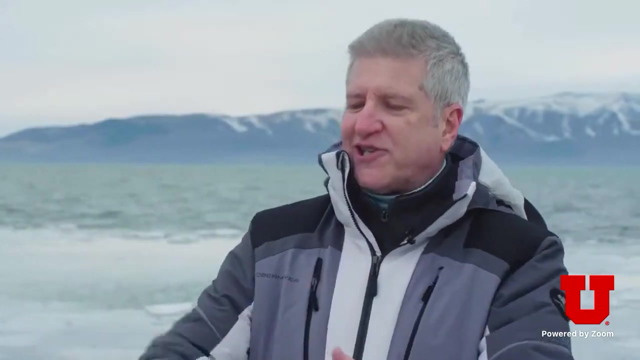 I had my condominium renovated. I had my condominium renovated And I started working with the contractor And I used this experience to develop the confidence that I would need to be able to work with my hands. think, on the fly, My first real expedition where I brought my own student. I had my own sled with my name on it. 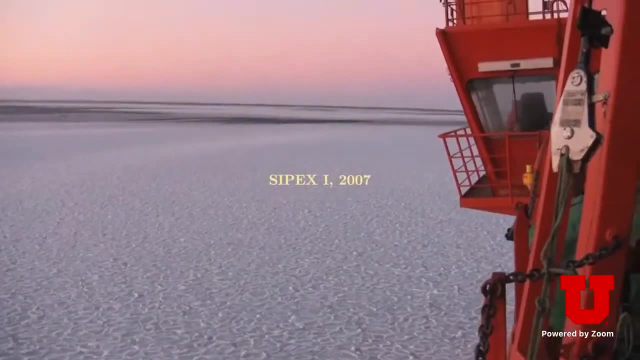 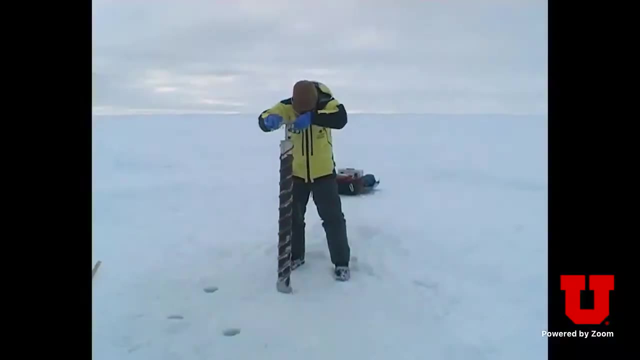 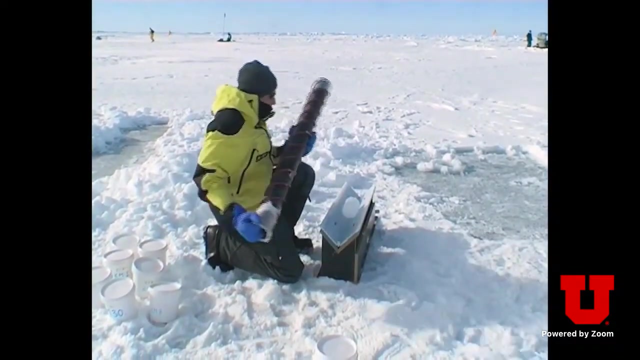 and started to have my own equipment was in 2007, on the SIPEX-1 expedition. I got into the mindset of really being able to prepare and what do you need to have to accomplish a somewhat complex experiment in such a remote and extreme environment? Two is one, one is none. 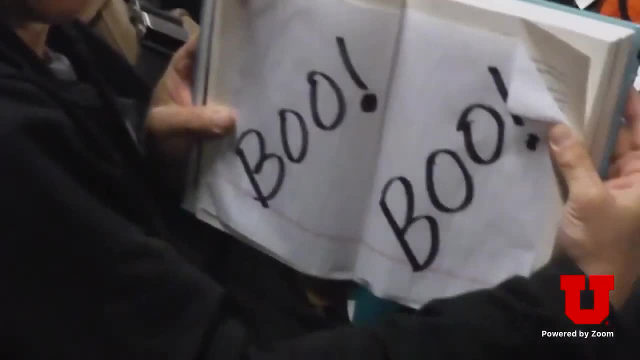 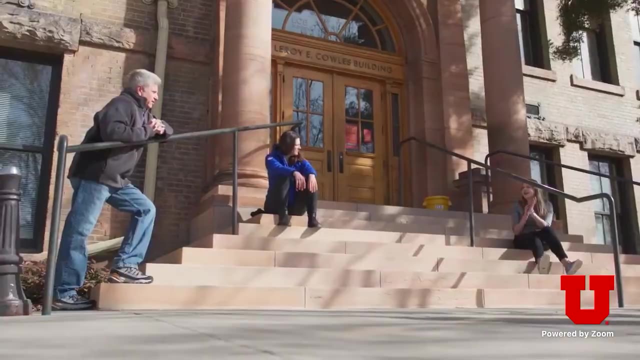 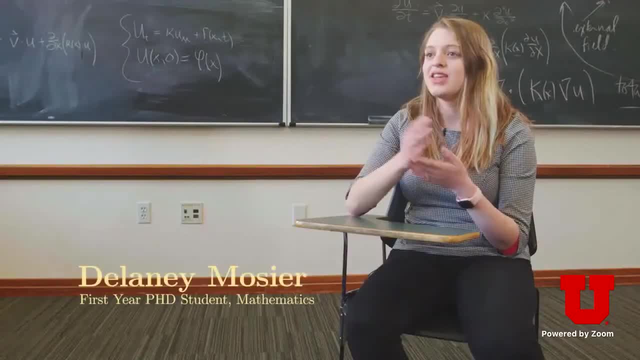 I've been a student for a long time. I've been a student for a long time. I've been a student for a long time. I love applying mathematics to sea ice. I think it's so neat that I can learn more about what's really going on in the world. 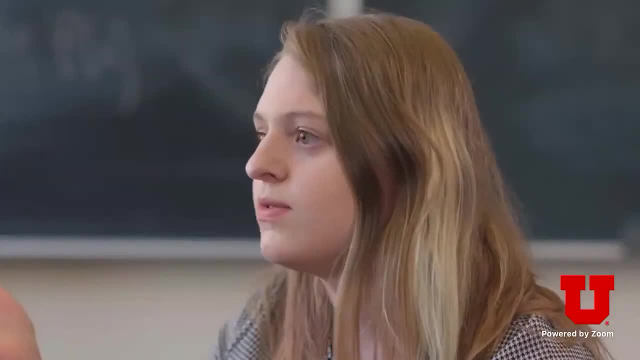 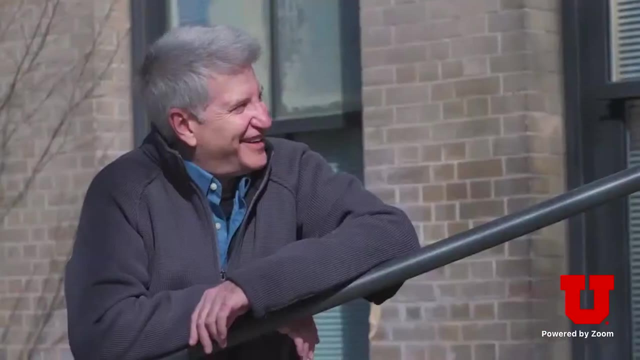 and potentially help attack one of the biggest problems facing modern society. with my math, There are two reasons I came here. The first was to work with Ken Coming to couple his understanding of the physics with my interest in the biology was the, I would say, the main appeal. 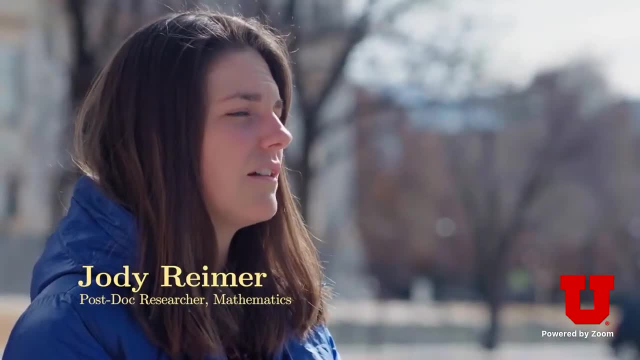 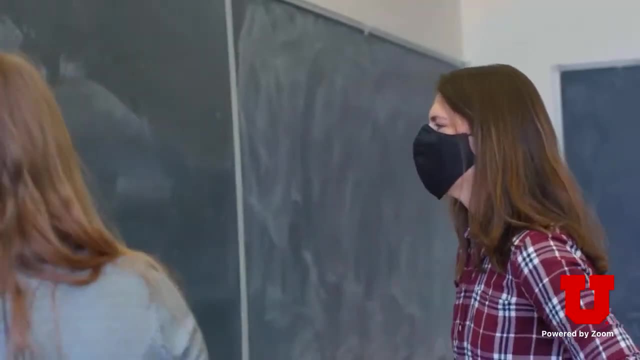 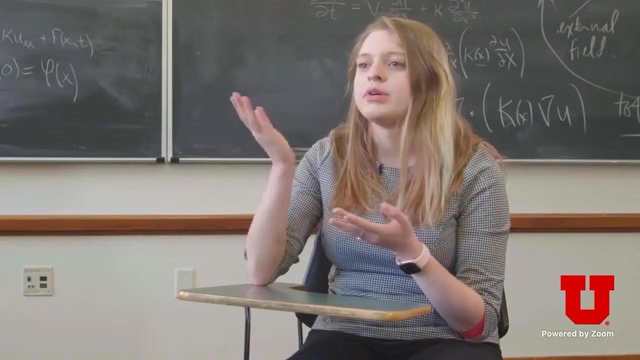 And the second reason is the strength of the math biology group here at this department. They have a vibrant mathematical biology community, and so I knew there'd be lots of exciting other stuff going on to get involved in. The level of math education and math research going on here is of a caliber 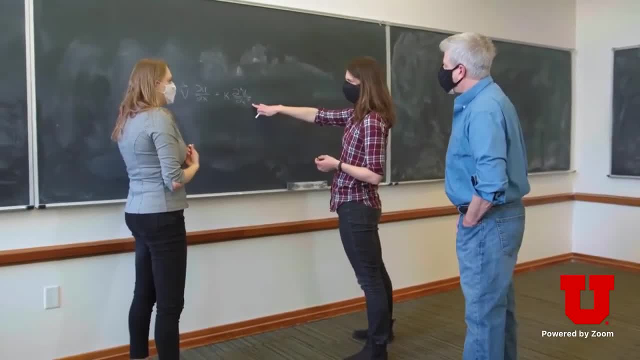 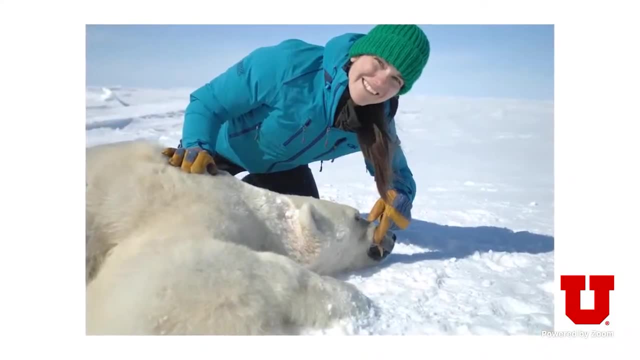 beyond anything I've seen at any other schools. I've had the opportunity to go to the Arctic, I think, six times. The value of that has been huge, I think, in developing my own research questions and coming into my own as an independent researcher as I transition. 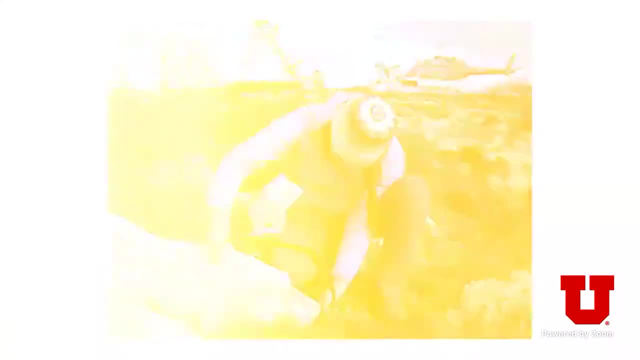 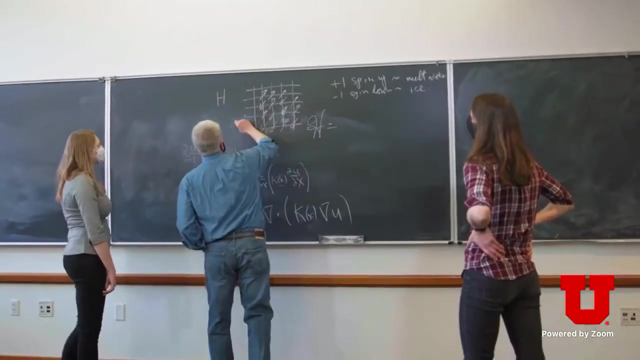 from grad school to postdoc and hopefully on to a research career. It's one thing to sort of sit in your office and develop theorems and theories and models about as complex a system as sea ice- If you actually go down there and see it for yourself. 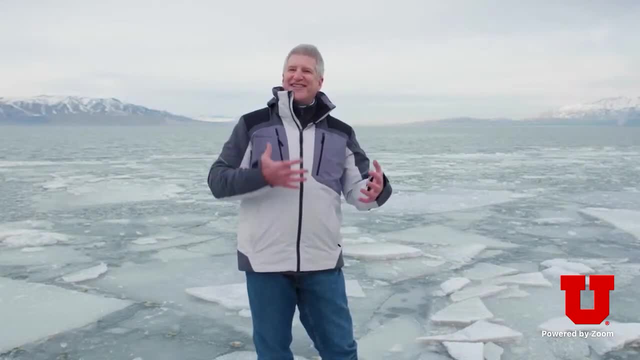 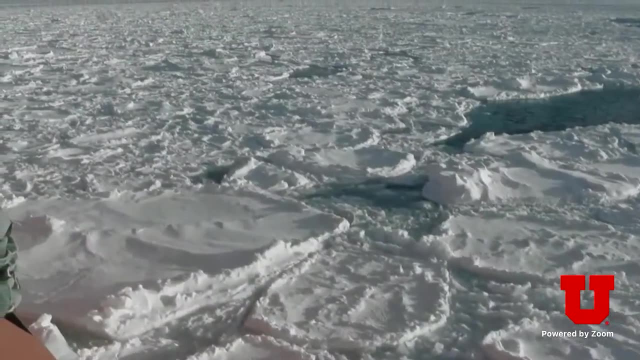 you understand that well. first of all, it's a lot more complicated than I thought. It exhibits all kinds of fascinating phenomena and behavior that you wouldn't necessarily expect or think is important until you actually get down there and see it in action. It is somewhat unusual. 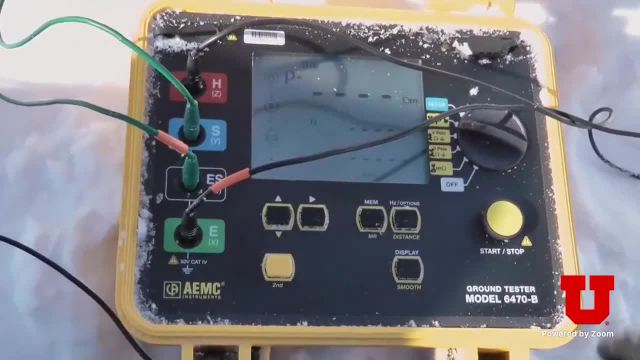 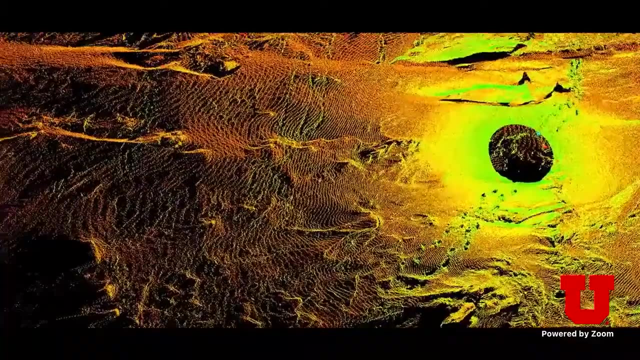 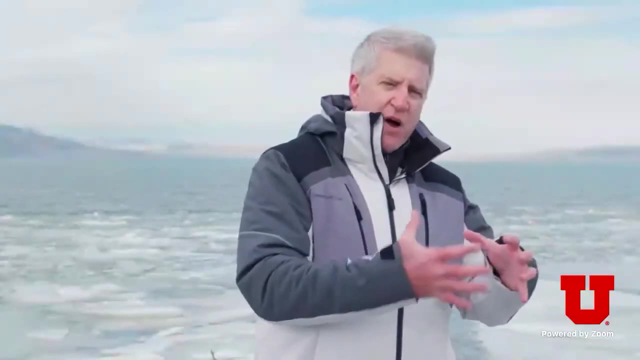 as a mathematician, to actually go down there and do experiments on sea ice. One of our main goals is to study sea ice and its role in the climate system. However, what we are doing in reality is to prove theorems and make models of the properties of sea ice. 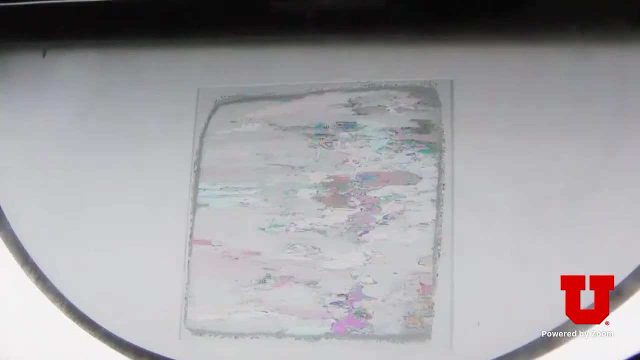 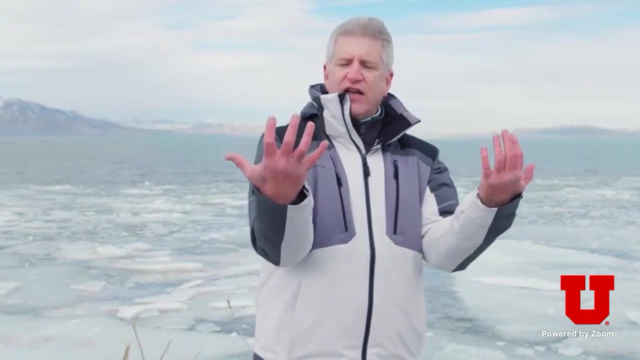 as a composite material. These results that we prove about sea ice have many other applications. If you put a picture of the brine microstructure of sea ice side by side with the microstructure microstructure of human bone, you see- wow, they look very similar to each other. 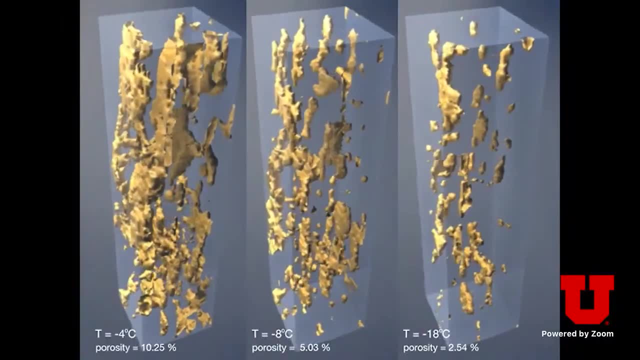 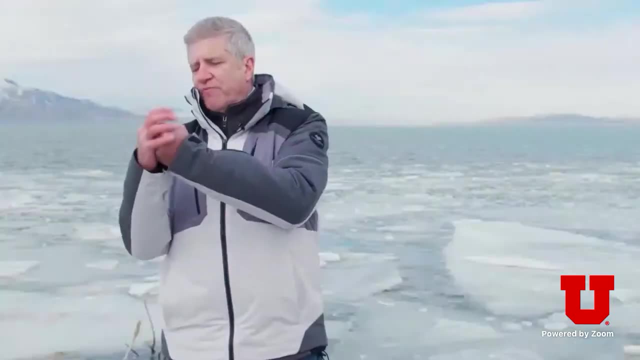 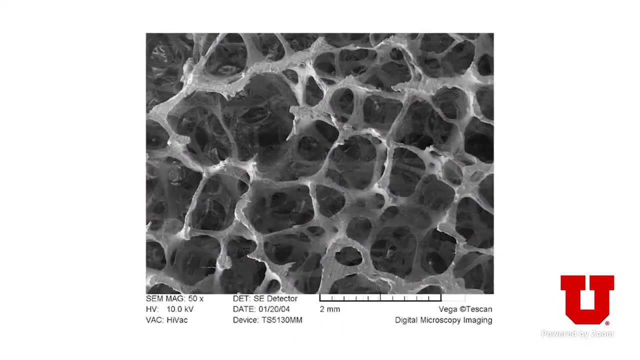 The mathematics that we developed to analyze the connectivity of the brine microstructure in sea ice, adapt that to analyzing the connectivity of the bone microstructure in humans and to develop a new method of monitoring the onset and progress of osteoporosis. It's the same mathematics. 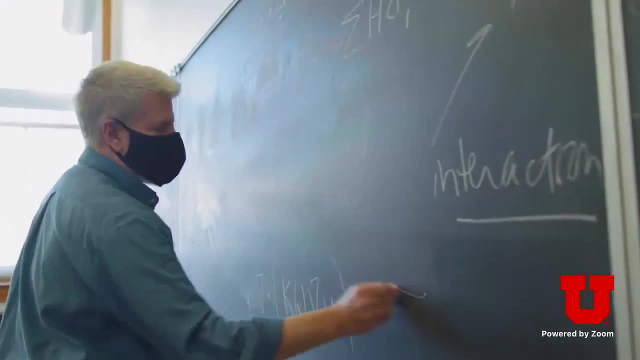 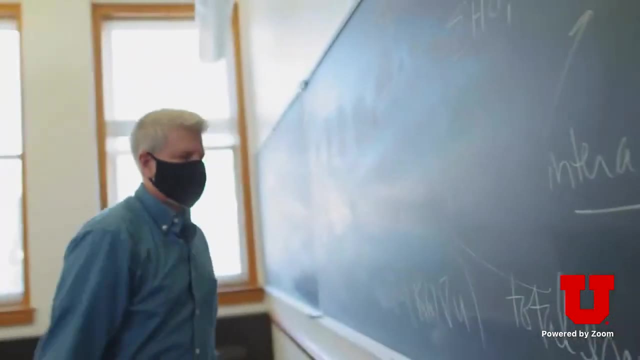 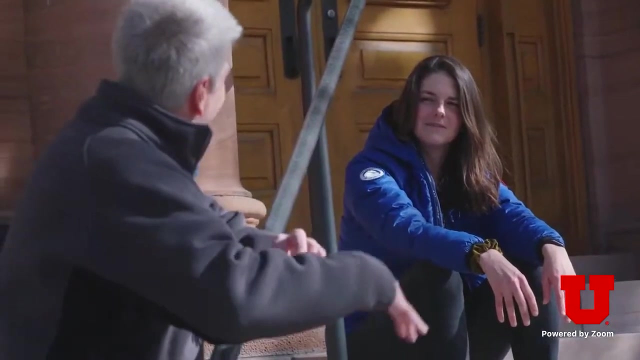 It's just amazing the degree to which mathematical models winds up helping you understand what's actually going on and to predict what the behavior is going to be in the future. Having the opportunity to turn young minds onto these kinds of fascinating, important ideas, where we're not just doing mathematics but also we're making an impact on some very important problems. 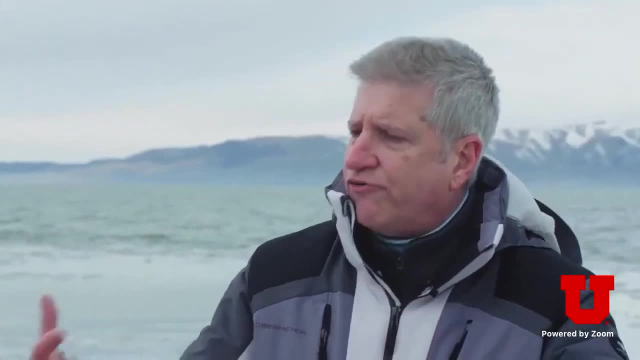 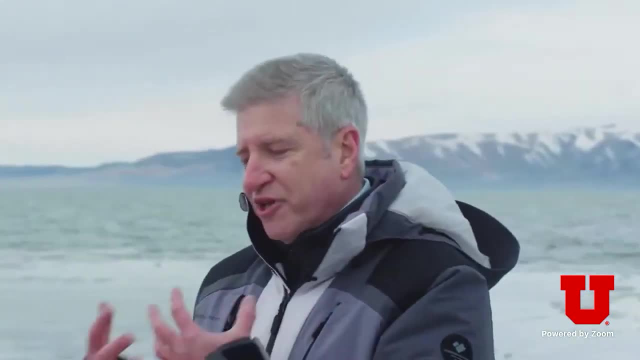 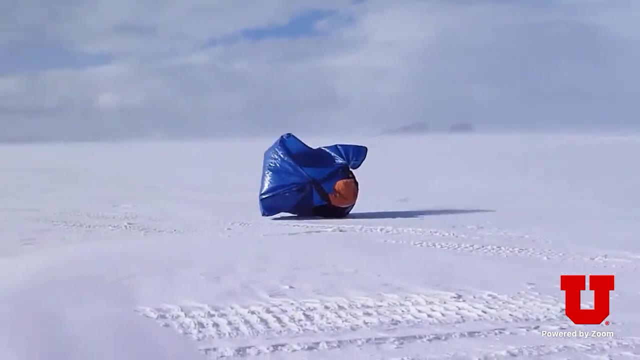 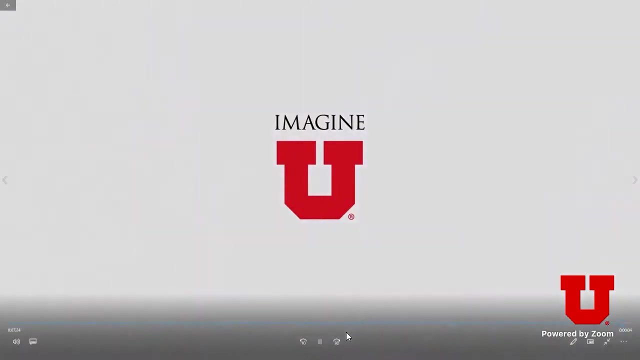 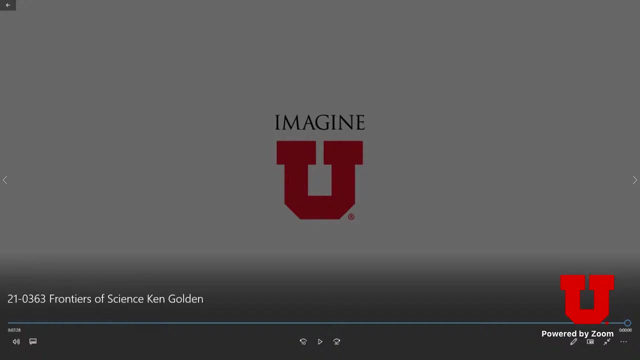 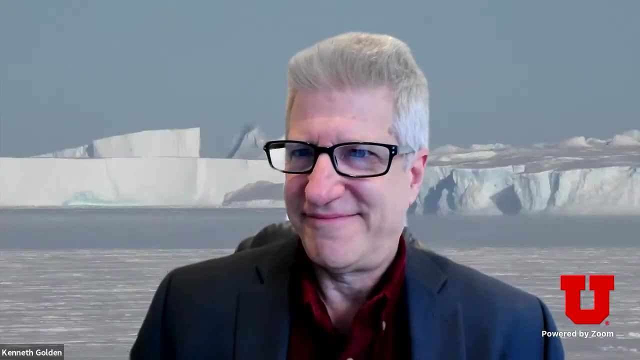 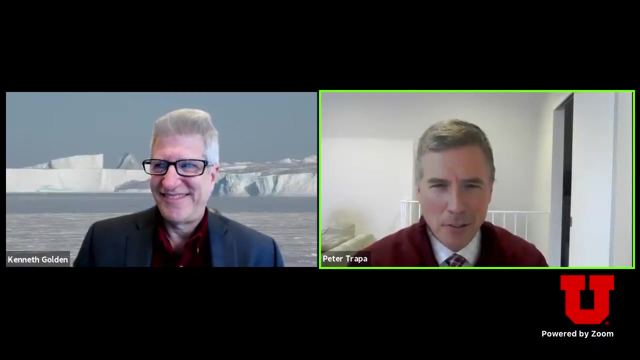 as well. you know, that's one of the main things I live for. So that was an inspiring video, And I think now I'm going to turn it over to Professor Golden, who's going to share his screen and talk through some slides. 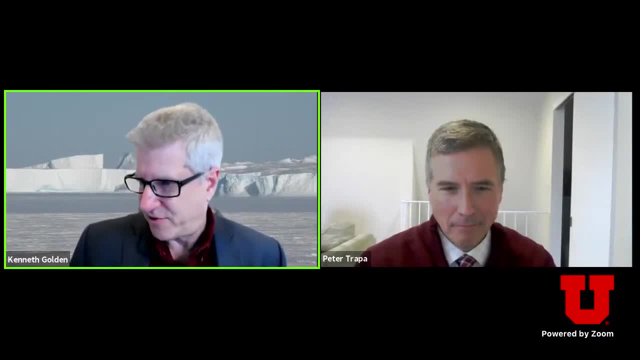 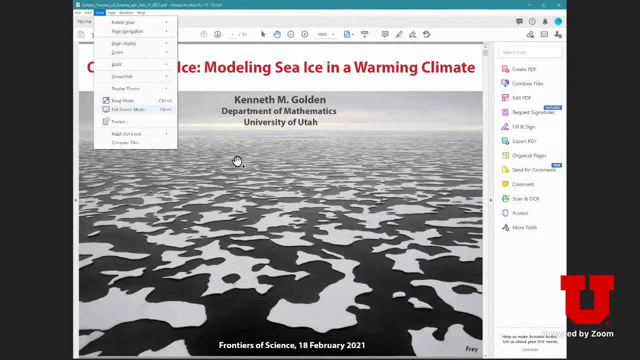 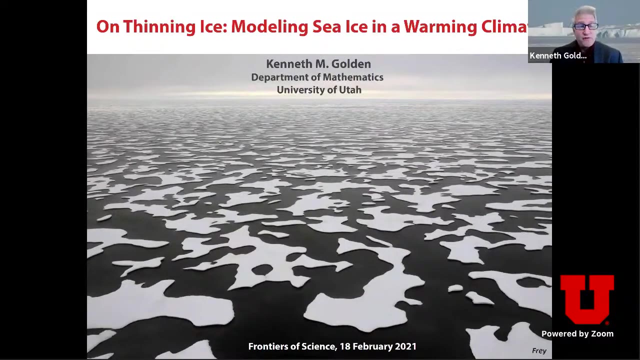 Great. Well, thank you very much, Peter. Let's see, let's here we go. Okay. well, thanks again, Peter. It's certainly a great pleasure and an honor to be here with all of you today and to be able to give. 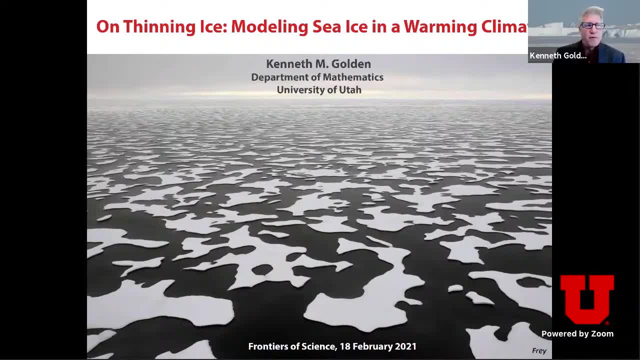 this Frontiers of Science lecture, And thank you all for coming today. So the evidence is clear: Our climate is changing, and it's changing perhaps most rapidly in the polar regions, And what I'm going to talk to you about today is how we're using mathematics to study one of the most important issues in our society. 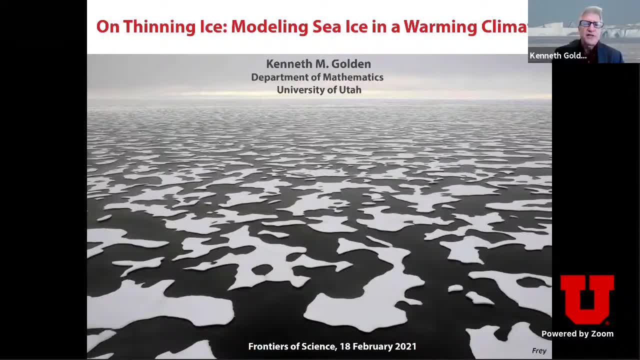 One of the critical components of our climate system, namely sea ice. And ultimately, we hope to use mathematics and theoretical physics to advance how sea ice is represented in climate models and improve projections of climate change, the fate of Earth's ice packs, as well as the ecosystems the sea ice supports. 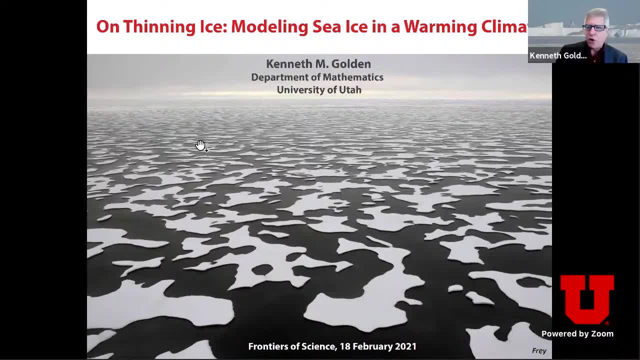 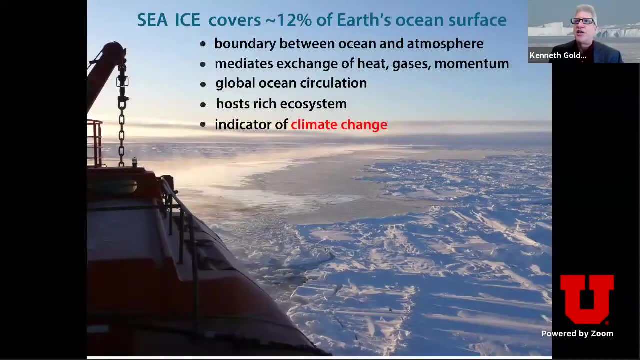 Now, already in this opening slide, this is melting Arctic sea ice. So hopefully already here you can see not just the beauty But some of the underlying geometrical richness and mathematics in such structures that we're going to be studying. So why study sea ice? 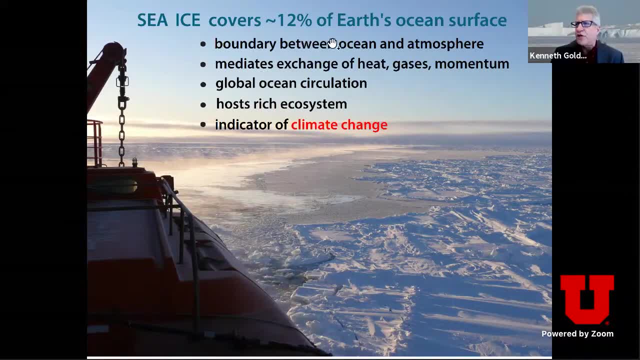 Well, it's melting, but there's still a lot of it. It covers roughly 12% of Earth's ocean surface. It forms the very thin frozen boundary layer between the two principal geophysical fluids on the Earth and with the ocean and the atmosphere. 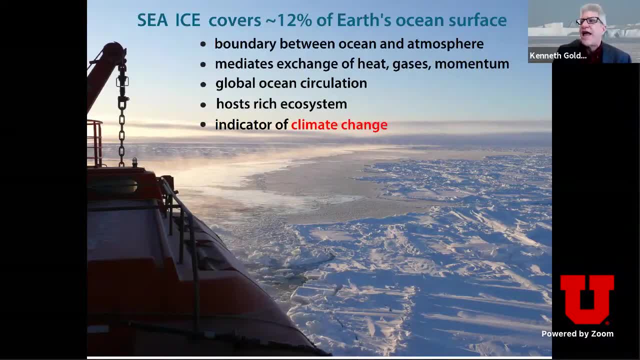 And, as such, it mediates the exchange of heat gases and momentary gases, And momentum between them. Both the melting and the freezing of sea ice play a very important role in global ocean circulation, And it's one of the principal pathways by which the polar regions communicate with the rest of the world ocean system, as well as the global climate system. 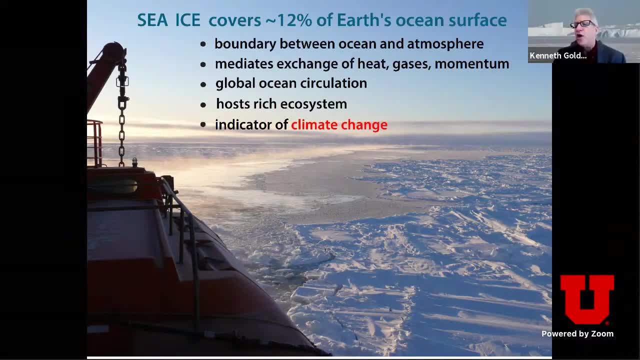 And, as you'll see, sea ice hosts a very rich and robust ecosystem from the top predators like the leopard, seals and polar bears, and so on, All the way up to the ocean. And, as you'll see, sea ice hosts a very rich and robust ecosystem from the top predators like the leopard, seals and polar bears, and so on. 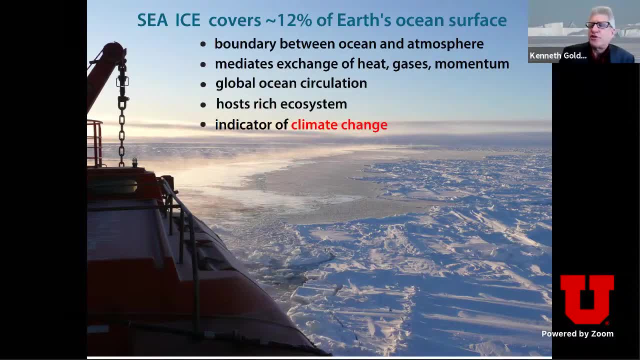 All the way up to the ocean And, as you'll see, sea ice hosts a very rich and robust ecosystem from the top predators like the leopard, seals and polar bears, and so on. All the way up to the ocean And, as you'll see, sea ice hosts a very rich and robust ecosystem from the top predators like the leopard, seals and polar bears, and so on. 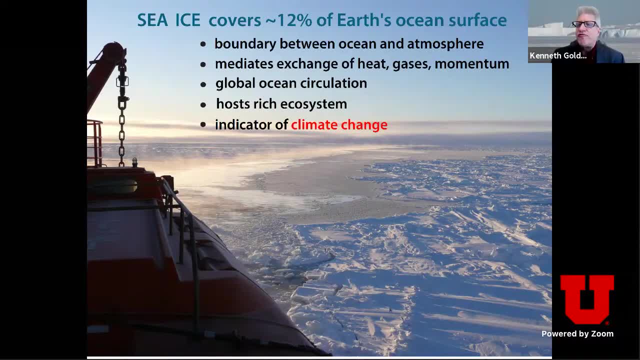 All the way up to the ocean And, as you'll see, sea ice hosts a very rich and robust ecosystem from the top predators like the leopard, seals and polar bears, and so on. All the way up to the ocean And, as you'll see, sea ice hosts a very rich and robust ecosystem from the top predators like the leopard, seals and polar bears, and so on. 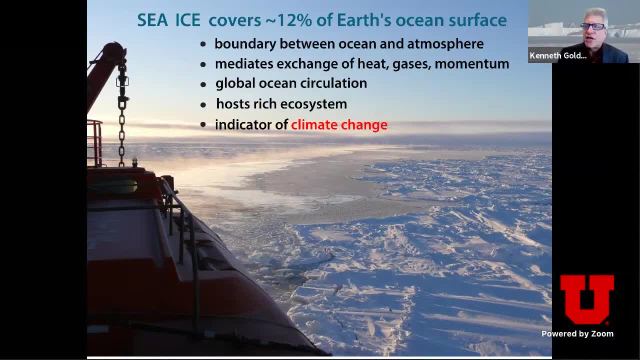 All the way up to the ocean And, as you'll see, sea ice hosts a very rich and robust ecosystem from the top predators like the leopard, seals and polar bears, and so on. All the way up to the ocean And, as you'll see, sea ice hosts a very rich and robust ecosystem from the top predators like the leopard, seals and polar bears, and so on. 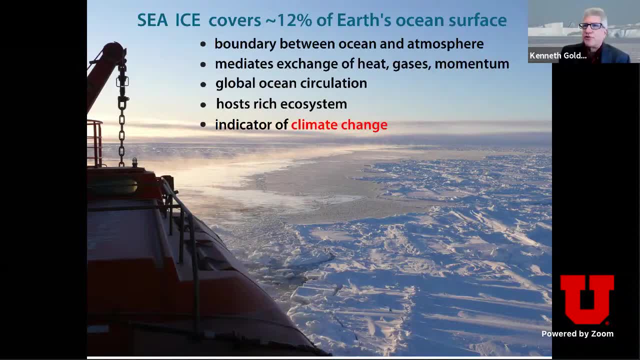 All the way up to the ocean And, as you'll see, sea ice hosts a very rich and robust ecosystem from the top predators like the leopard, seals and polar bears, and so on. All the way up to the ocean And, as you'll see, sea ice hosts a very rich and robust ecosystem from the top predators like the leopard, seals and polar bears, and so on. 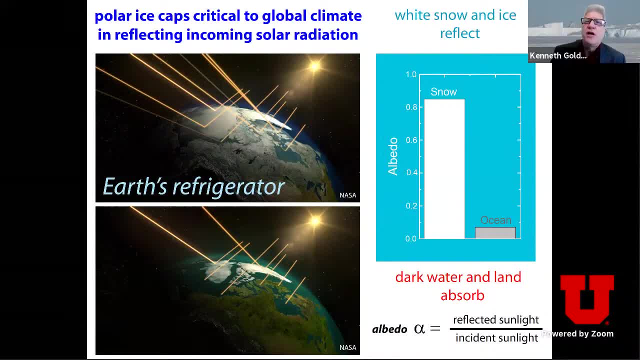 All the way up to the ocean And, as you'll see, sea ice hosts a very rich and robust ecosystem from the top predators like the leopard, seals and polar bears, and so on. All the way up to the ocean And, as you'll see, sea ice hosts a very rich and robust ecosystem from the top predators like the leopard, seals and polar bears, and so on. 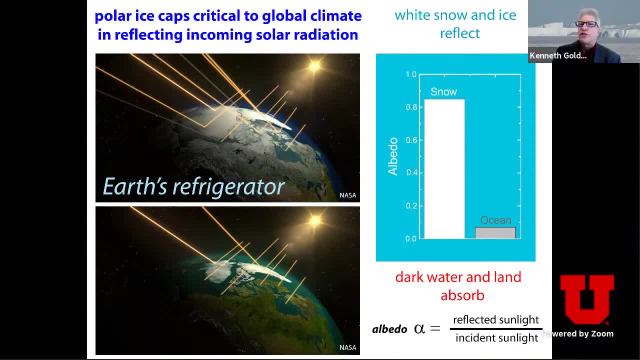 All the way up to the ocean And, as you'll see, sea ice hosts a very rich and robust ecosystem from the top predators like the leopard, seals and polar bears, and so on. All the way up to the ocean And, as you'll see, sea ice hosts a very rich and robust ecosystem from the top predators like the leopard, seals and polar bears, and so on. 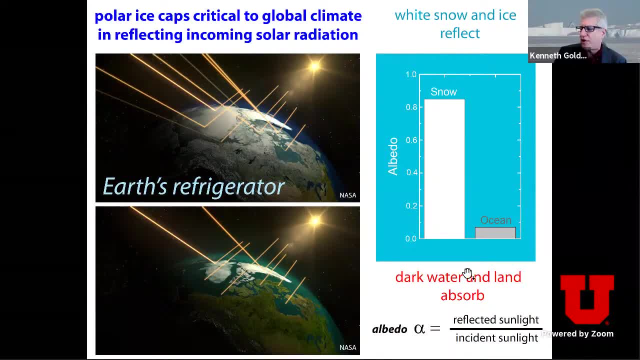 All the way up to the ocean And, as you'll see, sea ice hosts a very rich and robust ecosystem from the top predators like the leopard, seals and polar bears, and so on. All the way up to the ocean And, as you'll see, sea ice hosts a very rich and robust ecosystem from the top predators like the leopard, seals and polar bears, and so on. 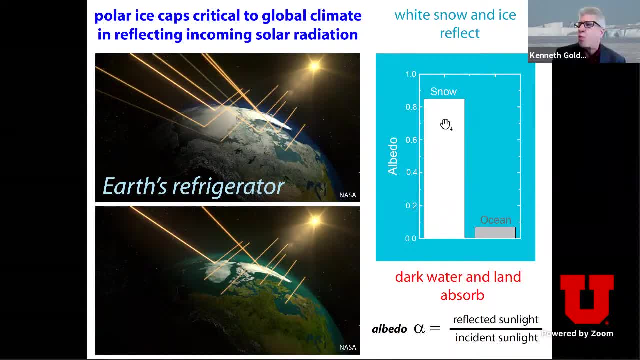 All the way up to the ocean And, as you'll see, sea ice hosts a very rich and robust ecosystem from the top predators like the leopard, seals and polar bears, and so on. All the way up to the ocean And, as you'll see, sea ice hosts a very rich and robust ecosystem from the top predators like the leopard, seals and polar bears, and so on. 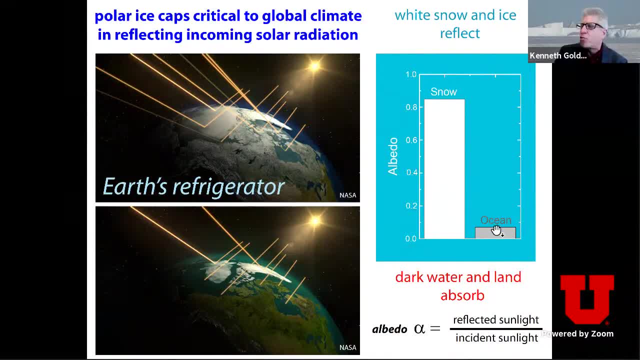 All the way up to the ocean And, as you'll see, sea ice hosts a very rich and robust ecosystem from the top predators like the leopard, seals and polar bears, and so on. All the way up to the ocean And, as you'll see, sea ice hosts a very rich and robust ecosystem from the top predators like the leopard, seals and polar bears, and so on. 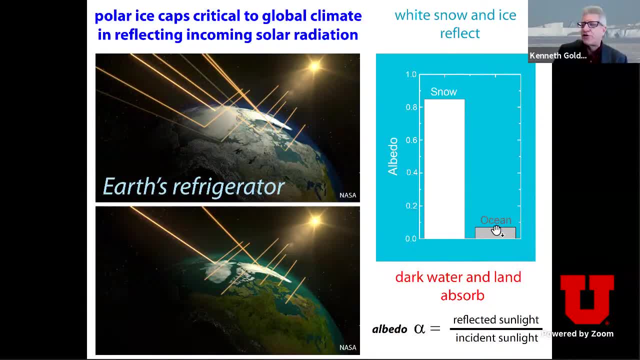 All the way up to the ocean And, as you'll see, sea ice hosts a very rich and robust ecosystem from the top predators like the leopard, seals and polar bears, and so on. All the way up to the ocean And, as you'll see, sea ice hosts a very rich and robust ecosystem from the top predators like the leopard, seals and polar bears, and so on. 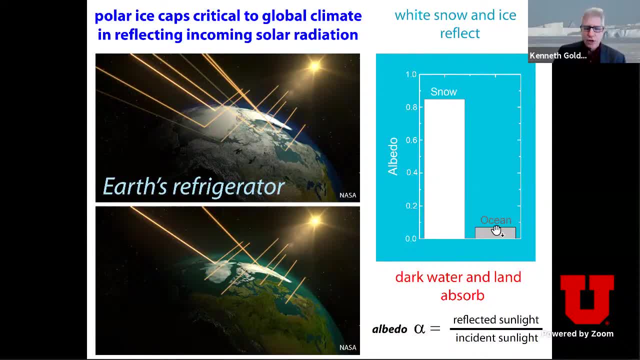 All the way up to the ocean And, as you'll see, sea ice hosts a very rich and robust ecosystem from the top predators like the leopard, seals and polar bears, and so on. All the way up to the ocean And, as you'll see, sea ice hosts a very rich and robust ecosystem from the top predators like the leopard, seals and polar bears, and so on. 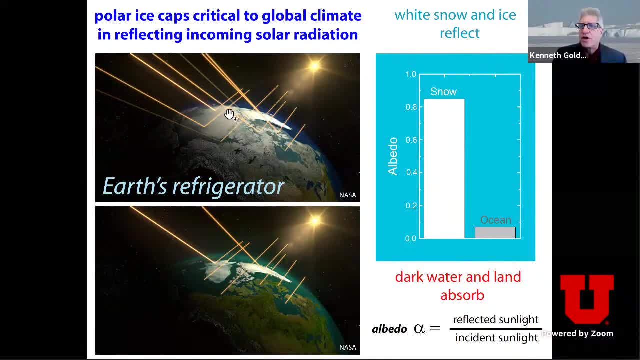 All the way up to the ocean And, as you'll see, sea ice hosts a very rich and robust ecosystem from the top predators like the leopard, seals and polar bears, and so on. All the way up to the ocean And, as you'll see, sea ice hosts a very rich and robust ecosystem from the top predators like the leopard, seals and polar bears, and so on. 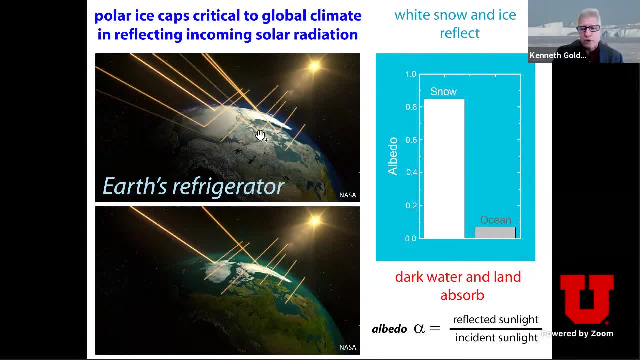 All the way up to the ocean And, as you'll see, sea ice hosts a very rich and robust ecosystem from the top predators like the leopard, seals and polar bears, and so on. All the way up to the ocean And, as you'll see, sea ice hosts a very rich and robust ecosystem from the top predators like the leopard, seals and polar bears, and so on. 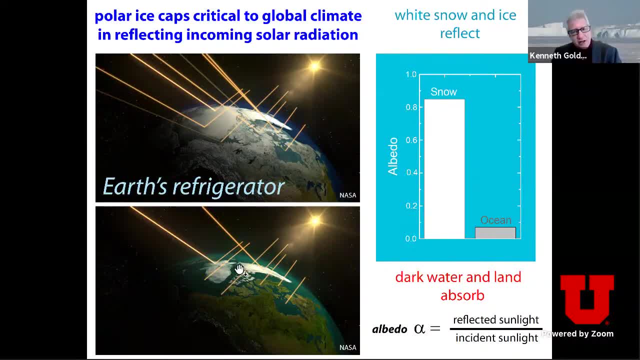 All the way up to the ocean And, as you'll see, sea ice hosts a very rich and robust ecosystem from the top predators like the leopard, seals and polar bears, and so on. All the way up to the ocean And, as you'll see, sea ice hosts a very rich and robust ecosystem from the top predators like the leopard, seals and polar bears, and so on. 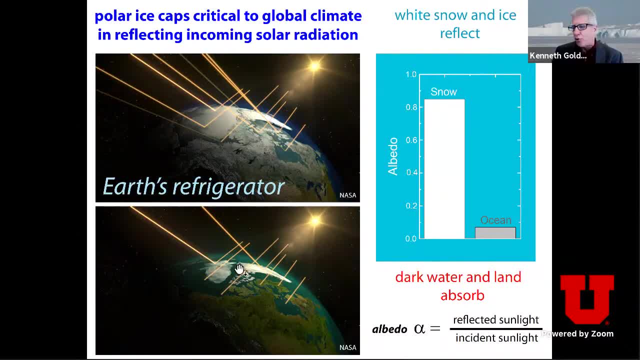 All the way up to the ocean And, as you'll see, sea ice hosts a very rich and robust ecosystem from the top predators like the leopard, seals and polar bears, and so on. All the way up to the ocean And, as you'll see, sea ice hosts a very rich and robust ecosystem from the top predators like the leopard, seals and polar bears, and so on. 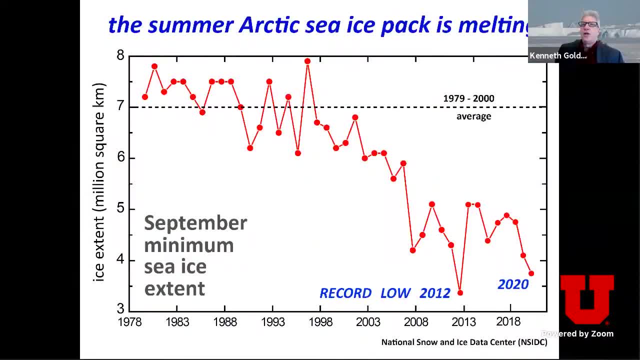 All the way up to the ocean And, as you'll see, sea ice hosts a very rich and robust ecosystem from the top predators like the leopard, seals and polar bears, and so on. All the way up to the ocean And, as you'll see, sea ice hosts a very rich and robust ecosystem from the top predators like the leopard, seals and polar bears, and so on. 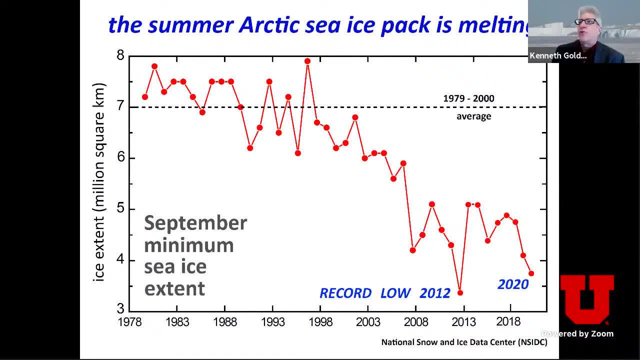 All the way up to the ocean And, as you'll see, sea ice hosts a very rich and robust ecosystem from the top predators like the leopard, seals and polar bears, and so on. All the way up to the ocean And, as you'll see, sea ice hosts a very rich and robust ecosystem from the top predators like the leopard, seals and polar bears, and so on. 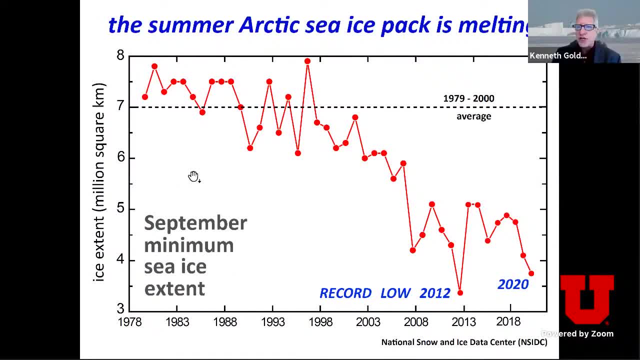 All the way up to the ocean And, as you'll see, sea ice hosts a very rich and robust ecosystem from the top predators like the leopard, seals and polar bears, and so on. All the way up to the ocean And, as you'll see, sea ice hosts a very rich and robust ecosystem from the top predators like the leopard, seals and polar bears, and so on. 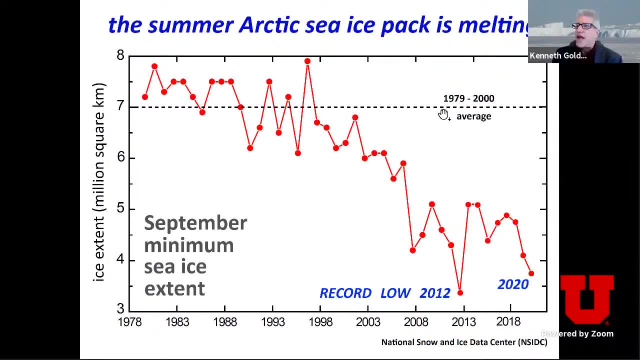 All the way up to the ocean And, as you'll see, sea ice hosts a very rich and robust ecosystem from the top predators like the leopard, seals and polar bears, and so on. All the way up to the ocean And, as you'll see, sea ice hosts a very rich and robust ecosystem from the top predators like the leopard, seals and polar bears, and so on. 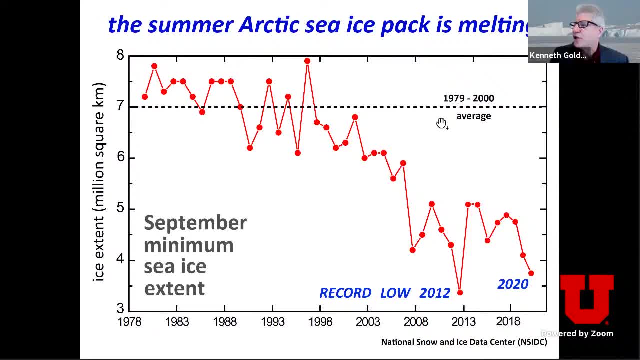 All the way up to the ocean And, as you'll see, sea ice hosts a very rich and robust ecosystem from the top predators like the leopard, seals and polar bears, and so on. All the way up to the ocean And, as you'll see, sea ice hosts a very rich and robust ecosystem from the top predators like the leopard, seals and polar bears, and so on. 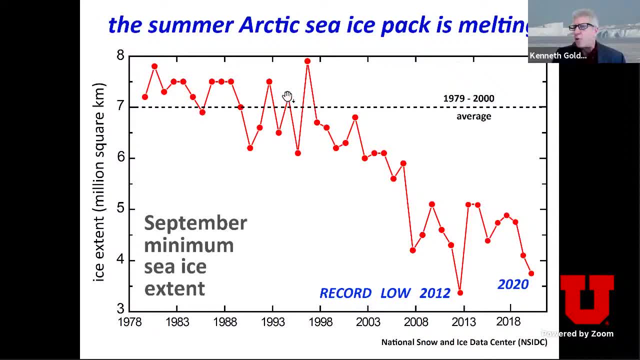 All the way up to the ocean And, as you'll see, sea ice hosts a very rich and robust ecosystem from the top predators like the leopard, seals and polar bears, and so on. All the way up to the ocean And, as you'll see, sea ice hosts a very rich and robust ecosystem from the top predators like the leopard, seals and polar bears, and so on. 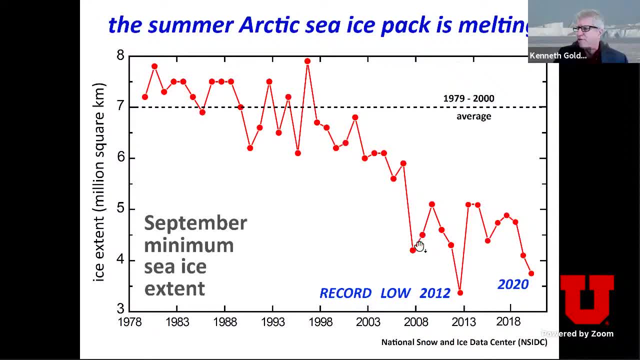 All the way up to the ocean And, as you'll see, sea ice hosts a very rich and robust ecosystem from the top predators like the leopard, seals and polar bears, and so on. All the way up to the ocean And, as you'll see, sea ice hosts a very rich and robust ecosystem from the top predators like the leopard, seals and polar bears, and so on. 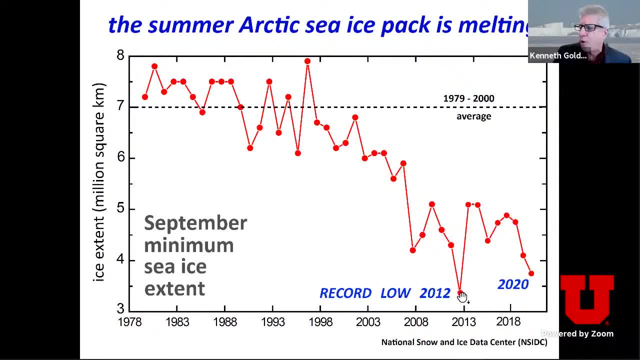 All the way up to the ocean And, as you'll see, sea ice hosts a very rich and robust ecosystem from the top predators like the leopard, seals and polar bears, and so on. All the way up to the ocean And, as you'll see, sea ice hosts a very rich and robust ecosystem from the top predators like the leopard, seals and polar bears, and so on. 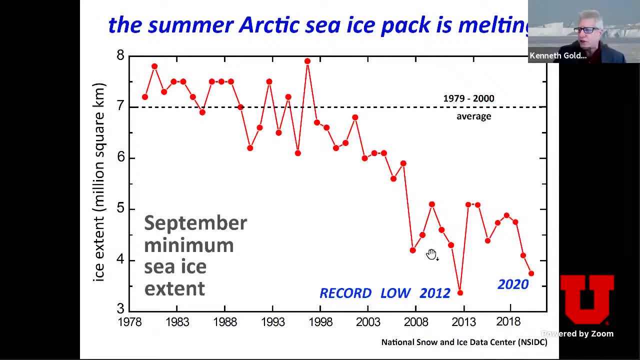 All the way up to the ocean And, as you'll see, sea ice hosts a very rich and robust ecosystem from the top predators like the leopard, seals and polar bears, and so on. All the way up to the ocean And, as you'll see, sea ice hosts a very rich and robust ecosystem from the top predators like the leopard, seals and polar bears, and so on. 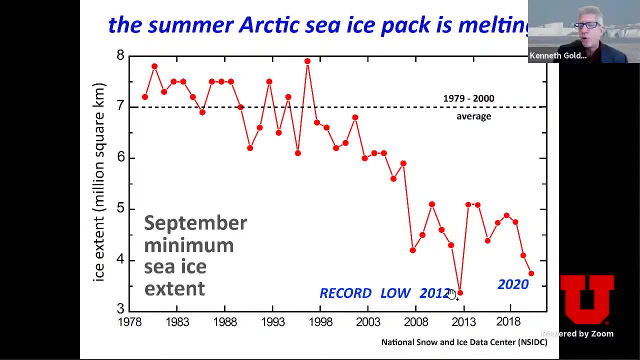 All the way up to the ocean And, as you'll see, sea ice hosts a very rich and robust ecosystem from the top predators like the leopard, seals and polar bears, and so on. All the way up to the ocean And, as you'll see, sea ice hosts a very rich and robust ecosystem from the top predators like the leopard, seals and polar bears, and so on. 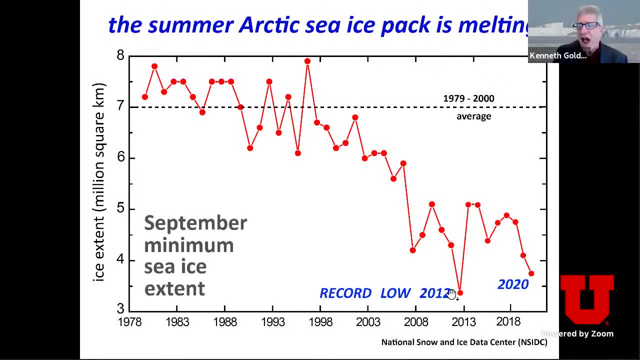 All the way up to the ocean And, as you'll see, sea ice hosts a very rich and robust ecosystem from the top predators like the leopard, seals and polar bears, and so on. All the way up to the ocean And, as you'll see, sea ice hosts a very rich and robust ecosystem from the top predators like the leopard, seals and polar bears, and so on. 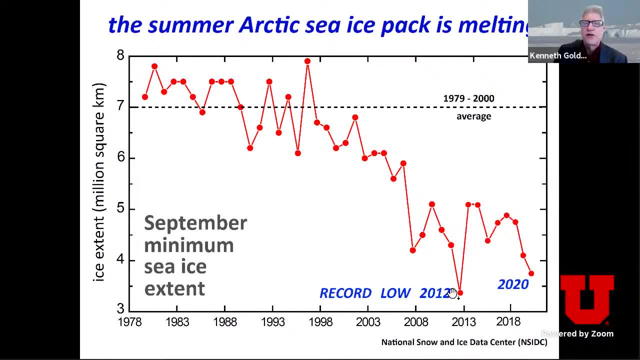 All the way up to the ocean And, as you'll see, sea ice hosts a very rich and robust ecosystem from the top predators like the leopard, seals and polar bears, and so on. All the way up to the ocean And, as you'll see, sea ice hosts a very rich and robust ecosystem from the top predators like the leopard, seals and polar bears, and so on. 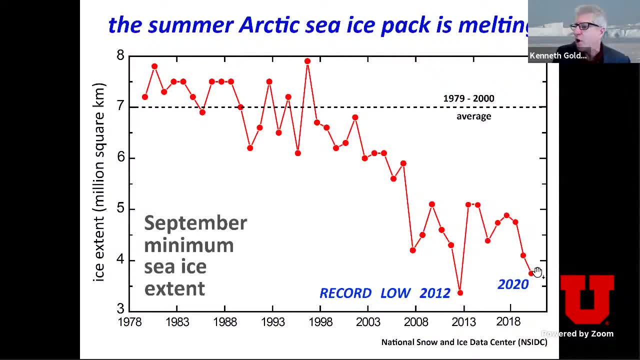 All the way up to the ocean And, as you'll see, sea ice hosts a very rich and robust ecosystem from the top predators like the leopard, seals and polar bears, and so on. All the way up to the ocean And, as you'll see, sea ice hosts a very rich and robust ecosystem from the top predators like the leopard, seals and polar bears, and so on. 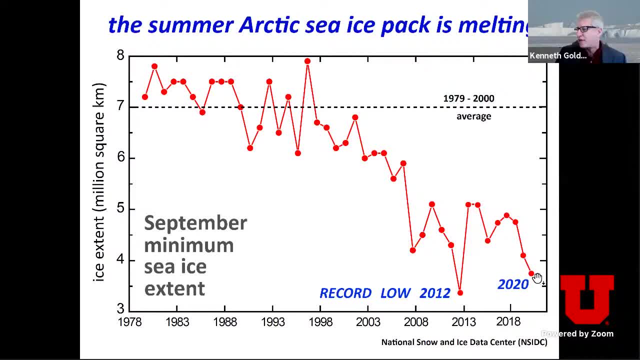 All the way up to the ocean And, as you'll see, sea ice hosts a very rich and robust ecosystem from the top predators like the leopard, seals and polar bears, and so on. All the way up to the ocean And, as you'll see, sea ice hosts a very rich and robust ecosystem from the top predators like the leopard, seals and polar bears, and so on. 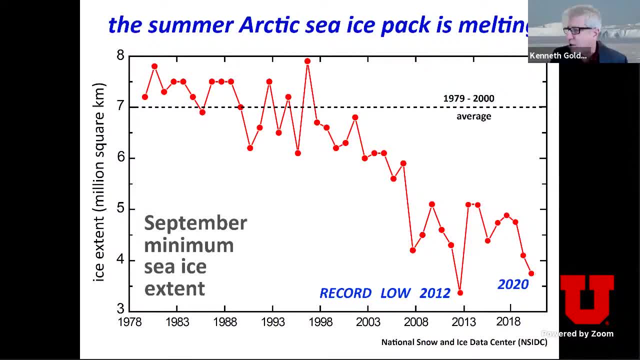 All the way up to the ocean And, as you'll see, sea ice hosts a very rich and robust ecosystem from the top predators like the leopard, seals and polar bears, and so on. All the way up to the ocean And, as you'll see, sea ice hosts a very rich and robust ecosystem from the top predators like the leopard, seals and polar bears, and so on. 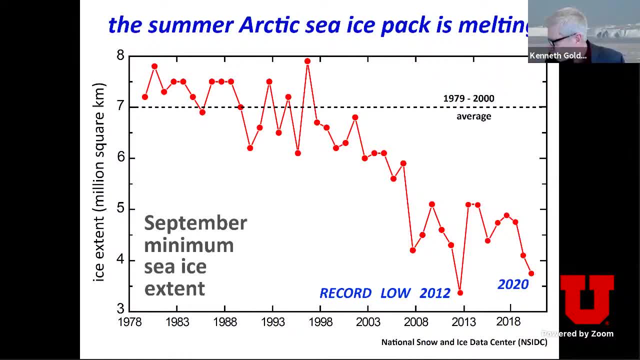 All the way up to the ocean And, as you'll see, sea ice hosts a very rich and robust ecosystem from the top predators like the leopard, seals and polar bears, and so on. All the way up to the ocean And, as you'll see, sea ice hosts a very rich and robust ecosystem from the top predators like the leopard, seals and polar bears, and so on. 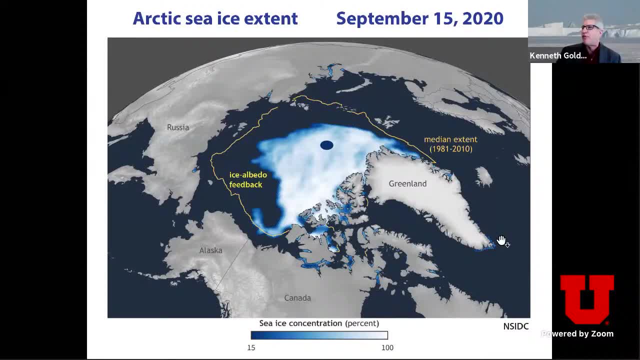 All the way up to the ocean And, as you'll see, sea ice hosts a very rich and robust ecosystem from the top predators like the leopard, seals and polar bears, and so on. All the way up to the ocean And, as you'll see, sea ice hosts a very rich and robust ecosystem from the top predators like the leopard, seals and polar bears, and so on. 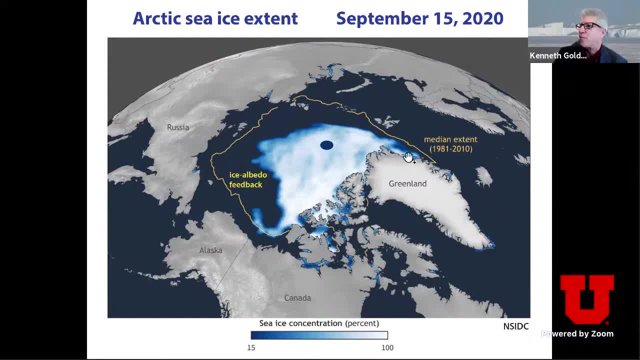 All the way up to the ocean And, as you'll see, sea ice hosts a very rich and robust ecosystem from the top predators like the leopard, seals and polar bears, and so on. All the way up to the ocean And, as you'll see, sea ice hosts a very rich and robust ecosystem from the top predators like the leopard, seals and polar bears, and so on. 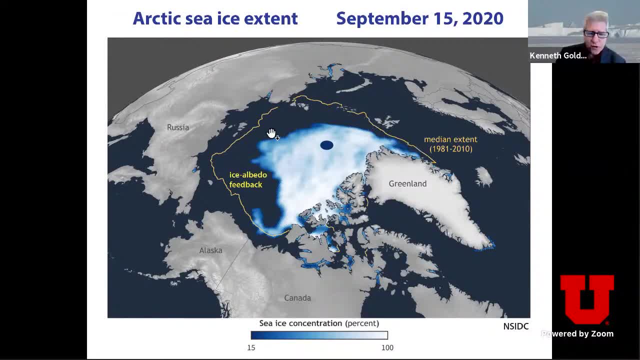 All the way up to the ocean And, as you'll see, sea ice hosts a very rich and robust ecosystem from the top predators like the leopard, seals and polar bears, and so on. All the way up to the ocean And, as you'll see, sea ice hosts a very rich and robust ecosystem from the top predators like the leopard, seals and polar bears, and so on. 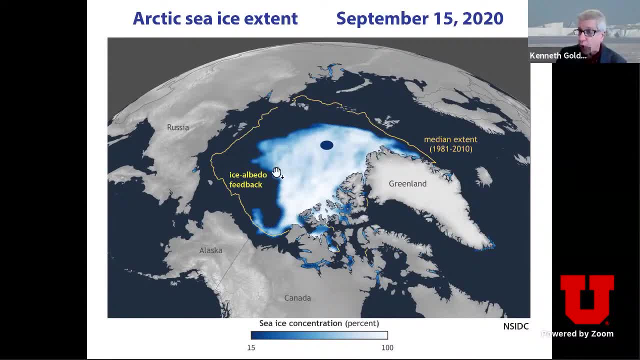 All the way up to the ocean And, as you'll see, sea ice hosts a very rich and robust ecosystem from the top predators like the leopard, seals and polar bears, and so on. All the way up to the ocean And, as you'll see, sea ice hosts a very rich and robust ecosystem from the top predators like the leopard, seals and polar bears, and so on. 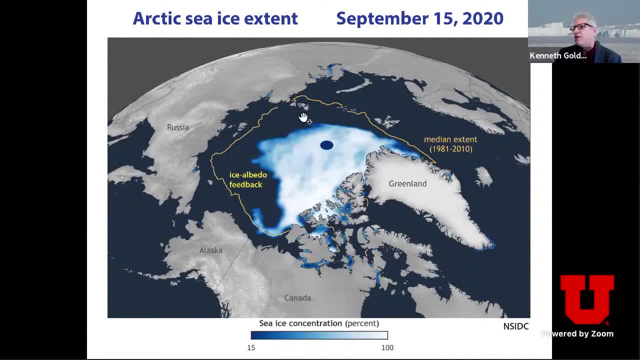 All the way up to the ocean And, as you'll see, sea ice hosts a very rich and robust ecosystem from the top predators like the leopard, seals and polar bears, and so on. All the way up to the ocean And, as you'll see, sea ice hosts a very rich and robust ecosystem from the top predators like the leopard, seals and polar bears, and so on. 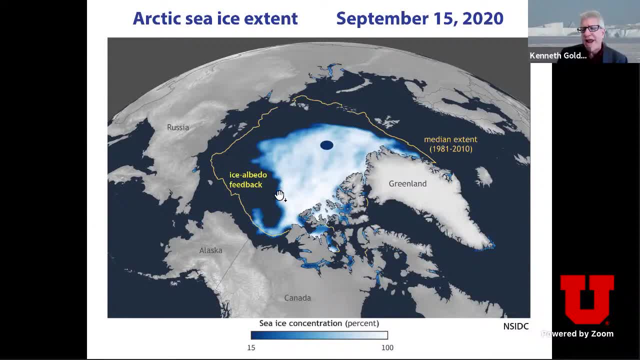 All the way up to the ocean And, as you'll see, sea ice hosts a very rich and robust ecosystem from the top predators like the leopard, seals and polar bears, and so on. All the way up to the ocean And, as you'll see, sea ice hosts a very rich and robust ecosystem from the top predators like the leopard, seals and polar bears, and so on. 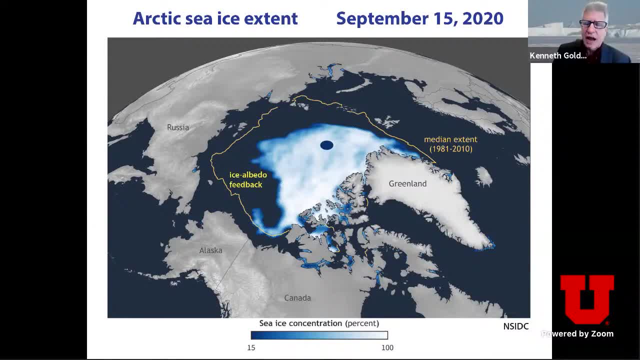 All the way up to the ocean And, as you'll see, sea ice hosts a very rich and robust ecosystem from the top predators like the leopard, seals and polar bears, and so on. All the way up to the ocean And, as you'll see, sea ice hosts a very rich and robust ecosystem from the top predators like the leopard, seals and polar bears, and so on. 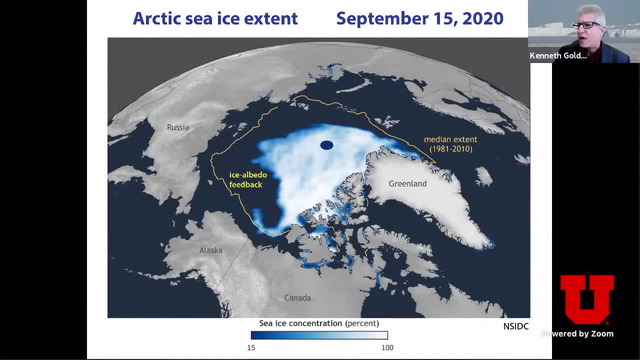 All the way up to the ocean And, as you'll see, sea ice hosts a very rich and robust ecosystem from the top predators like the leopard, seals and polar bears, and so on. All the way up to the ocean And, as you'll see, sea ice hosts a very rich and robust ecosystem from the top predators like the leopard, seals and polar bears, and so on. 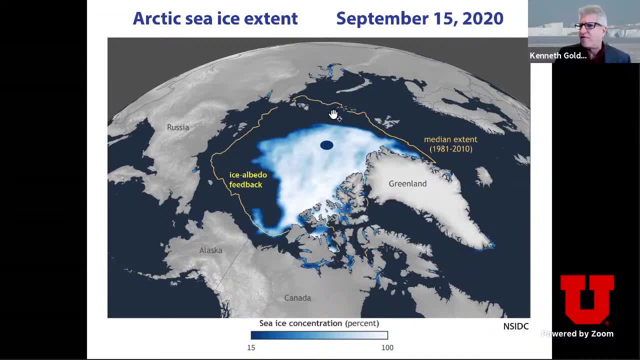 All the way up to the ocean And, as you'll see, sea ice hosts a very rich and robust ecosystem from the top predators like the leopard, seals and polar bears, and so on. All the way up to the ocean And, as you'll see, sea ice hosts a very rich and robust ecosystem from the top predators like the leopard, seals and polar bears, and so on. 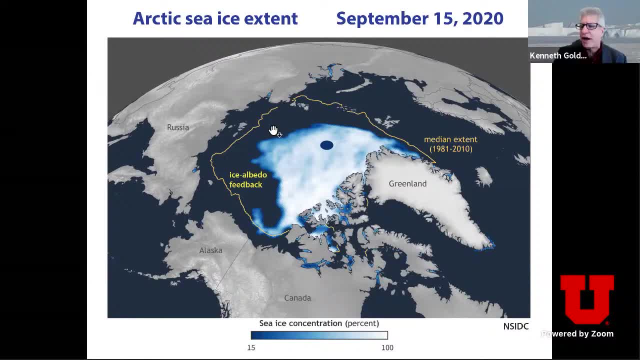 All the way up to the ocean reflective surface um is replaced by a darker uh absorptive surface- name of the ocean- then that further warms the ocean, which melts more ice, which recedes further, which exposes more darker surface and it feeds on itself and this is called ice albedo feedback, which is one of the principal. 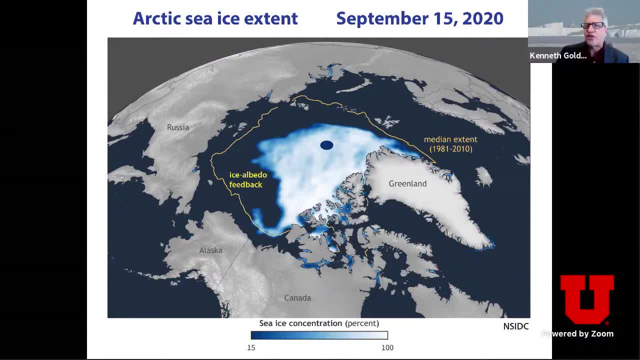 mechanisms that help, that is, helping to drive um the precipitous losses that we're seeing um, particularly in the arctic. and the other feature i'd like you to notice here is this hole right in the center there of the sea ice concentration field, and this is a perennial. 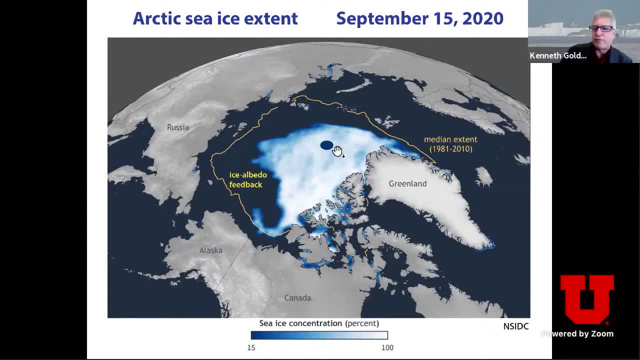 feature. this is. this is um basically the the way from the way satellites are configured and the way they take their images. um. this hole was much bigger earlier on and um one of the um. it used to not matter too much. it was thought not to matter because, um, they figured well, the there. 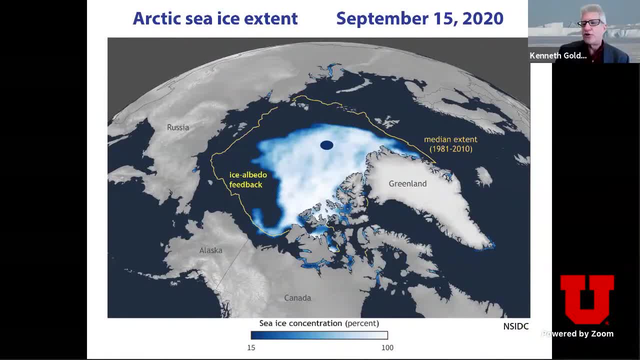 there's pretty much 100 concentration there, but that's not the case anymore. so to fill in the climate data record, it's really important to understand what's going on in there and you'll see later on. um, that's one of the sort of mathematical uh, uh, magical types of um uh. 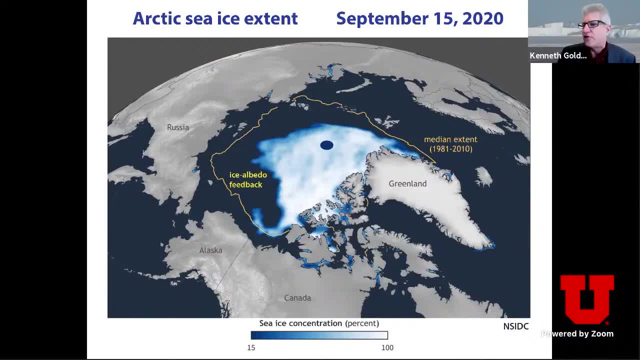 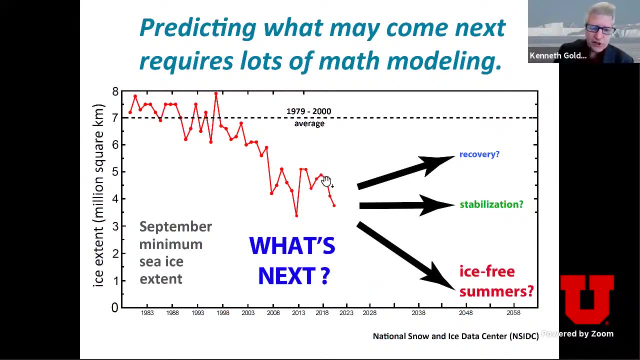 techniques that we've developed, along with some of the theory of partial differential equations, to try to fill in that hole and, um, uh, to add to uh, fill in the gap, the inherent gap that we see in the sea ice concentration field. okay, now the main sort of the main point of this talk and kind of 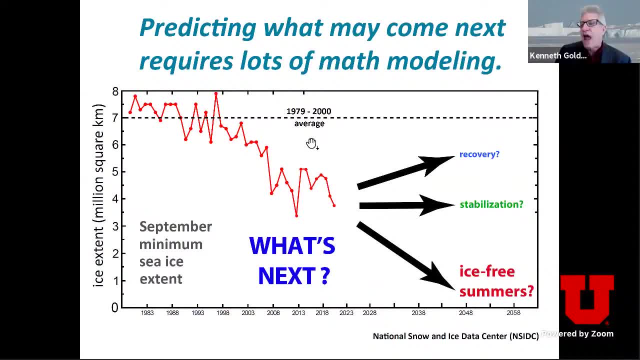 what we're doing is we're going to look at what's going on in the sea ice concentration field. and what we're doing is we're going to look at what's going on in the sea ice concentration field and, well, predicting what may come next, be it perhaps a recovery, not too likely. stabilization, not too. 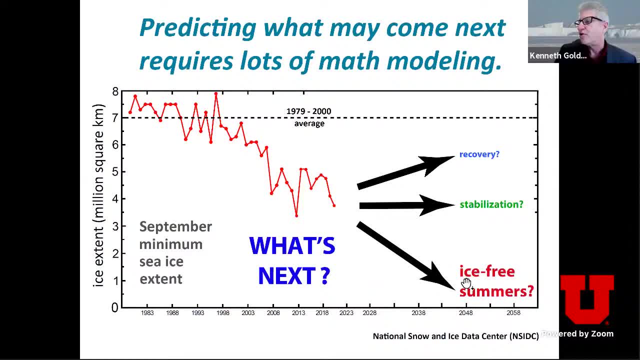 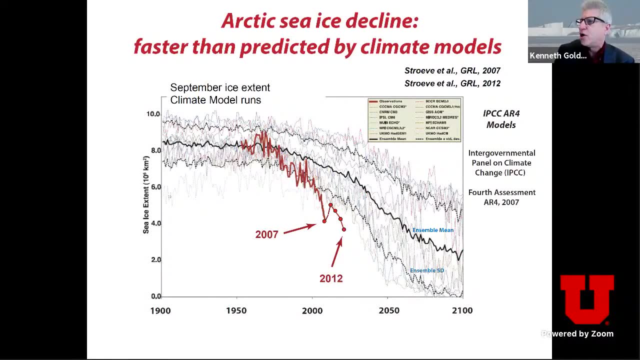 likely, or eventually, ice-free summers at some point uh, predicting what may happen um requires a lot of mathematical modeling, as you uh, as you see, and to put this in what we're doing in some context, some historical context, going back a few years, um, and looking at the uh, the runs of the uh, 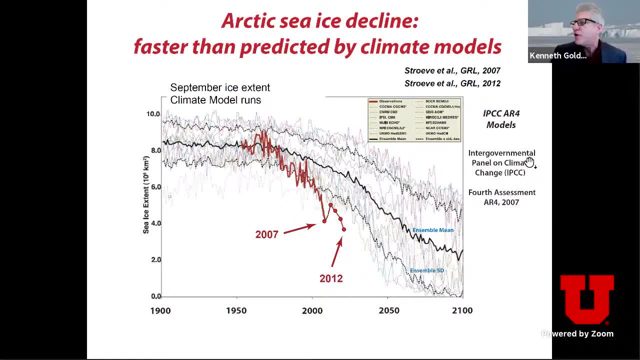 climate models used in these, uh, these these huge reports of the ipcc or the intergovernmental panel on climate change. um, where so? these are roughly the the 20 world's best climate models a few years ago and, uh, they all predict a general decline of summer arctic sea ice over the 21st. 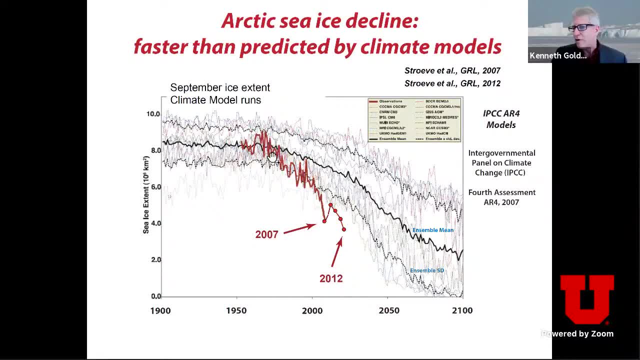 century. here's the mean, here's the standard deviation, and so on, and, however, here's the actual data. so the ice was melting at a much faster rate than any of the world's best global climate models did. so this presents a fundamental challenge: how do we represent sea ice more? 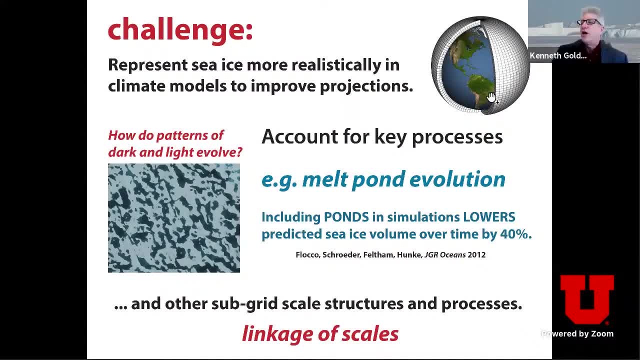 realistically um in global climate models, uh to improve projections and, in particular, how do we account for key processes such as um the evolution of melt ponds shown here, these patches of of dark and light on the surface of melting arctic sea ice? there was an early study showing that, if you 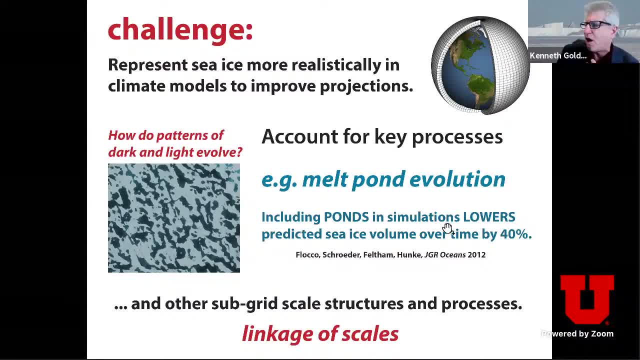 include ponds in simulations over pretty long periods of time, this can lower the predicted sea not by a tiny, tiny amount, but by almost 40 percent, And so this is one of the fundamental challenges of sea ice modeling- is how do you incorporate these processes that are happening? 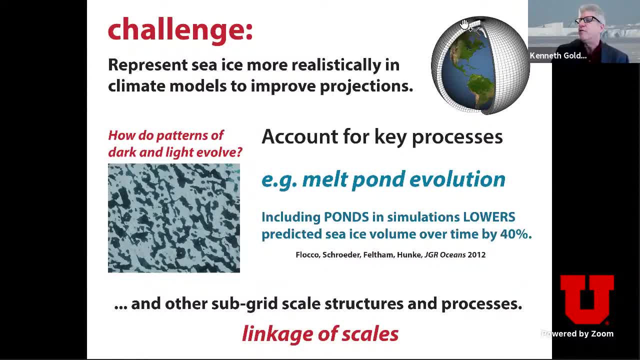 on much, much finer scales than the grid sizings, the grid spacings of typical global climate models, as well as large-scale sea ice models, and how do you account for such processes rigorously in these larger-scale models, And this is particularly challenging in the case of sea ice? 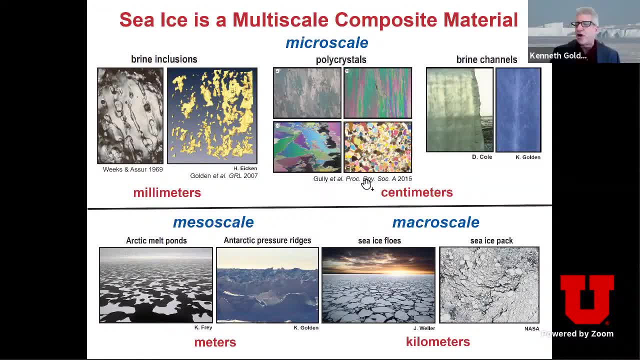 which is a multi-scale composite material which exhibits complex composite structure over length scales ranging over about 10 orders of magnitude. So even at the finest scale, the submillimeter scale, as you freeze seawater, you can't incorporate the salt into the crystalline. 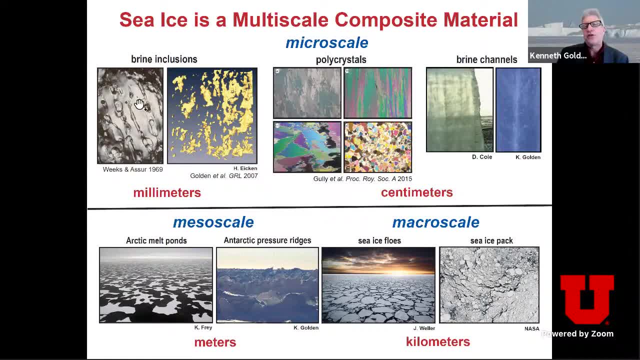 structure, and so you get these inclusions of salty water that are laced throughout the sea ice, and their volume, fraction, geometry and connectivity depend dramatically on the temperature. Sea ice is also a polycrystalline composite material, shown here, where the polycrystalline structure depends strongly. 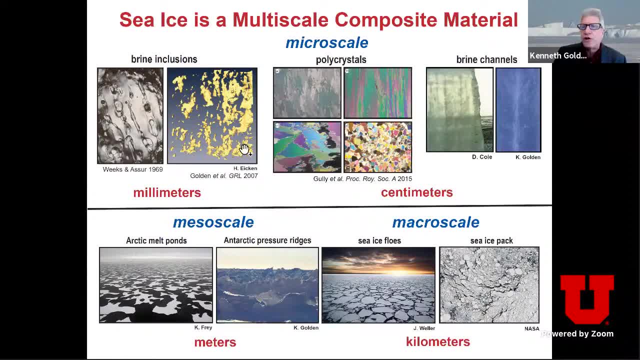 on the conditions under which the ice was grown. These brine inclusions can connect up to form meter-scale channels through which fluid and flow, which controls a lot of very important processes. as we'll see, Moving up in scale to the so-called mesoscale, we have the melt ponds as well as, say, pressure ridges, when 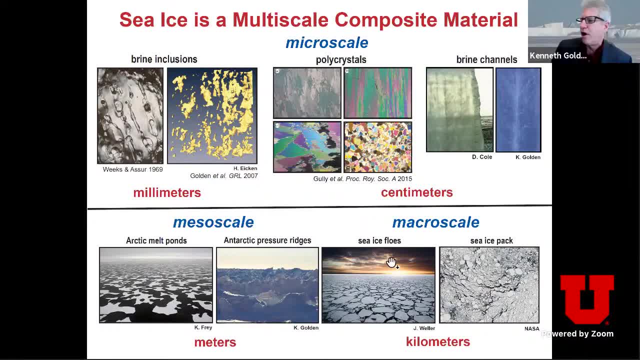 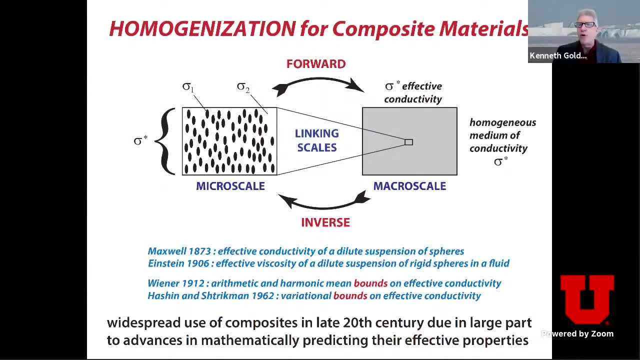 the ice crashes together and then up in the largest scales of sea ice flows, and looking at the ice pack, say from space, or the entire- say Arctic basin. Now, when you're dealing with a composite material, you're often most interested in what are the effective or overall 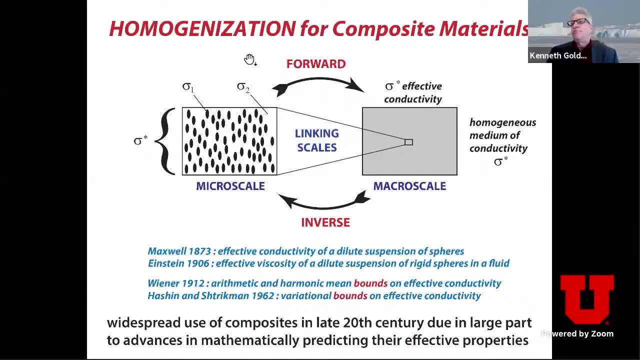 properties. This is called homogenization, and this is one of the main things that we do- sort of that a lot of the faculty here in mathematics are interested in, in these types of problems, which I'll tell you about in a second, And so here we might have a two-phase composite material. 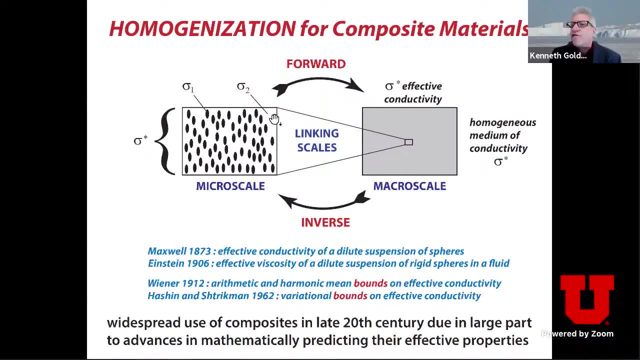 say, a good conductor- conductivity sigma-1,- embedded in a host of, say, a core conductor of conductivity sigma-2,. and then we want to step way back and find, say, a homogeneous medium which behaves macroscopically the same as this inhomogeneous medium, and then the conductivity of 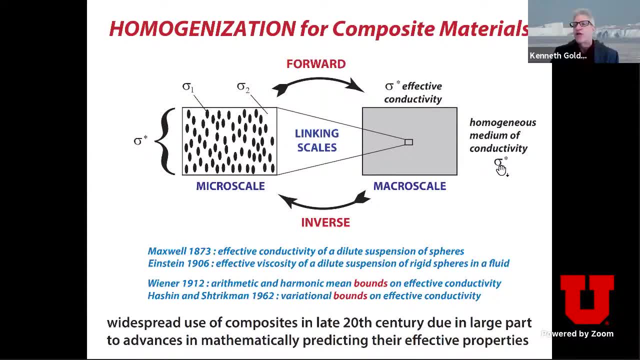 that homogeneous medium. that is the effect of conductivity, the overall or effective behavior, And that's the forward problem, where you're given information about the microscale and then you want to find the effective behavior. But then a very important problem going the other way. the inverse problem is to where you're given information about the bulk properties and 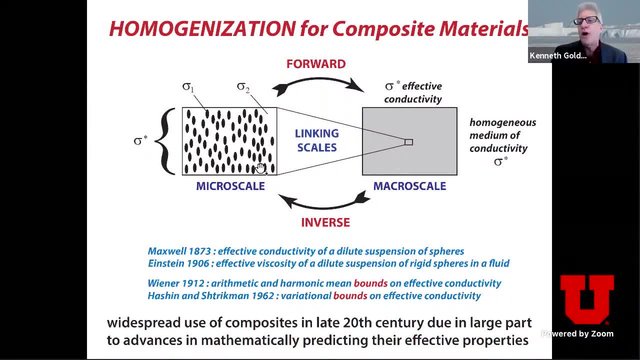 you try to infer or plot the effect by variables to get the correspondingounty of the behavior. Has a infer or figure out what's inside the black box, namely what it's going on inside, say, the sea ice, or what's going on in the microstructure, And these problems have a 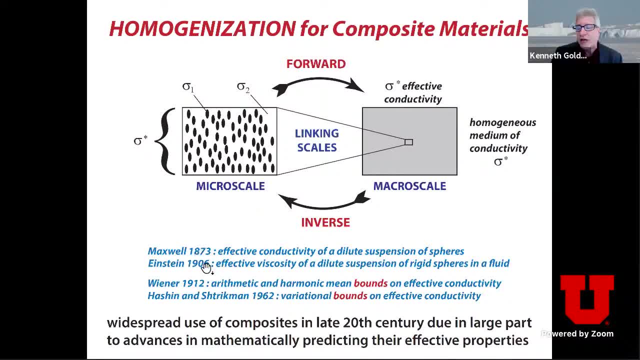 very long and storied history. Scientists such as Maxwell and Einstein have worked on these problems And there have been a lot of advances throughout the 20th century and a lot of work on trial and error, on trying various microstructures and so on and seeing what kind of properties you get. 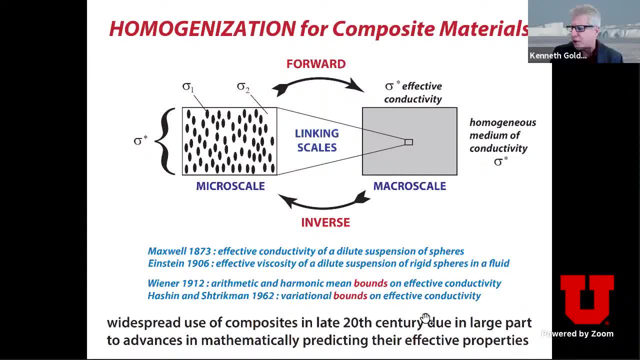 However, the widespread use of composite materials in the late 20th century was due in large part to significant advances in mathematically predicting the effective properties of composite structures And, fortunately for us here and for somebody like me who works on sea ice, which is a 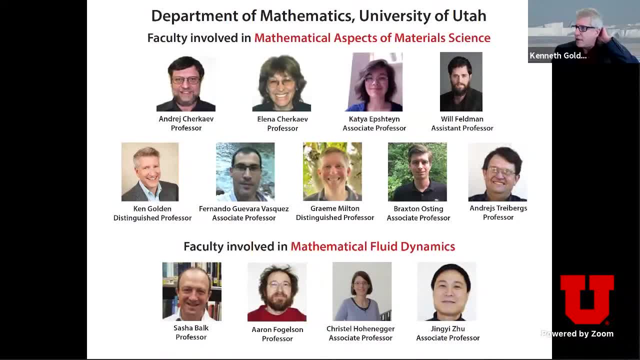 composite material. we have a lot of faculty in the mathematics department that are involved in mathematics, And so we have a lot of faculty in the mathematics department that are involved in mathematics, And so we have a lot of faculty in the mathematics department that are involved in. 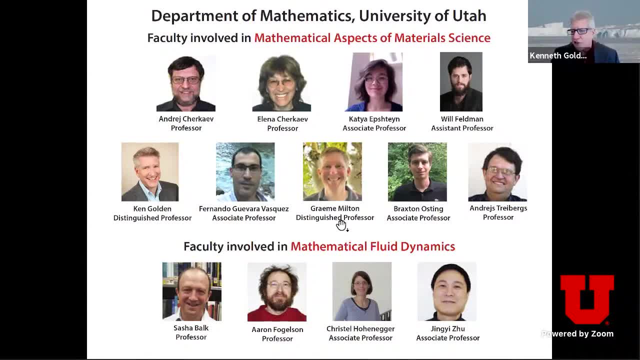 mathematical aspects of material science as well as faculty involved in related problems. in mathematical fluid dynamics There's world-renowned advances and people working in optimal design in inverse problems, going the other way in polycrystalline problems and phase transition, developing numerical methods, And so one of the 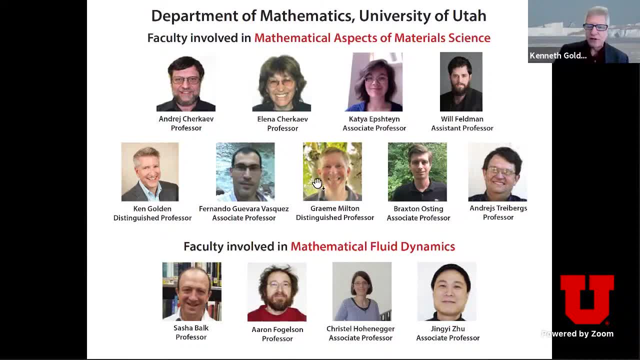 really exciting areas is cloaking or making things invisible. Yes, I mean like Harry Potter, And I think what's interesting is that these things are going on in a mathematics department, So you might want to check that out a little bit, And it's been extremely exciting for me. 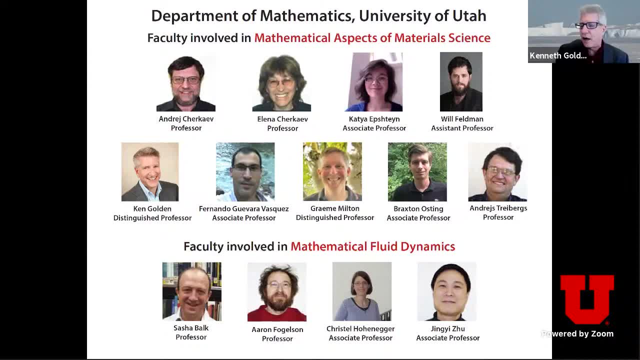 to be closely connected to all these great faculty in the mathematics department who are interested in composite materials, and in particular, Elena Cherkaev and I have worked extremely closely over many years on problems involving sea ice, And so I think it's really interesting to be able to connect these two. I'll give you a little bit more detail about 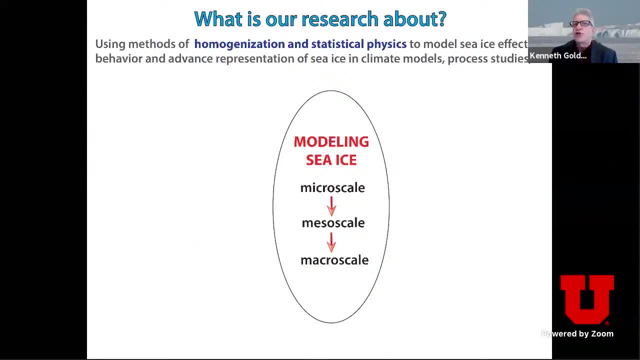 what is sea ice and bring into bare methods of composite materials to study in sea ice. So what is our research about? Well, it's about using methods of homogenization coming from composite materials, as well as statistical physics to model the effective behavior of sea ice. 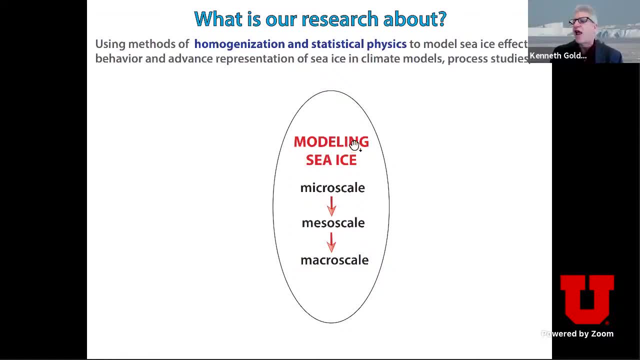 and advance how sea ice is represented in climate models and process studies and so on, And moving up in scale, say from knowing information about the microscale, figuring out what then happens on larger scales, knowing what about the mesoscale property such as the ice pack characteristics, and then figuring 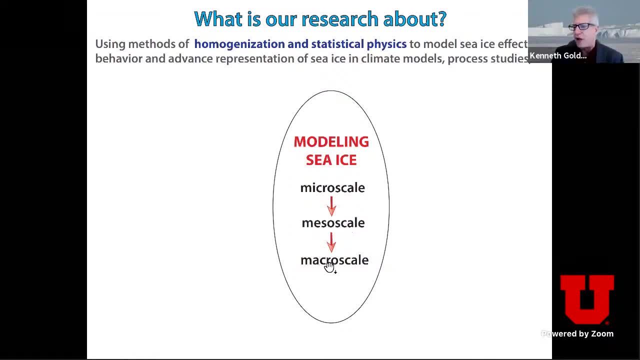 out well what happens on the much larger macro scale And one of the I think that the real takeaways that I'd like you to get from this presentation is that I think one of the things that distinguishes how we approach this as mathematicians is that we are very interested. 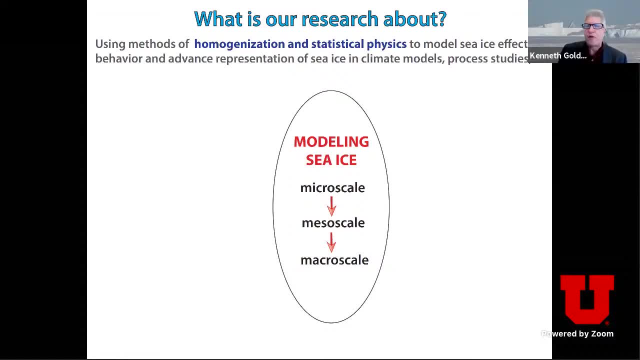 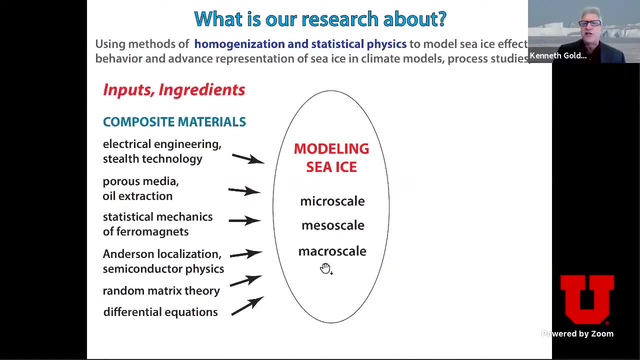 in using mathematical techniques that are relevant, but we don't really care where they come from, And they come from a broad range of other areas of science and engineering. So the inputs and ingredients that we use to study sea ice, we're bringing, of course, a lot of. 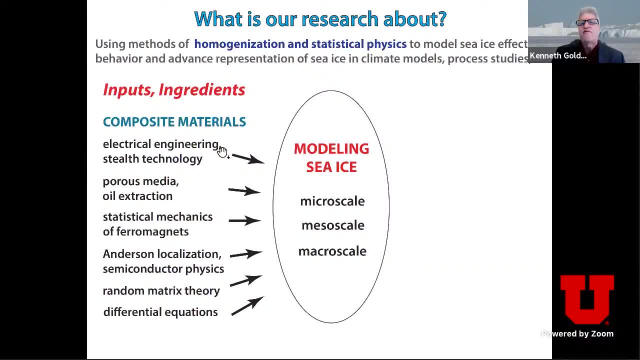 techniques and mathematical methods from composite material. We're bringing in a lot of electrical engineering, including stealth technology, a lot of the mathematics and physics of porous media which originally, which a lot of that work originated in oil, the problem of oil extraction. 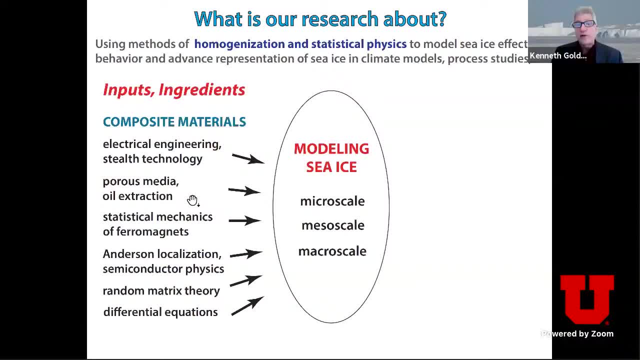 but has now been turned around into carbon sequestration. We'll be using the statistical mechanics of carbon sequestration. We'll be using the statistical mechanics of carbon sequestration. We'll be using the statistical mechanics of magnetic materials and even Anderson localization. 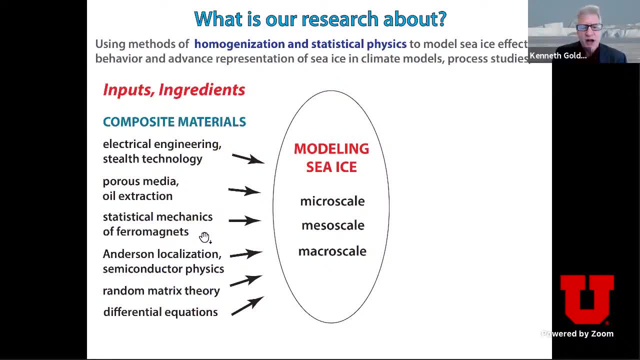 and semiconductor physics, And then many areas from mathematics, such as random matrix theory, differential equations, stochastic processes, functional analysis, complex analysis and so on. It's such a diverse studying sea ice is such a highly interdisciplinary area that we're able to 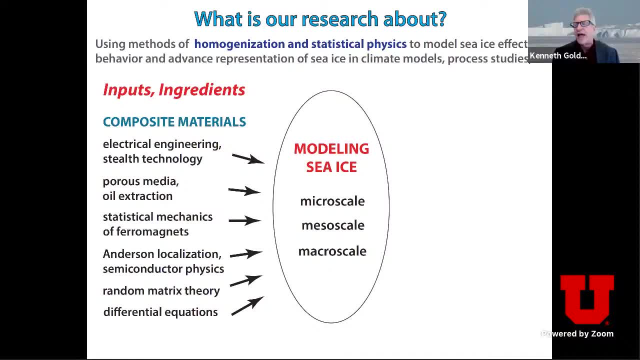 use and bring in so many different kinds of methods and ideas to play. And then, on the flip side, we have a lot of applications. We have a lot of applications to other areas of science and engineering because, again, sea ice touches on so many different. 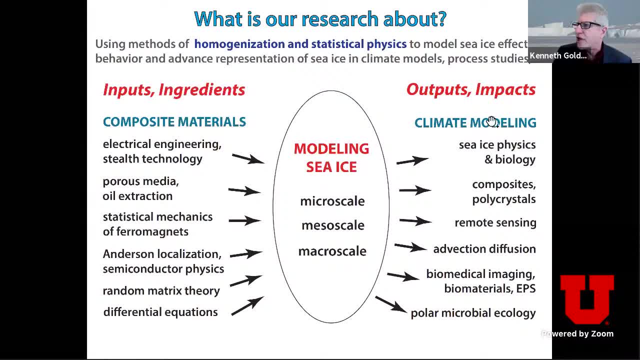 areas and different types of structures. Of course, we're having implications to climate modeling. Some of our methods and techniques and results have been used in, in fact, advancing large scale climate models. We get results, of course, in sea ice, physics and biology, But then also again, as I mentioned in the video. 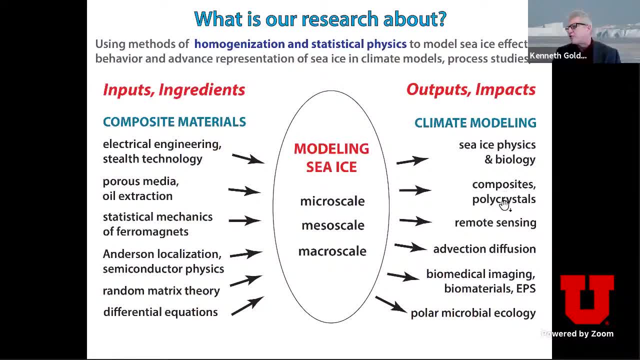 we are proving general theorems about composite materials such as polycrystals and so on. A lot of our earlier work centered on the electromagnetic properties of sea ice, which then has applications to remote sensing, and using satellites and airplanes and helicopters to figure out what's going on in the ice. 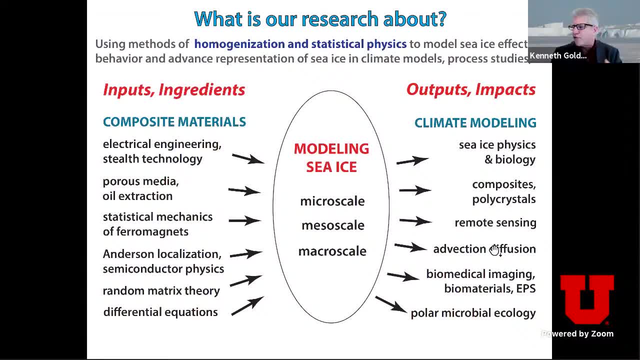 Also we're very interested in advection diffusion processes and have proved a lot of general results there, where you have not only say diffusion, like heat transported through sea ice, but there's fluid moving helping to move, move the heat around. Biomedical imaging like this method of 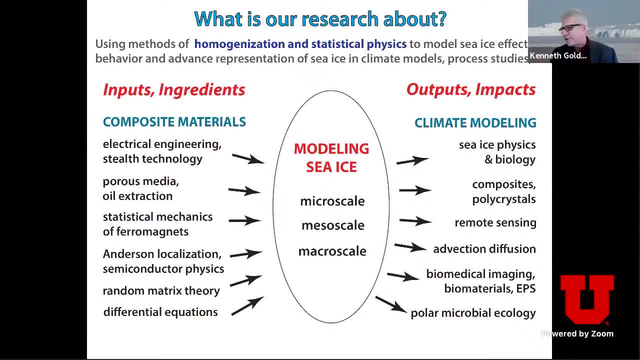 monitoring osteoporosis, where of course you know the bone doesn't, the mathematics doesn't care if it's bone or sea ice or whatever. You'll hear a little bit in a second about some other biomaterials And we're getting really interested lately in polar microbial ecology and using the advances that we've made in sea ice, physics and what is that, and the mathematics and what does that tell us? how can that help us advance models of polar microbial life? 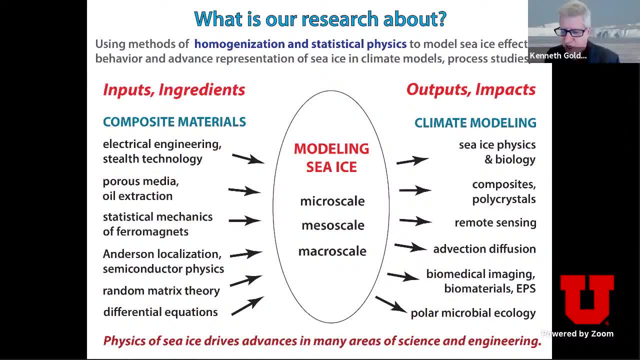 So, one of again, one of the key takeaways here is that the physics of sea ice drives advances in many areas of science and engineering, And what you're going to see is where we take ideas and methods from seemingly completely unrelated areas of science and engineering and bring them to bear on sea ice and vice versa, where we take 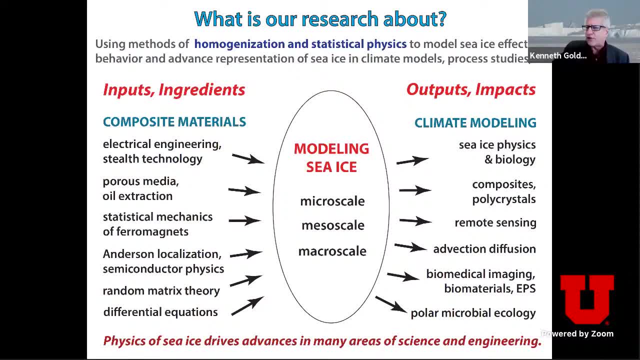 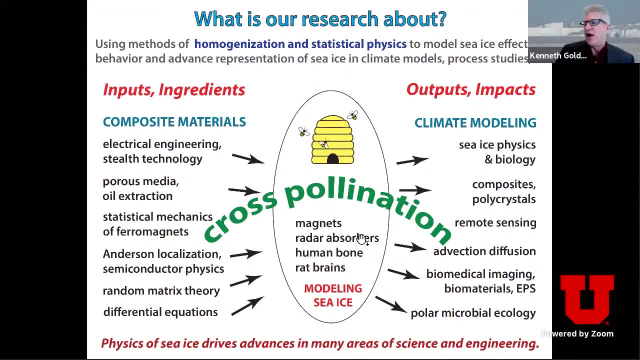 mathematics and physics and ideas where we've developed for sea ice and are able to apply that those ideas to completely seemingly unrelated areas of science, engineering and medicine and so on. And I call this cross pollination. And here you see these bees. you know what could be more appropriate for Utah? This is one of the symbols of Utah And there's a lot of connections to a lot of very interesting problems again in science and engineering: magnets, radar absorbing materials, human bone and, as you'll see, even rat brains. 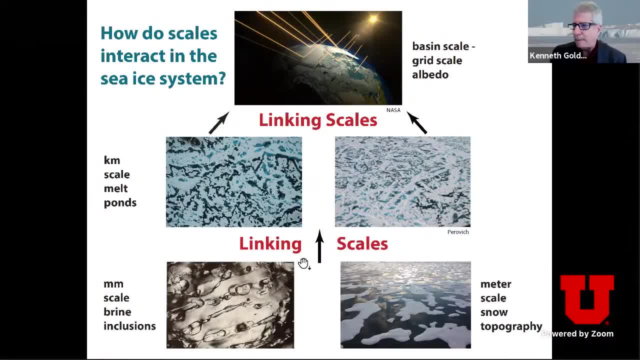 Okay, so how do these scales link up? Well, let's look at this, one of the central problems here: The micro scale of the sea ice, the brine microstructure, ultimately determines its fluid permeability properties, how easy it is for fluid to flow through the ice, which then sort of sets the water level here. 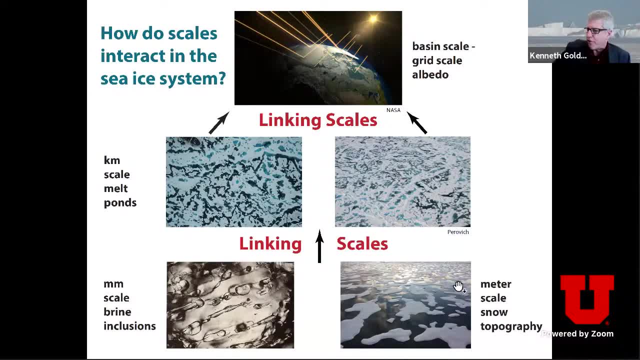 and how that interacts then with the meter scale topography of the snow, which then determines the geometry of these patterns that you see on the surface of melting Arctic sea ice and then ultimately on the basin scale. we're interested in the overall albedo reflectivity, or the 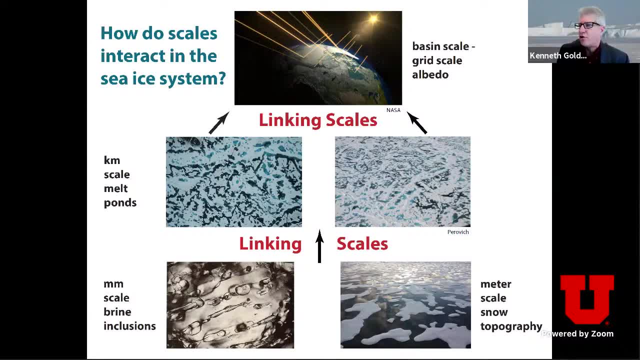 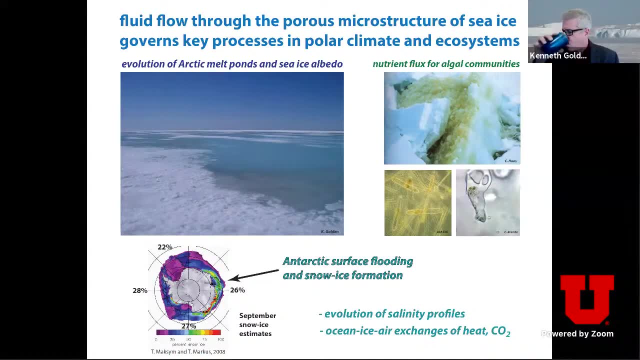 bulk effective behavior of the whole system At that very, very large scale. So let's focus on the microphysics of sea ice and fluid transport. So fluid flow through this porous microstructure of sea ice governs key processes in polar climate as well as these key polar ecosystems. So whether or not these ponds grow or drain overnight, completely changing the albedo, depends on how easy it is for fluid to flow through the porous microstructure of sea ice. 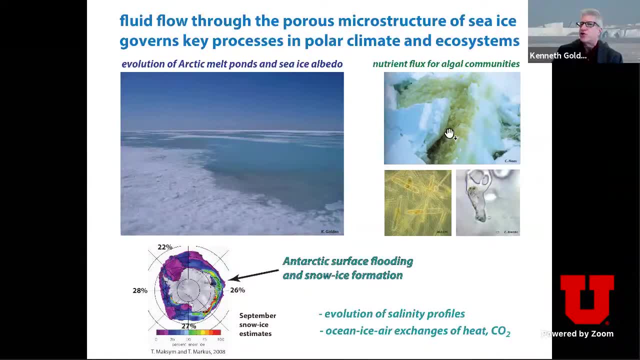 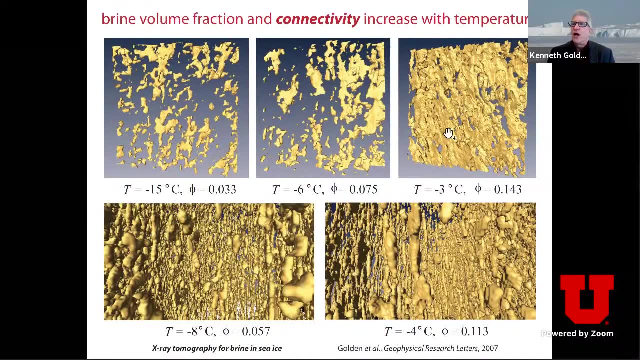 And these algal compounds. they get their nutrients through nutrient-laden seawater percolating through the brine microstructure of sea ice. So here's sort of some of our X-ray tomography of the brine microstructure of sea ice. 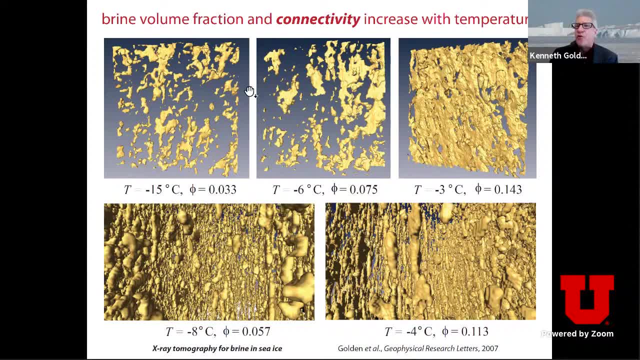 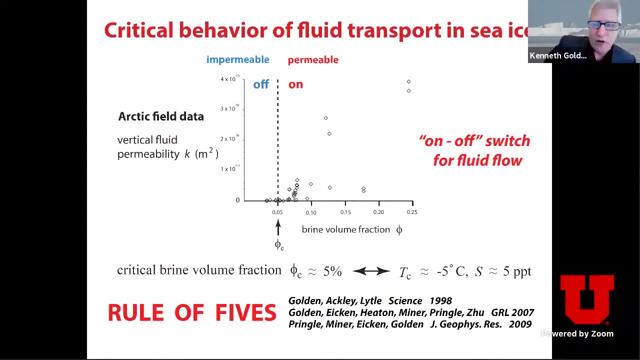 and showing the significant dependence of its connectivity and brine and volume fraction on the temperature. No pathways, one pathway, many pathways, and you can see the significant changes with relatively small changes in temperature. Now, one of the key phenomena, one of the key aspects that I've sort of uncovered was a sense about sea ice physics, which controls a lot of the 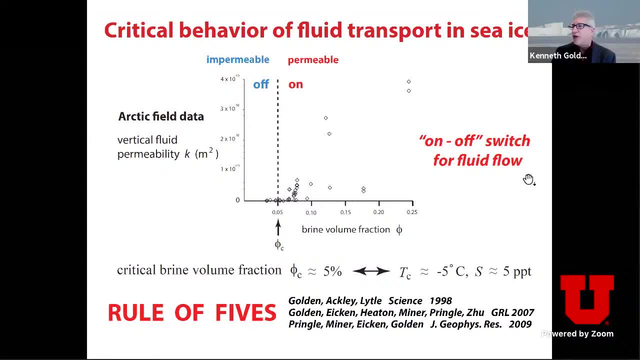 processes in sea ice that are important for the climate system as well as the biology, is effectively the on-off switch for fluid flow, And so for brine volume fractions below about roughly 5%, for so-called columnar sea ice grown under quiescent conditions. 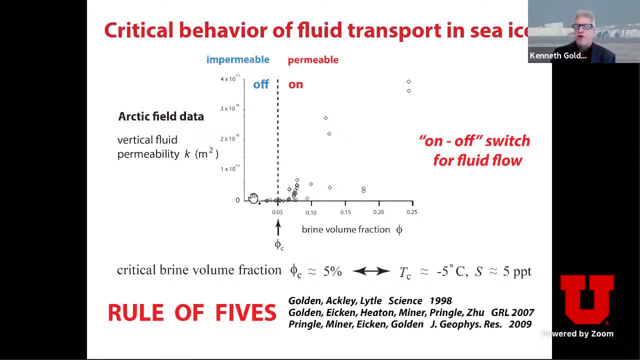 then the sea ice is effectively impermeable. The vertical fluid permeability is very, very small. But for brine volume fractions above 5% the fluid permeability grows and it's permeable and fluid can flow. and this critical brine volume of 5% corresponds to a critical temperature of minus 5 Celsius for a typical bulk salinity of about five parts per thousand, which has become known as the rule of fives. 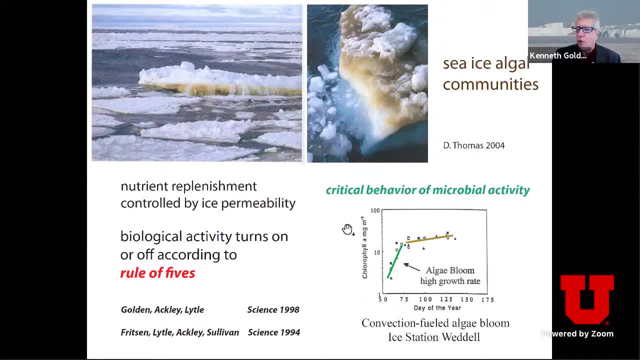 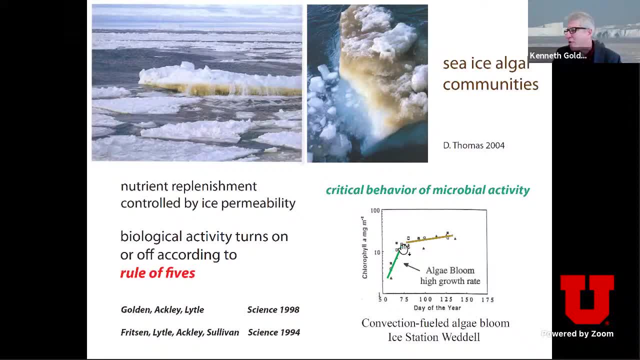 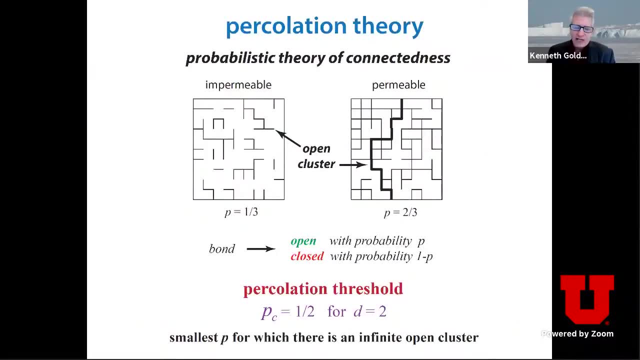 And basically that's the on-off switch. There's this rapid run up, rapid bloom, and then it effectively shuts down. That's the on-off switch. Now, why does this happen? What's the underlying idea? What's the underlying mathematics? Well, it's a percolation threshold. 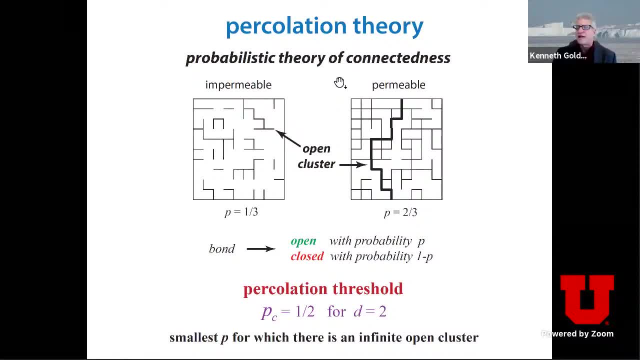 This is the percolation theory, is the probabilistic theory of connectedness. We start, say, with a two-dimensional infinite lattice in two dimensions which is square, and a bond is open with probability p, closed with probability 1 minus p, And then here's a configuration where about a third of the 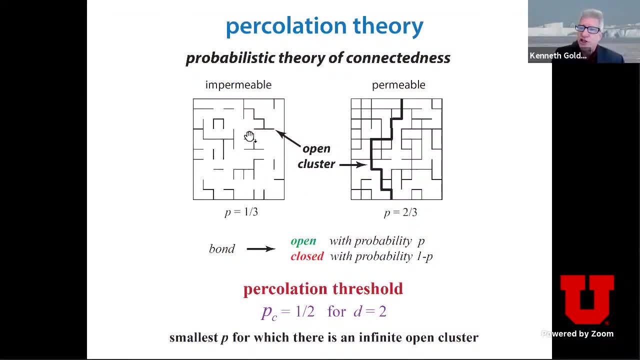 bonds are open, and so if fluid or electricity tries to get through here, well, it can't get stuck. Here's about two-thirds of them filled, and then there's an infinite pathway. This is a permeable state, And then you might ask: well, what's the smallest p for which there's an infinite? 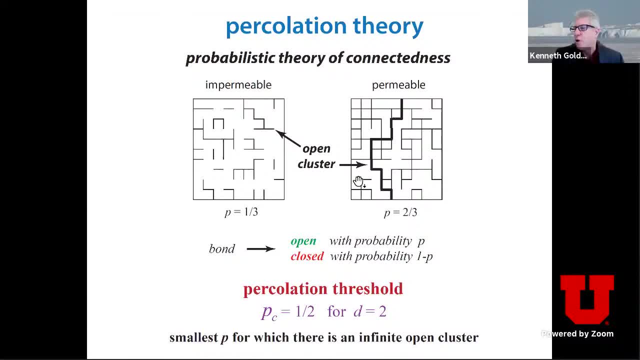 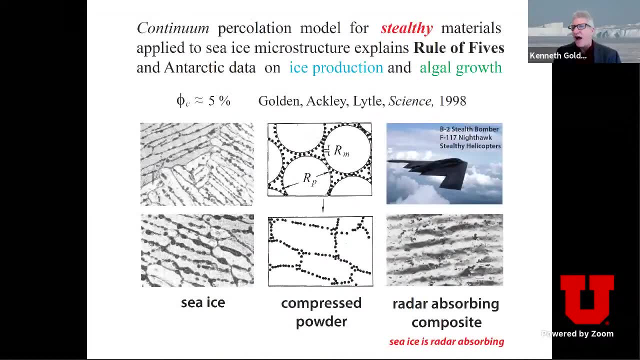 open cluster for which fluid can flow, And for this two-dimensional square lattice it's exactly one-half or 50%. So then the question would: be well, why is sea ice so small? 5%? Well, it's because you have an excluded volume effect, where the Brine inclusions are not all randomly. 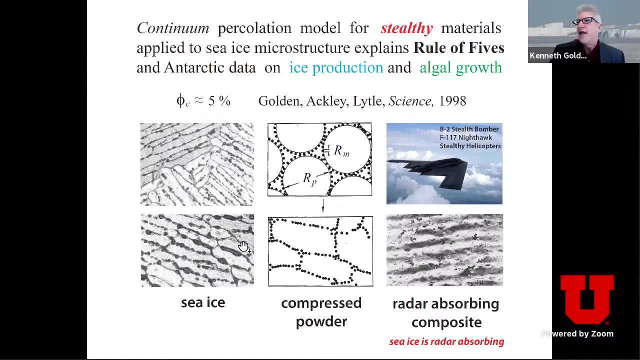 distributed, but they live on the boundaries of the little ice, And so you have an excluded volume effect, where the Brine inclusions are not all randomly distributed but they live on the boundaries of the little ice platelets. And then? so how do we? 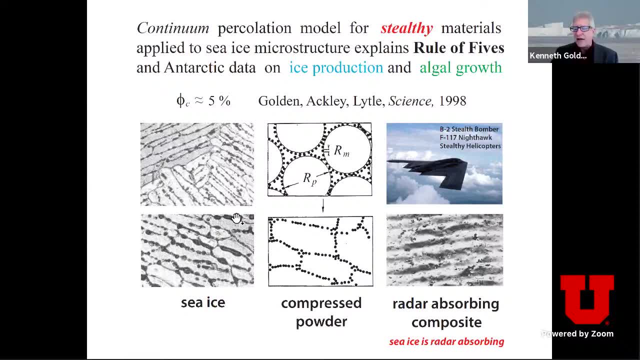 predict that? Well, it turns out that if, again side by side, if you compare the microstructure of sea ice to the microstructure of so-called compressed powders- big polymer spheres and little metal particles squashed together so that you can achieve radar-absorbing capabilities and 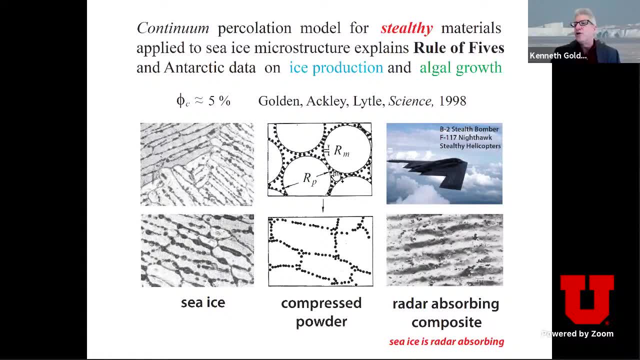 connectivity with very low volume fractions. then we use the continuum percolation model developed for compressed powders to predict the 5%. And what's so fascinating, though, is that these materials were used in the development, again, of stealthy material coatings that they put on aircraft to make them be able to be invisible. 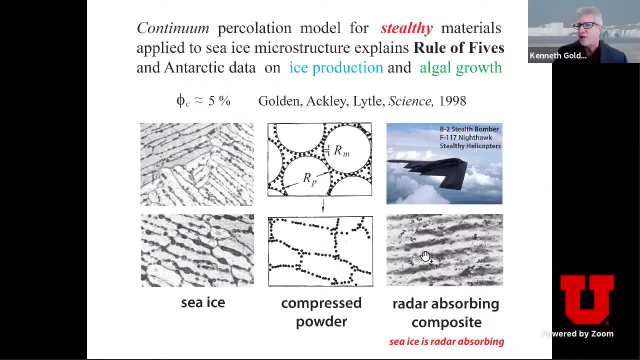 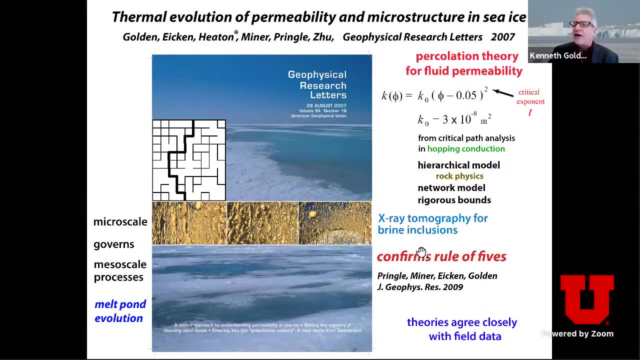 to radar, And, in fact, sea ice, then, is a radar-absorbing composite as a result of this similarity. Now the next big step is to well, how does the permeability depend? on the volume fraction or on the temperature above the threshold? And so this: 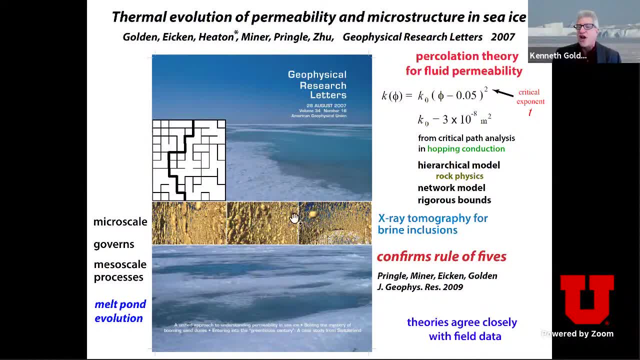 I like to view this cover in geophysical research letters as sort of a homogenization axon. This is about a centimeter across. How does the microscale control the macroscale processes, such as the evolution of melt palms? And we developed a beautiful percolation theory for. 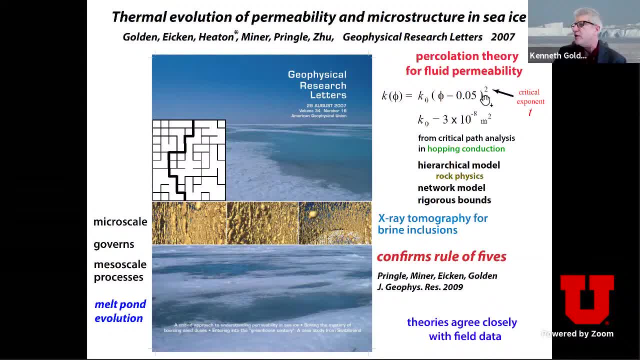 the fluid, the vertical component of the fluid, permeability in sea ice- And this is a deceptively simple formula- where there's the 5%, where the permeability takes off, This is the best known value for the critical exponent in three dimensions And I actually did a lot of. 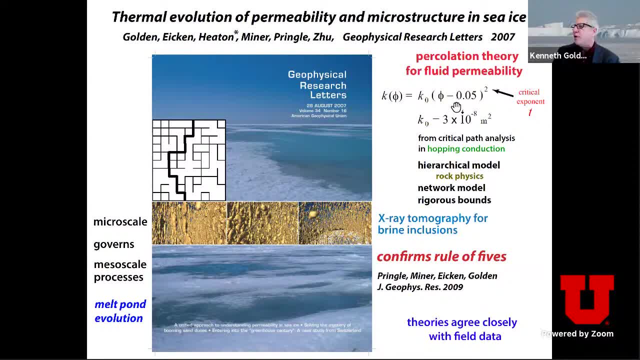 mathematical work earlier in my career on these critical exponents And then this constant in front. you might think it's sort of a free parameter that you adjust to match the data, but that's not it at all. We use our X-ray tomography data to find the bottlenecks. 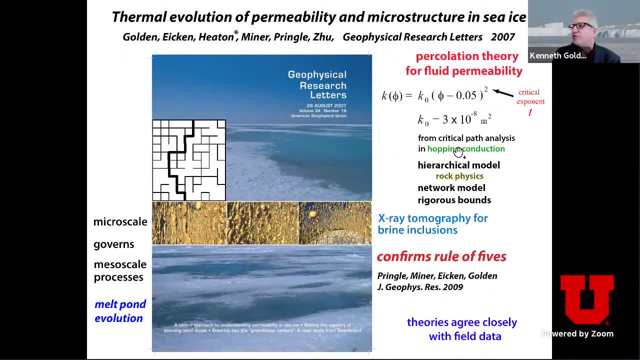 in the pathways, in the fluid pathways, And then we use so-called critical path analysis, which was originally developed in the context of hopping conduction in semiconductors. So we apply that theory, as well as our X-ray tomography, to actually 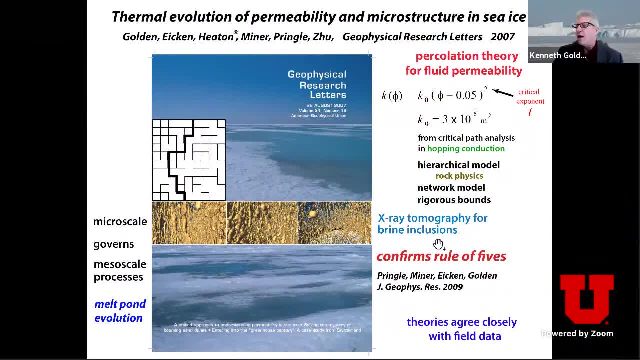 estimate this parameter And then, many, many years after we originally conjectured it, finally, this X-ray tomography, and then the mathematical analysis of the connectivity of the brine microstructure, allows us to finally confirm this rule of fives. Now this is all well. 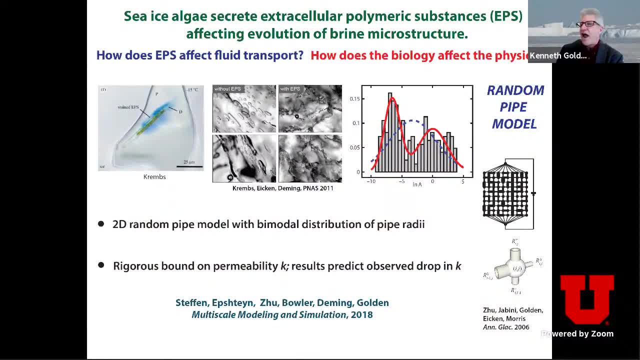 and good when your ice doesn't have any biology in it, when it doesn't have any algae living there. However, to help them thrive in these extreme conditions, we have to be able to estimate this parameter. And then we have to estimate this parameter, And then, many, many years after we originally 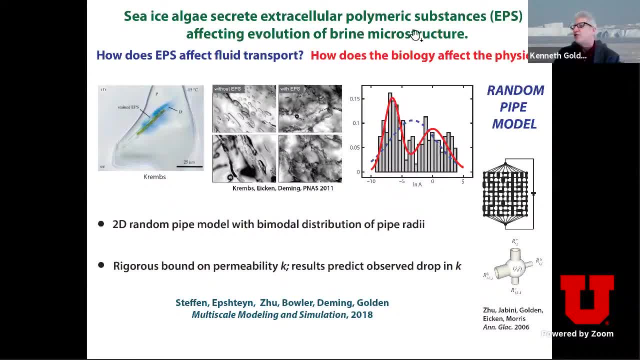 CONNECTED TO THE CONNECTION THAT THE ALGAE HISTORY DEPENDING ON THE FIBLE IS UNDERSTATED. they are extremophiles. sea ice, algae, secrete extracellular polymeric substances Which affect the evolution of the brine microstructure. So we ask the question here. 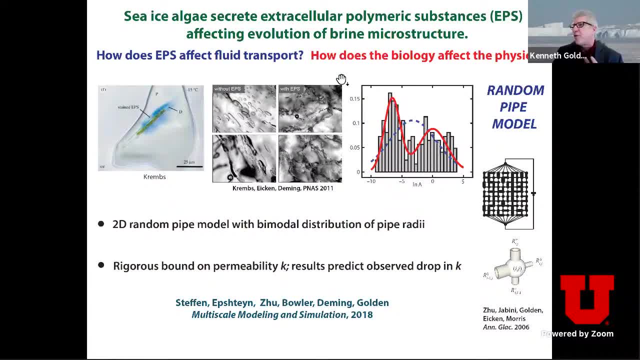 how does EPS affect fluid transport in particular, having the biology affect the physics. So here's a n algal cell And then the blue is the EPS, the extracellular polymeric substances. Here's sea ice without EPS. with EPS It sort of messes up the brine microstructure and changes. 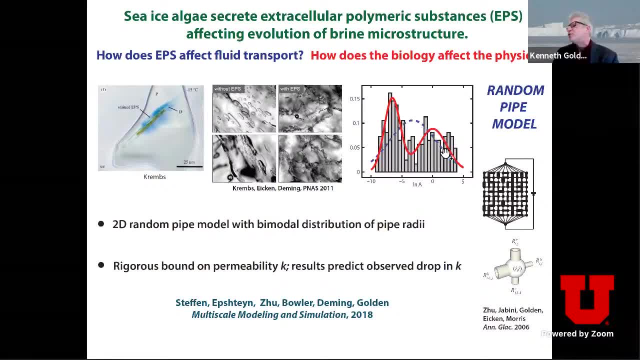 CONNECTED TO THE CONNECTION THAT THE EPS HAVE A LABEL CELL WOULD AFFECT FLUID TRANSPORT TO THE EPS AND the distribution of the sizes of the inclusions from a simple log normal to a bimodal log normal, And we've developed a two-dimensional random pipe model which actually sort of explains. 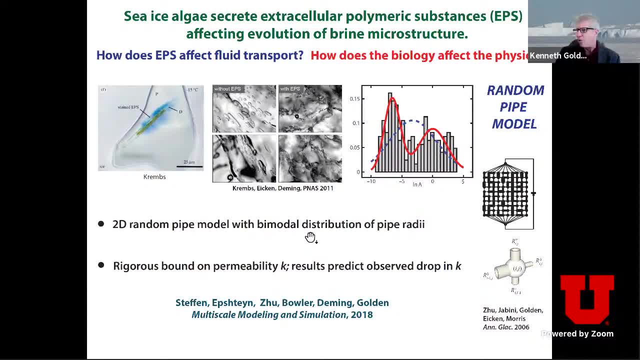 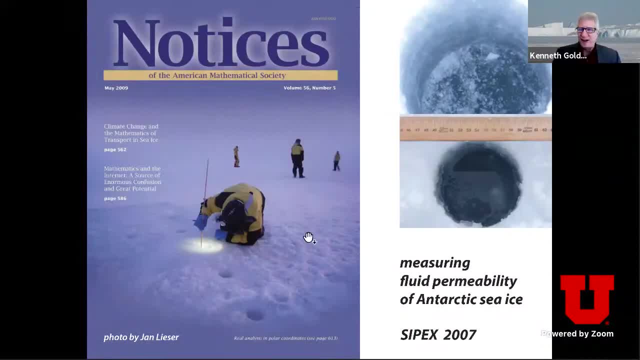 some of the observations And we also develop rigorous bounds on the fluid permeability on sea ice under these conditions. Oh, this is a photo on the notices of the American Mathematical Society from several years ago where I did a big review article on this type of work. 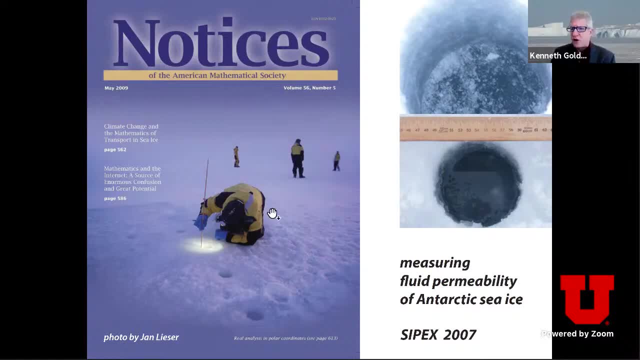 And here I am making the first measurements of fluid permeability in the Antarctic ice pack. And of course this is the cover of a big mathematical journal and this is on a big expedition. And so these three scientists out here, you might think they're involved. 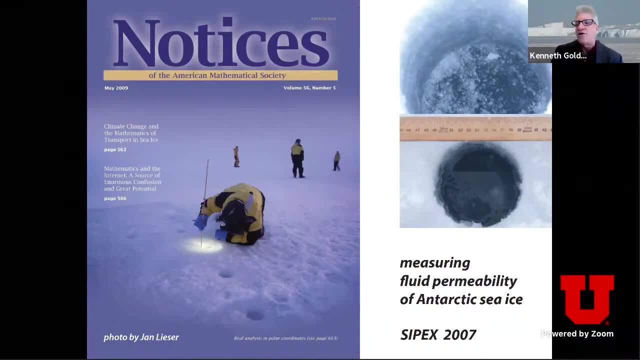 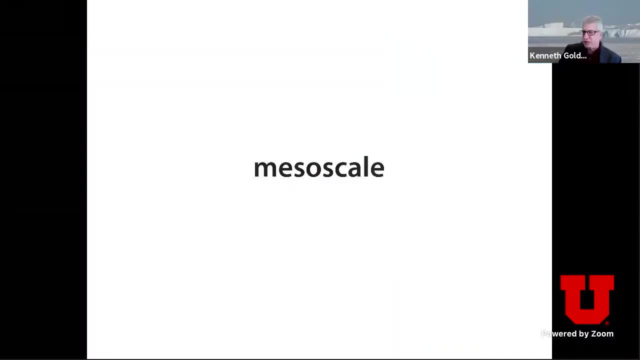 getting an experiment set up. However, they were playing soccer. I was there, I saw it, I participated, so I know what they were doing. Okay, so let's move up to the Meso scale, In particular, focus on again what we saw in the Antarctic ice pack. So we saw the Meso scale. in the Antarctic ice pack, And so we saw the Meso scale in the Antarctic ice pack. And so we saw the Meso scale in the Antarctic ice pack, And so we saw the Meso scale in the Antarctic ice pack. 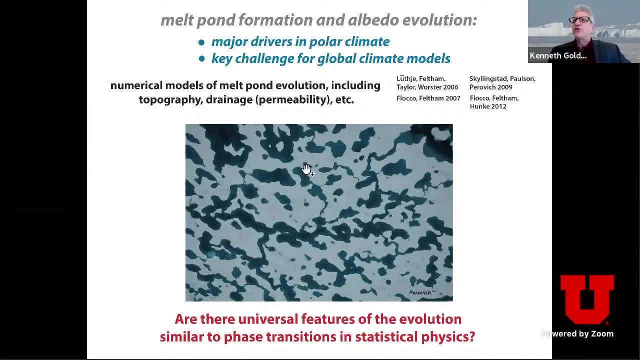 focus on, given what we saw initially, these melt ponds. So melt pond formation and the evolution of albedo is one of the major drivers of polar climate And it's one of the key challenges. And there's been a lot of advances on very detailed numerical models which incorporate, say for, 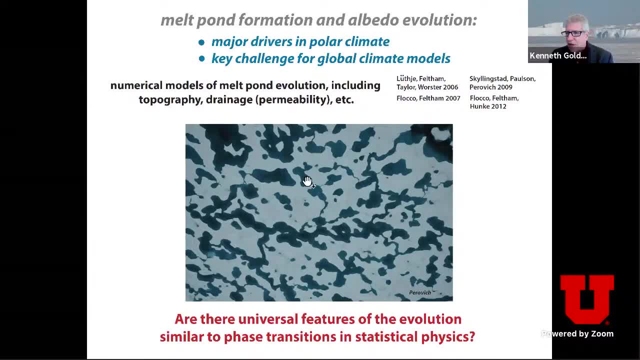 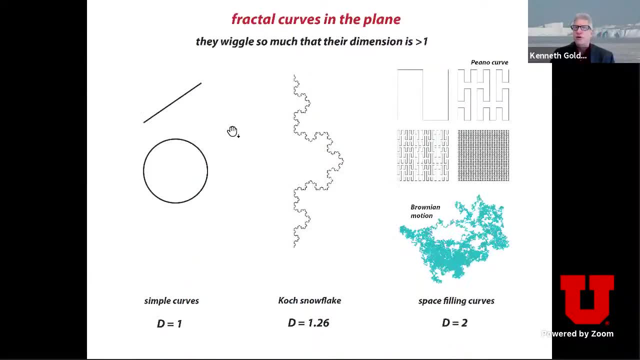 example, some of our permeability results. But I looked at melt ponds and I'd say, hey, that looks like a fractal. Let's ask some more general questions about these types of structures. And so here's just a little background on fractals. If you have a straight line or a 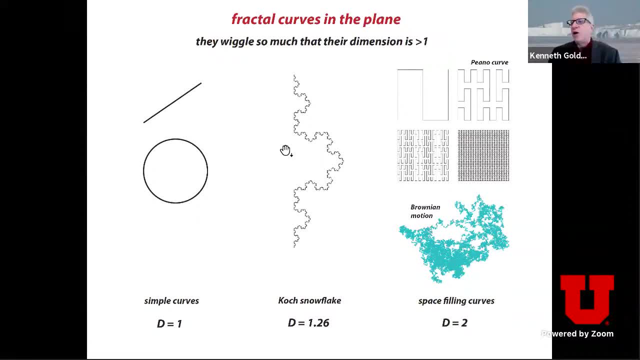 simple curve. this is a one-dimensional curve. It doesn't wiggle at all. But then the so-called Koch snowflake: it wiggles so much. if you zoom in it looks the same, And then it has a fractal. 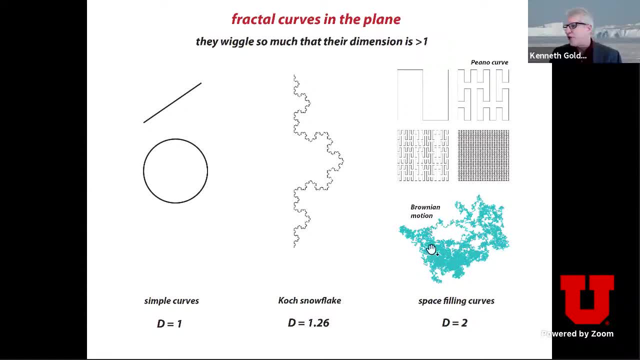 dimension bigger than one, and it's 1.26.. And then the most you could wiggle in two dimensions would be so-called space-filling curves, which have a fractal dimension of two, like Brownian motion or these space-filling curves. 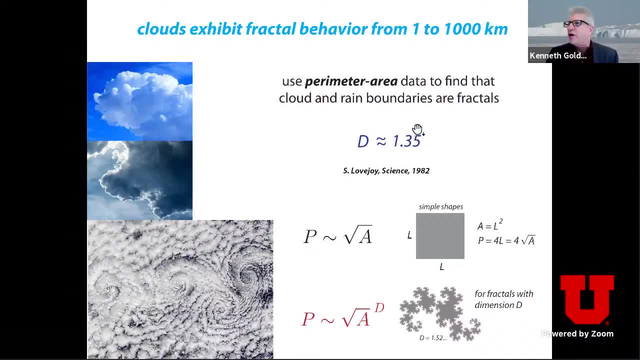 Now, motivated by some beautiful work of Lovejoy, looking at cloud and rain boundaries, then he found that they have a fractal dimension of 1.35.. Now for simple shapes. the perimeter. this is all boils down to an analysis of perimeter versus area. If there's so much perimeter compared to 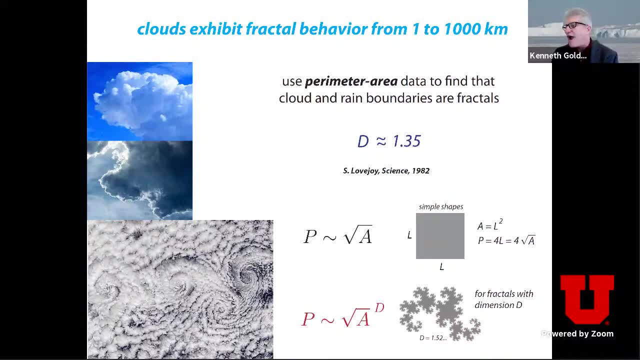 the area. then you start to generate fractally or a fractal dimension bigger than one, And so for simple objects you have a fractal dimension of 1.35.. And then you start to generate fractally objects. the perimeter scales like the square root of the area For fractally objects, the 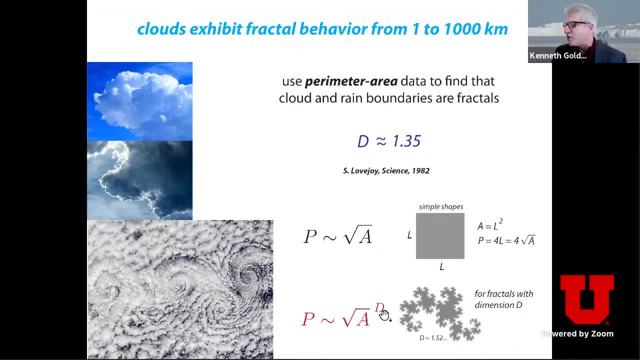 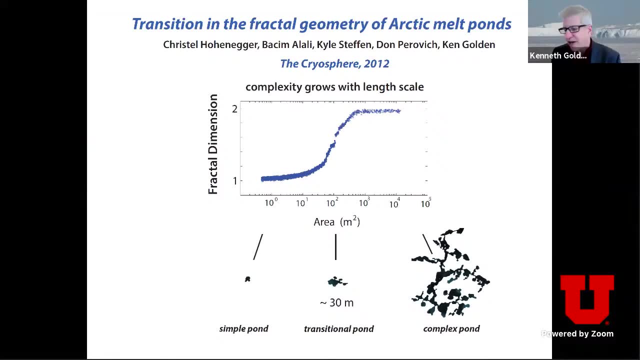 perimeter scales like the square root of the area, to a parameter D, which is the fractal dimension And what we found. so I thought we'd look at melt ponds and find a nice simple fractal dimension, but we found something much more interesting: that we looked at hundreds of thousands of ponds. 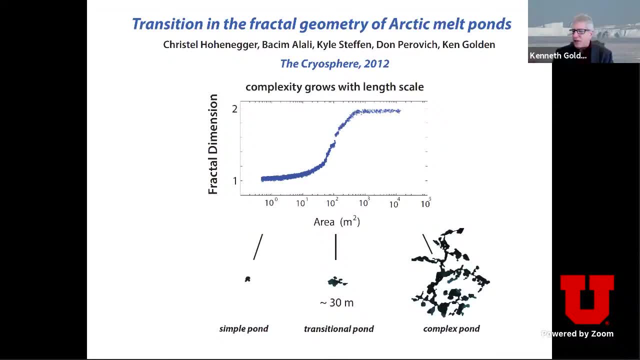 and we found that as they grow and coalesce, their fractal dimension goes from simple Euclidean, from one all the way up to two to basically a fractal dimension. And so we found that the fractal dimension goes from simple Euclidean, from one all the way up to two to basically a fractal dimension. And so we 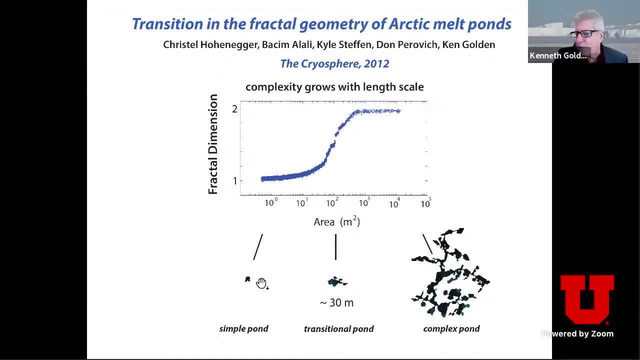 space-filling behavior. So when they're tiny they have these simple ponds have fractal dimension of one, and then they start to grow and become more self-similar And then they become these fully developed, complex, self-similar ponds with a boundary that's behaving like a space-filling. 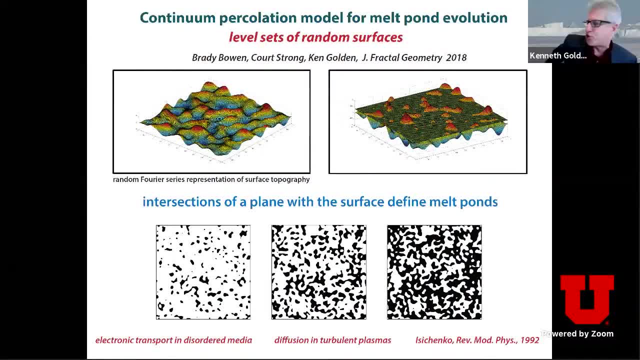 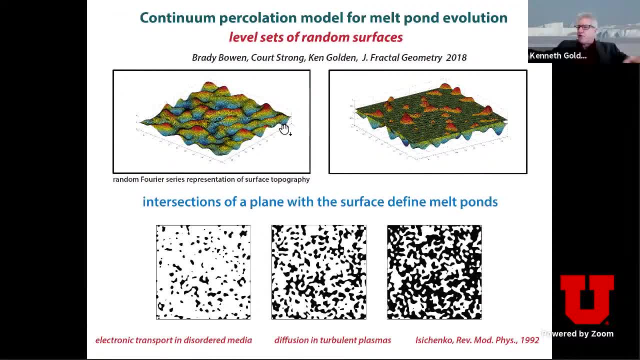 And basically you have a snow topography and then a level set which you can move up and down And as you move it up they coalesce and we can study this beautiful fractal behavior this way, And the motivation for this model came out of diffusion in turbulent plazas from a 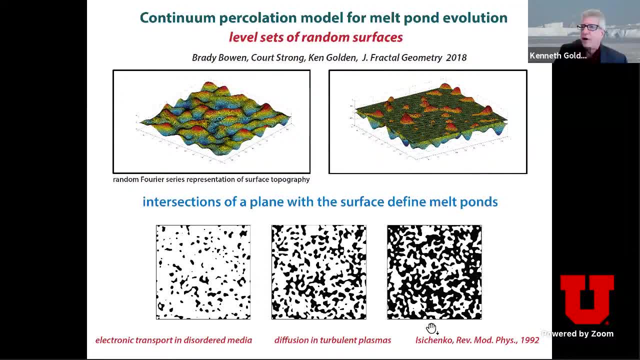 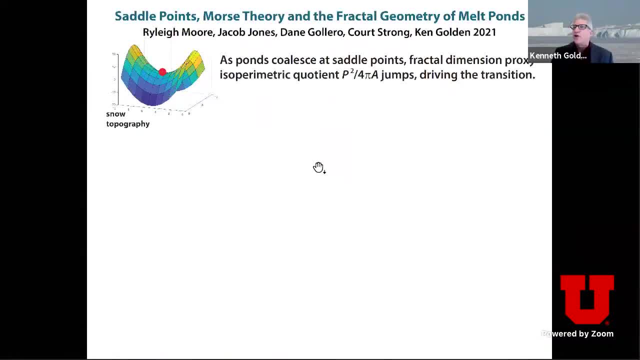 very – a physicist that we met many years ago named Isachenko. Now, if you follow these, the saddle points here, the little points that look like saddles, it turns out that that's the only places where ponds coalesce. And then Riley Moore, a graduate student here in the math department, led a study that shows. 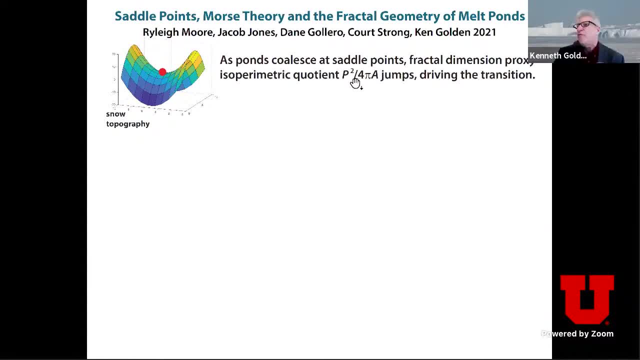 that if we study a proxy for the fractal dimension, namely the isoparametric quotient- the perimeter squared over 4 pi times the area- then as these ponds coalesce, this isoparametric quotient jumps at these saddle points which drives the fractal transition. 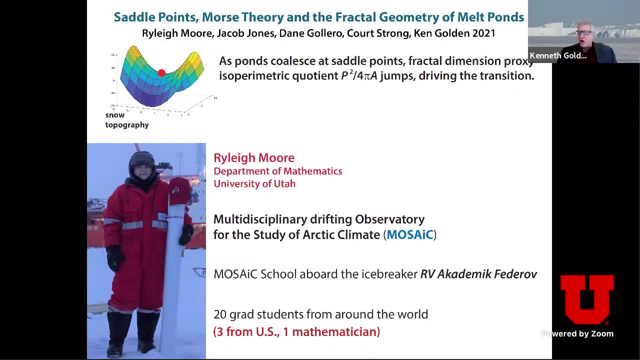 But Riley is also known for having gone – having been the only math student in the entire world accepted as one of 20 graduate students from all over the world to go on the largest – the first leg of the largest Arctic expedition ever: the Multidisciplinary. 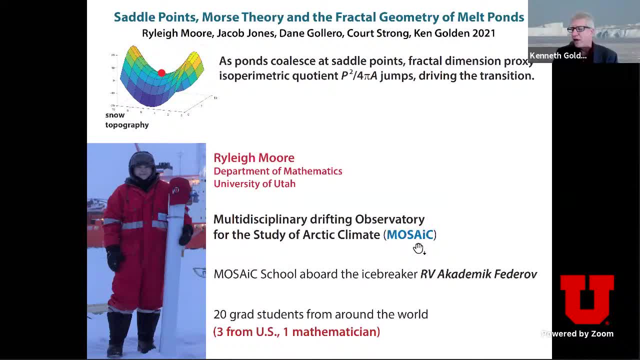 Drifting Observatory for the Study of Arctic Climate, or MOSAIC, which just ended this past fall, And again there were only three students from the US. but there was only one student who was chosen, who was from a math department, and that was Riley. 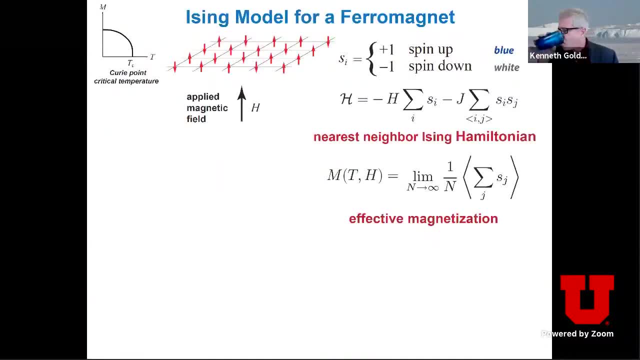 Now, one of the models that we were most excited about is adapting a 100-year-old model that was designed – that was built to understand magnetic materials, so-called Easing Model, And we've adapted that to study and predict the distribution of water, the geometry of melt ponds. 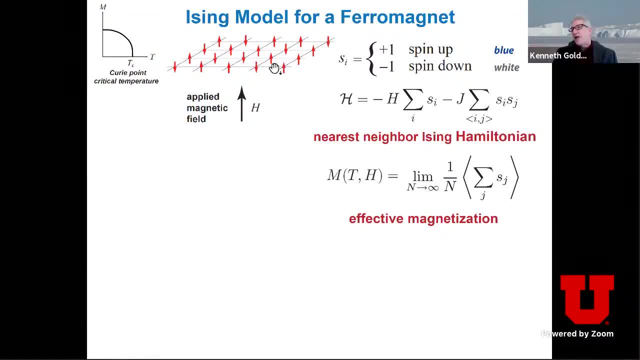 So this model starts out with just a two-dimensional lattice again of spin, spin up or spin down and little magnetic moments. And then this is a cartoon for the energy of the system, how the spins interact with an applied magnetic field and how they interact with each other. And one. 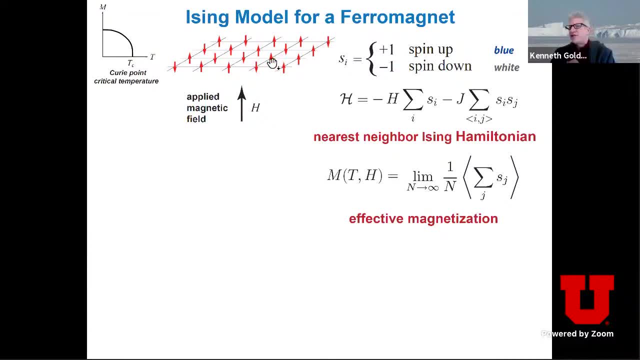 of the brilliant aspects of the model is its nearest neighbor. In other words, yes, the spins really interact with all the other spins, but you truncate the model, the Hamiltonian, so that it only – they only interact with nearest neighbors. And then the order parameter, the homogenized. 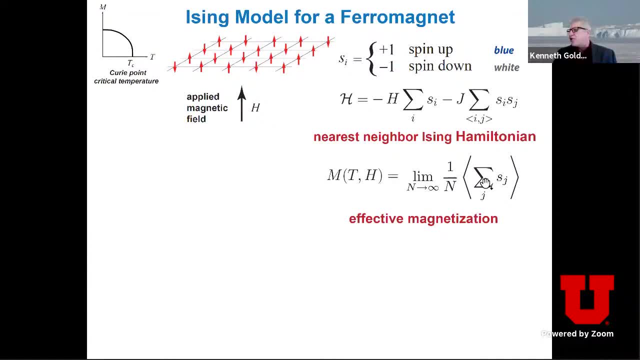 parameter. the overall bulk behavior is measured by the magnetization of the average spin. and now one of the main, one of the main ways locally of lowering energy- and that's what the system wants to do is lower its energy- is to for spins to align locally. in other words, they want 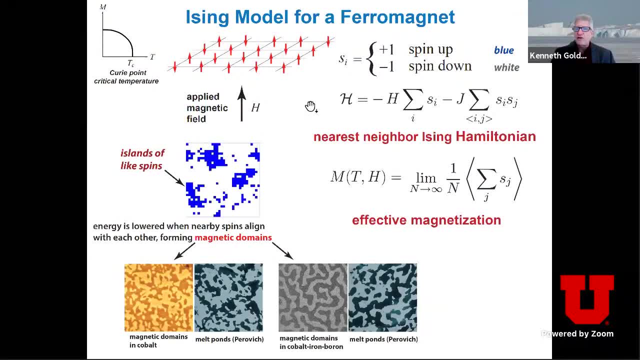 to line up, they want to be like each other and so you get these clumps, these little islands of like spins. and i simply noticed that these islands of like spin are very similar to how water overall wants to settle in these little troughs in the snow topography to lower gravitational energy. 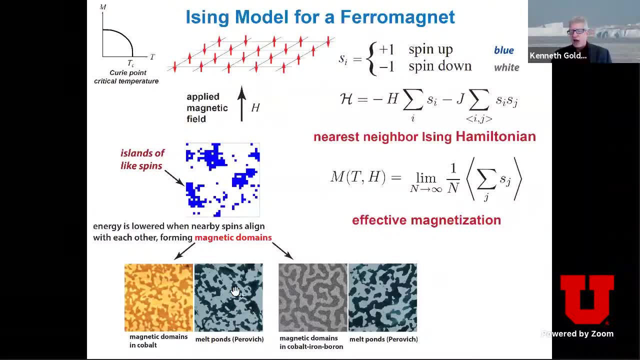 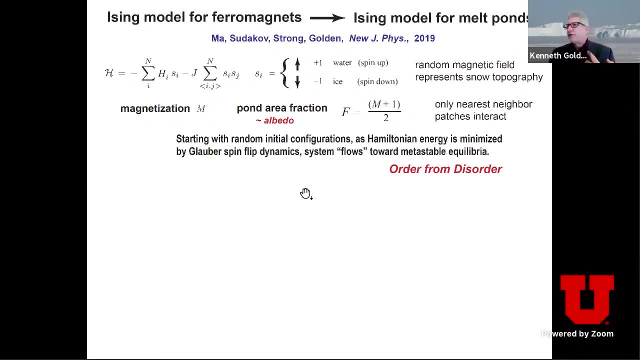 when the melt ponds form. so here we just side by side. i think it's very interesting how they look so similar magnetic melt ponds versus magnetic domains, and so we then adapted this easing model. so, instead of spin up, spin down, it's it's water and ice, and then the random magnetic 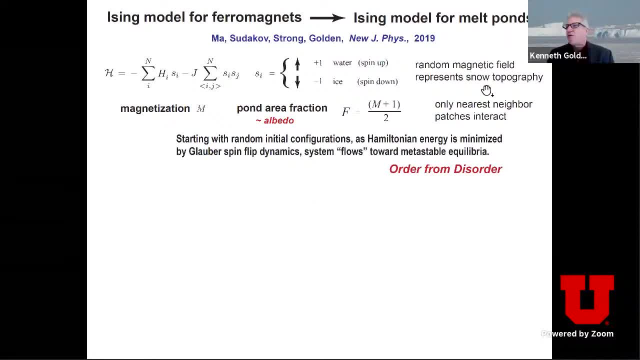 field instead of a uniform magnetic field, represents the random snow topography and then the homogenized parameter. the magnetization is then related to the pond area fraction, which is the albedo, and we start from a completely random initial configuration and then we lower the hamiltonian energy by so-called globular spin flip dynamics. 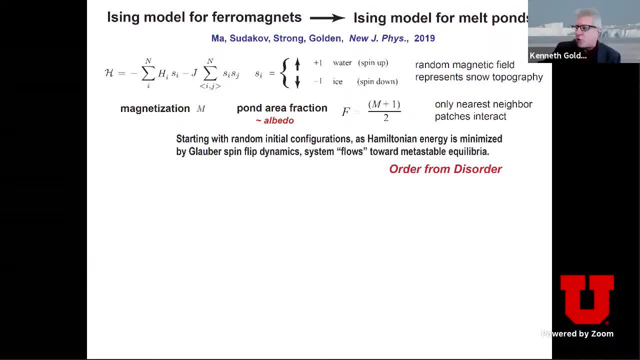 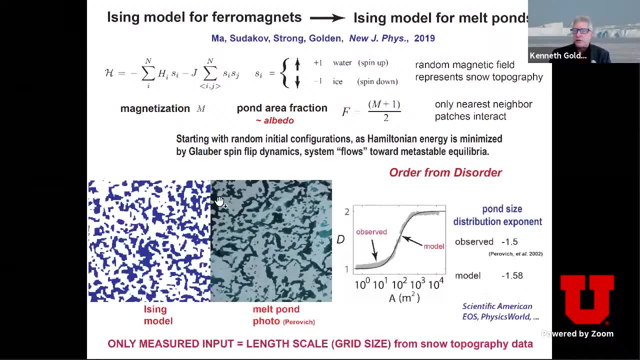 the system flows toward lower energy states, toward local energy minima, and they become more ordered. and then, amazingly, the the the minimal energy states are ponds. these are our ponds and our melt pond easing model, and to me they look very, very similar to real melt ponds and kind of also, surprisingly, there's um only one measured input that we put into the model. 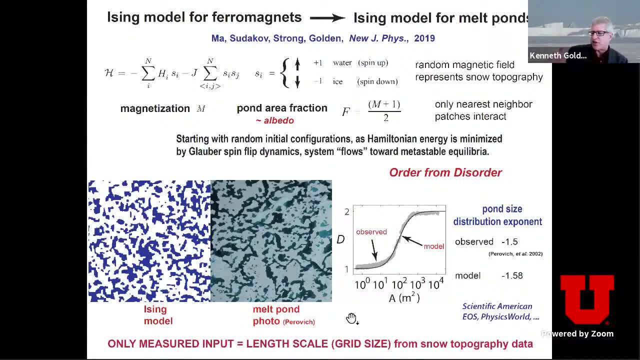 and that is where we have to relate the, the scale, the size of the, of the grid size, to the um, uh, to actual reality, and we use that by analyzing snow topography data and with that one observed parameter, measured parameter um, we match up beautifully with the fractal transition as well. 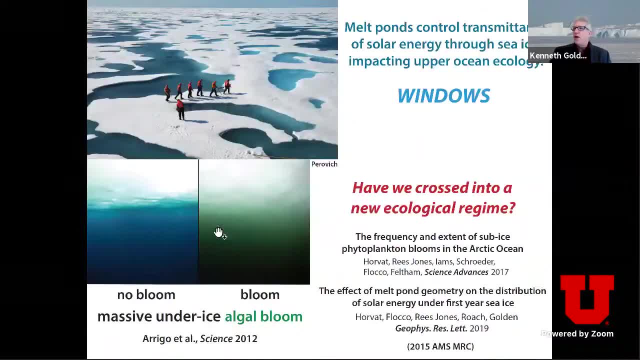 as the sizes of the ponds and so on. um, now, these ponds control transmittance of solar energy through sea ice, which impacts upper ocean ecology. they act like windows allowing light to the upper ocean, and one of the things that was discovered just very recently, about 10 years ago, was not a bloom, a massive bloom not out in the 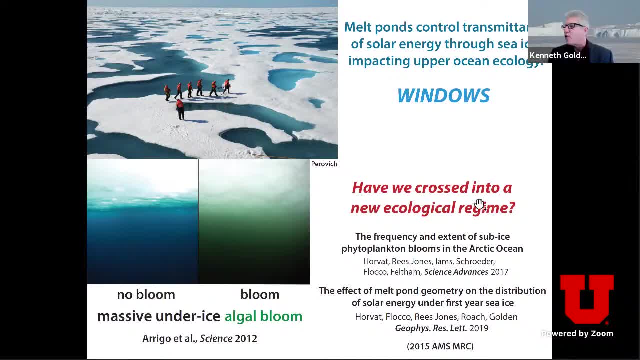 open ocean but underneath the sea, ice. so have we crossed into a new ecological regime and i was asked in 2015 to run a american mathematical society mathematics research community up at snowbird for 40 years and i was asked to run a mathematical society mathematics research community. 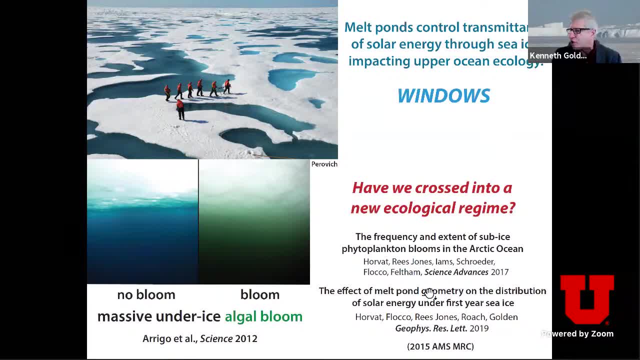 up at snowbird for 40 years and i was asked to run a mathematical society, mathematics research community, graduate students and postdocs to immerse them, and some of these really interesting publications came out, such as the frequency and extent of sub-ice phytoplankton blooms in the arctic ocean. 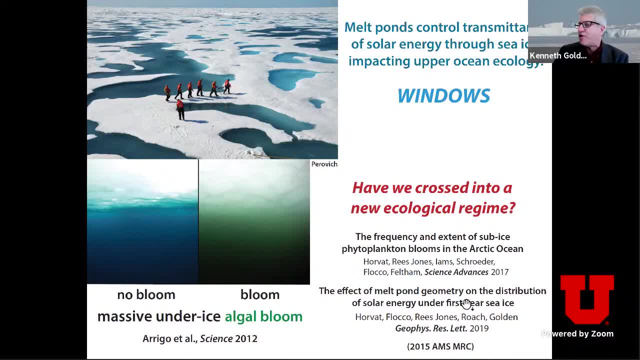 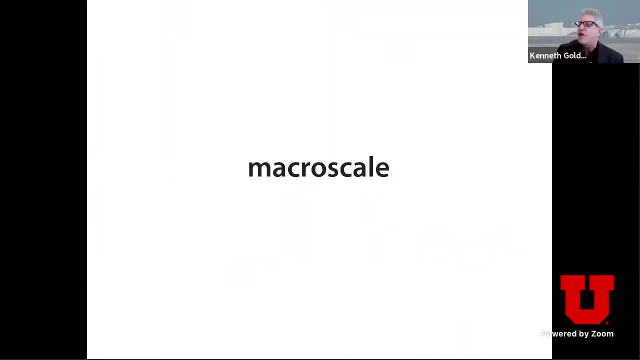 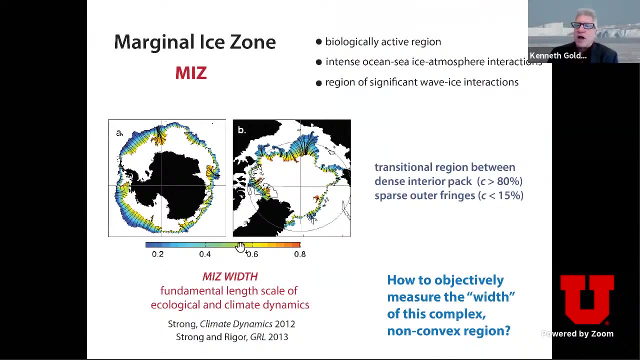 and something more recently, about looking how the geometry of melt ponds influences the under ice light field. now, finally, the last thing i want to mention is some of just briefly, is um some of our work on the very biggest scales, on the macro scale, and so this is about looking at. 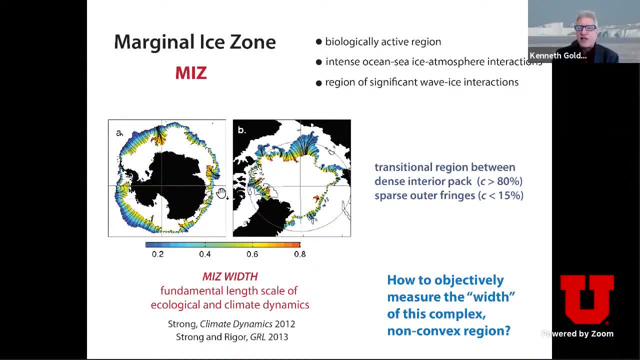 um the so-called marginalized zone. so now you can see we're at the biggest scale and we're at the, that's the antarctic continent. this is the entire arctic basin and the marginal ice zone is this colored in region, from the outermost fringes of 15 percent down to the inner core of 80 percent. 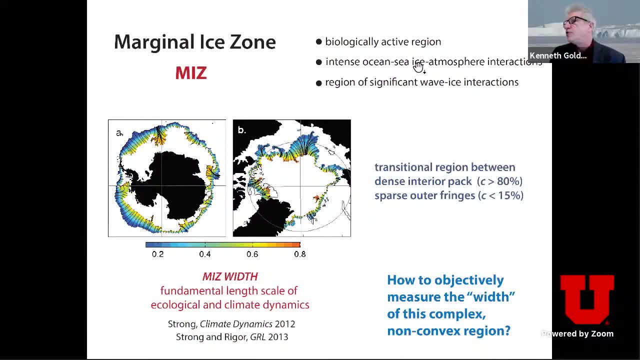 it's a biologically active region. you have intense ocean ice atmosphere interaction and significant wave ice interactions, and but but one of the a very big challenge is well, this serpentine, crazy, non-convex region. how do you get an objective measure of its width? and this is 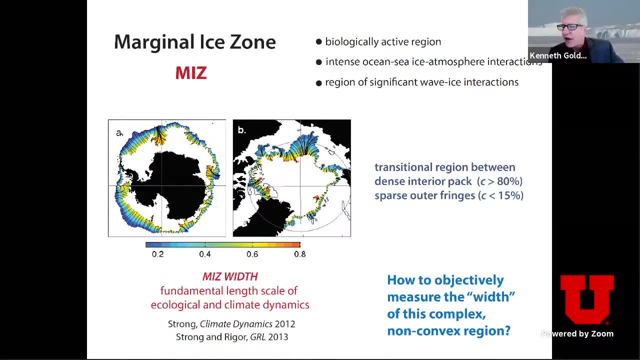 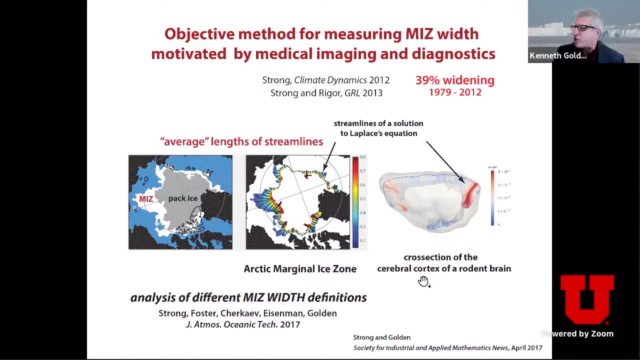 what court strong. our very close colleague in atmospheric science has figured out just a brilliant way of of of objectively measuring this width, and it was motivated by medical imaging and, in particular, measuring the cross-section, the, an objective measure of the cross, the size of the cross-section of the cerebral cortex of a rat brain, and the idea was to solve laplace's equation. 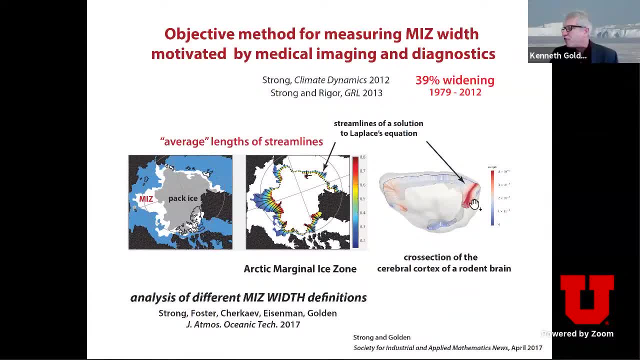 a simple one of the simplest partial differential equations for, like the electric potential, and then you can go around the whole thing and measure- and that's exactly what court did here- and you can get an objective measure then for the, the width of the marginal ice zone, and he found that that that 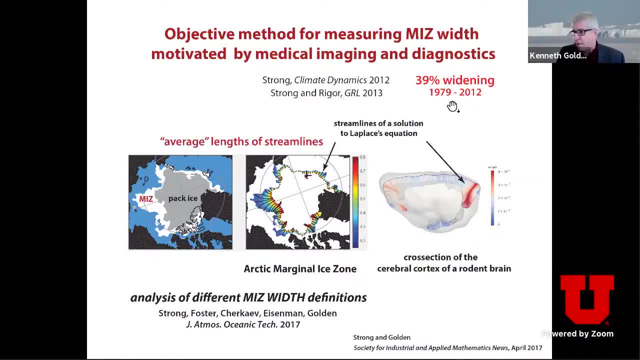 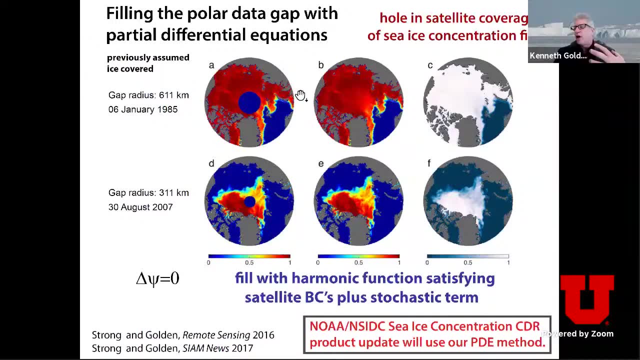 widened by almost 40 percent as our climate has warmed, and then, using similar, these same kinds of ideas, we've then adapted that same kind of- um, uh, simple, simplistic model for the sea ice concentration field to fill the whole thing. and that's exactly what court did here, and that's. 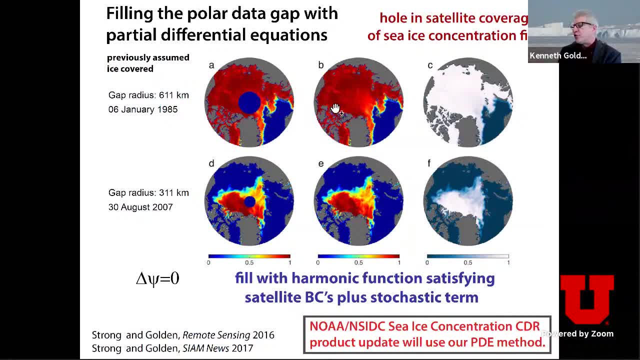 what we're going to do is we're going to apply this method to the polar data gap and with just a simple solution to the steady state heat equation, taking into account the boundary conditions that are given by satellite data, and then measuring the stochastic variation nearby and incorporating that, and then 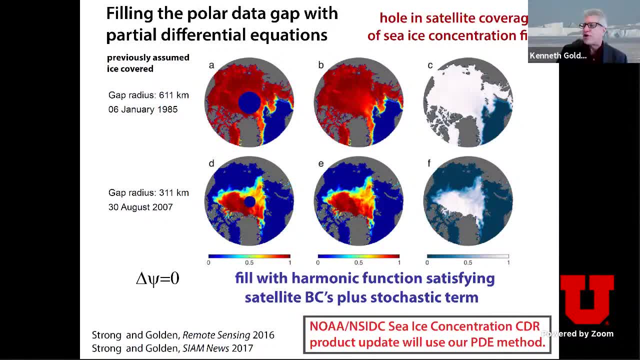 we get a really effective interpolation for the polar data gap, um, which is now, uh, going to be used. we believe in the national snow and ice data center, in their sea ice concentration um data product, for the um, their climate data record. so we hope that, again, that our, our work is having a- you know, an- impact on these larger. 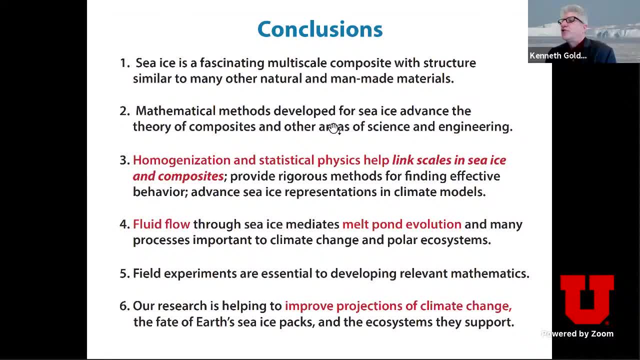 scales. so, in conclusion, uh, sea ice is a fascinating multi-scale composite with structures similar to many other natural and man-made materials. um mathematical methods that uh are developed for sea ice also advance the theory of composites and many other areas of science and engineering, and, in particular, homogenization and statistical physics really help us link these scales in both. 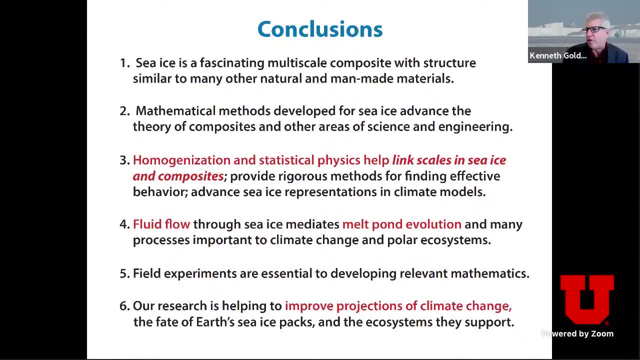 sea ice and, more generally, for composites, and ultimately provide rigorous methods for finding effective behavior and advancing how we represent sea ice and climate models, and, in particular, fluid flow through sea ice mediates melt, pond evolution, as well as many processes important to climate change and polar ecosystems. 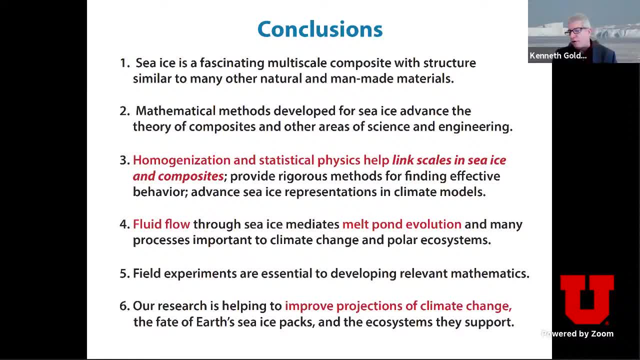 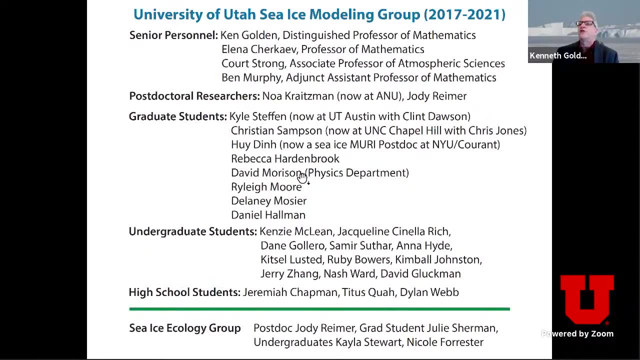 and, from my perspective, these field experiments that we are involved in are essential to developing mathematics that's particularly relevant to the system at hand. and, ultimately, we hope that our research will improve projections of climate change, the fate of earth, sea ice packs and the ecosystems they support. and so, just over the past four years, all these people, wonderful, my 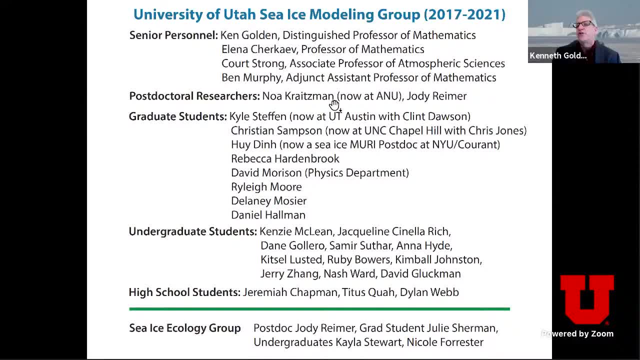 colleagues in the math department and atmospheric sciences, as well as postdocs and graduate students who wound up wonderful places, and so many wonderful undergraduates from many different departments- uh, even lots of high school students, um, as well as we have this emerging sea ice ecology group. i just want to thank them for doing all the work and being such a wonderful colleagues. 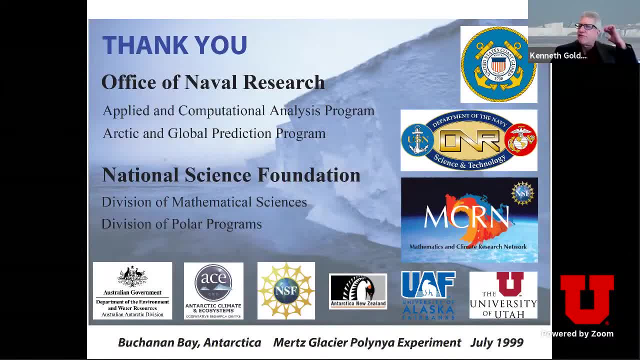 and supporting this, our research efforts, and also thanks to the office naval research and national science foundation for supporting this research and all the countries and other institutions that help, in particular to the university of utah, who has been so supportive, our administration and so on, has been so supportive. 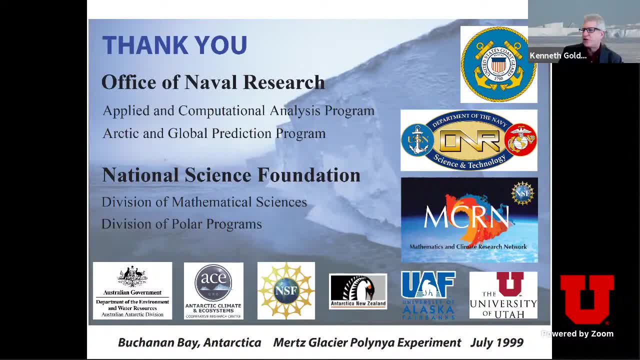 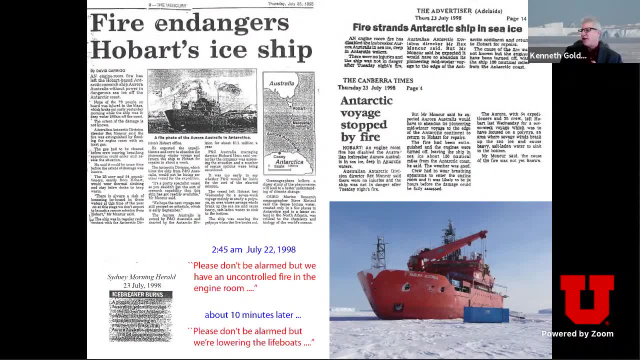 of of our research program. and finally, just to bring this all to full circle, you heard that first story about laying out on the ice and measuring some very thin ice. and well, my one of my trips soon after that was my first trip with the australians- and about 237- the fire alarm goes off just as we're. 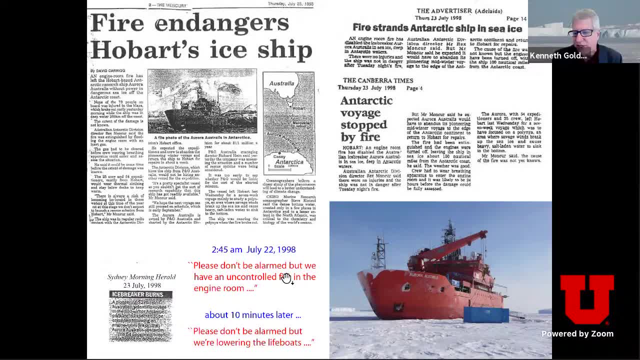 inside the ice pack. and then we all have to muster out on the fan tail. and it's well, please don't be alarmed. but we have an uncontrolled fire in the engine room a few minutes later. it's well, please don't be alarmed, but we're lowering the lifeboat. so here i am, a mathematician. i'm thinking, oh my. 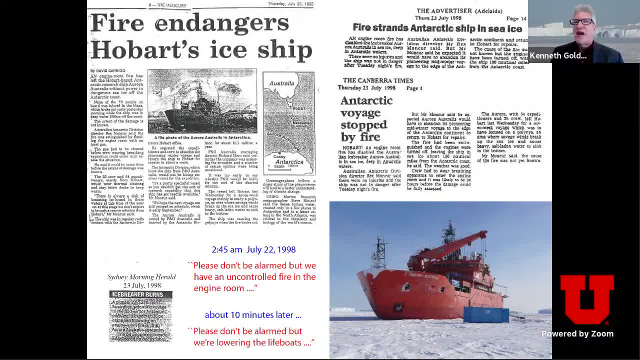 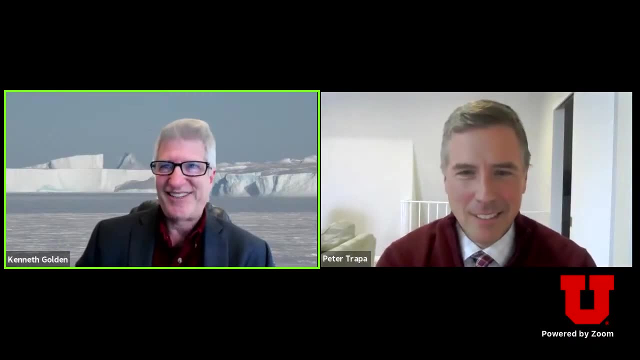 goodness, i prove theorems for a living. what am i doing on a burning ship in antarctica? and anyway, um, obviously i made it back, but uh again, thank you so much all for your attention, and with that i will turn it over to peter to uh answer, to ask questions and so on. 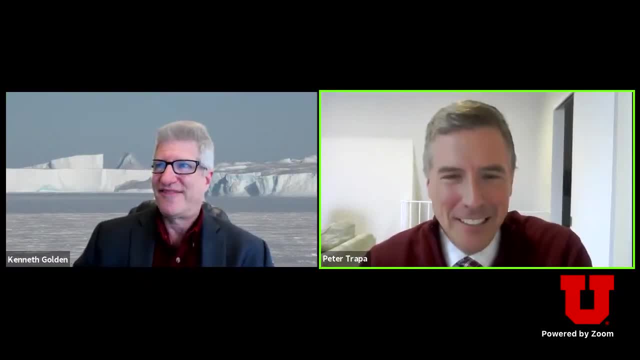 well, thank you, ken uh, for that fantastic presentation and video that preceded it. uh, i'm reminded when i listen to you every time how inspiring you are as a speaker, and i miss the days when we used to walk, walk the halls together and i'd bump into you. 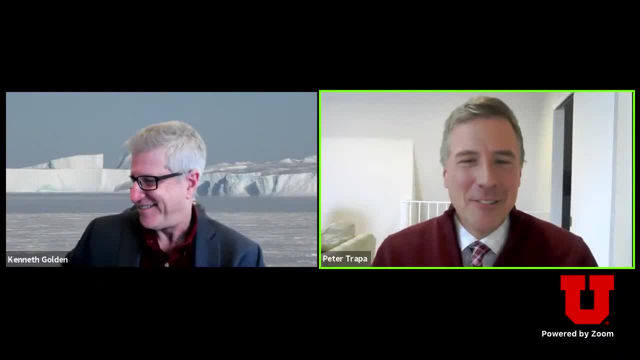 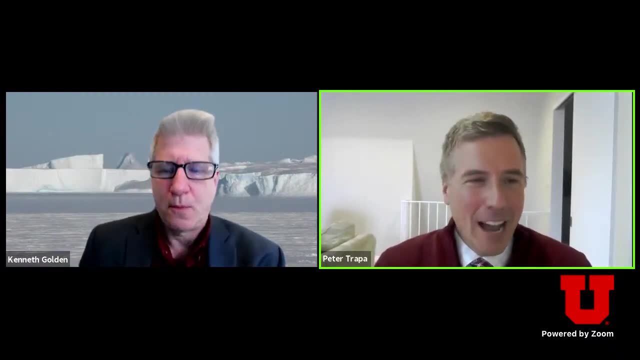 and i'd get inspired by you that way, so i'm glad that we still can do it in this format. um, you know, your talk touched on so many different things. uh, i i'm afraid that we're not gonna get uh a chance to even uh skim the surface, so to speak, because we we do have a hard um stop time at. 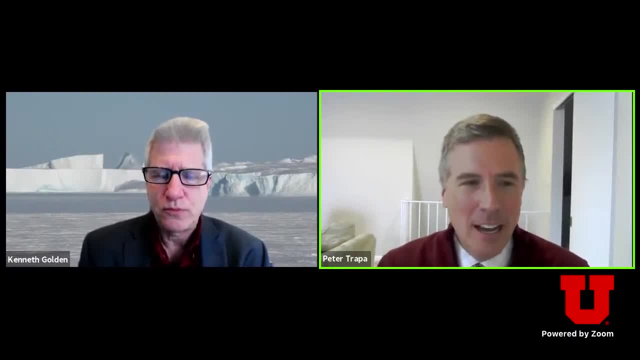 one o'clock, but i want to get to a couple of key ideas that emerged, um, and the first one really gets back to that cross pile pollination slide. um, you know, that was the one where you you started with this central question about understanding sea ice and you talked about this incredible array of 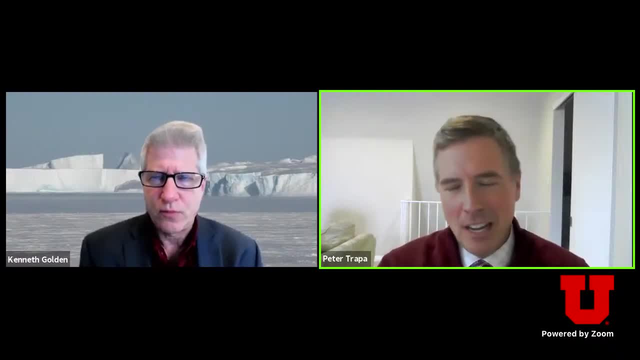 techniques from everything from stealthy technology originating electrical engineering and extractive industries all the way to more traditional areas of mathematics like stochastics and functional analysis, complex analysis that you. you incorporated that, that huge, diverse collection of techniques to attack the problem, and then what came out from that analysis had 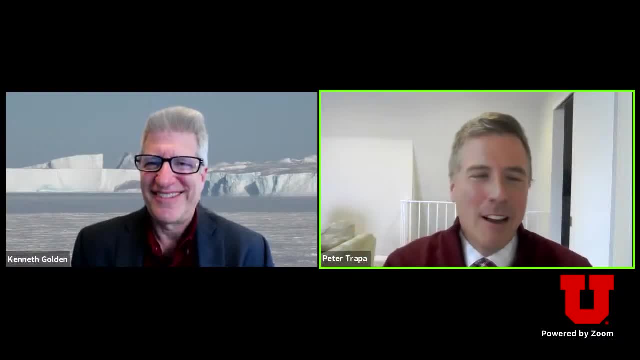 applications to in completely unexpected directions, like the porosity of bones and detecting um bone diseases like osteoporosis. so you know, this is something that everybody wants. this is a model for doing interdisciplinary science. it's what everybody wants to do and they want to understand how to do this. i mean, it's not only about doing science, it's how do you attack public policy. 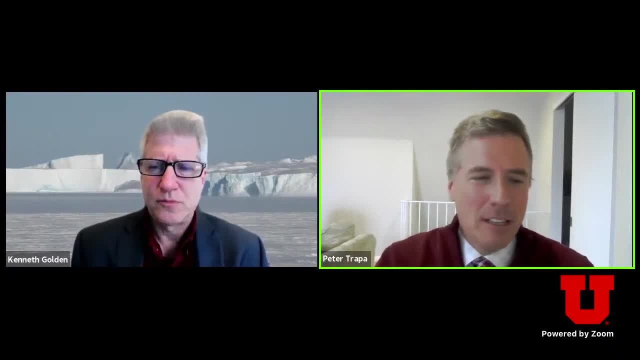 questions. or how do you, how do you attack problems in business or economics? you know you, you have this problem. you need, you need to marshal all these different techniques and to attack it, and some approaches are very deliberate. they assemble these large teams that have you know someone from. 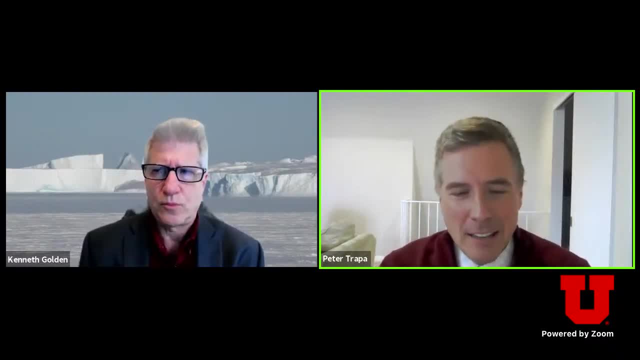 geophysics, someone from electrical engineering, someone from mathematics and, uh, others. other approaches are just more organic, that they sort of grow out of just um chance interactions like hallway interactions and conversations of that nature. so i wonder, how do you approach interdisciplinary science and you've been so successful in so many different um domains? uh, 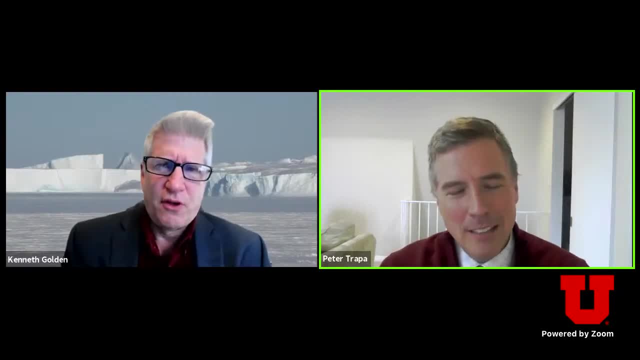 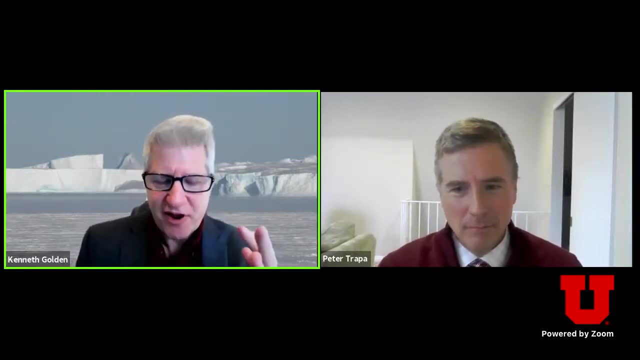 is it deliberate? do you approach it deliberately in that kind of form or way that i sketched, or is it? is it something that just happens organically? yeah, that's that's a really interesting question and i think i i actually have, i think, kind of an answer to it. 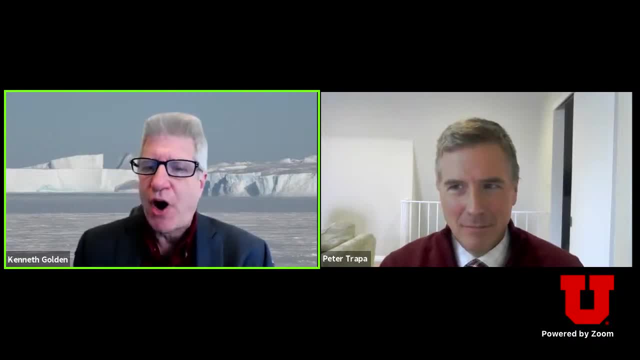 um, as i think back over, you know, over the course of my career, because you know i was trained, um, as a mathematician, as a mathematical physicist, and so certainly the ma, the main mode of working then 35 years ago is, you know, you're a single author, you have single author papers, you're mostly 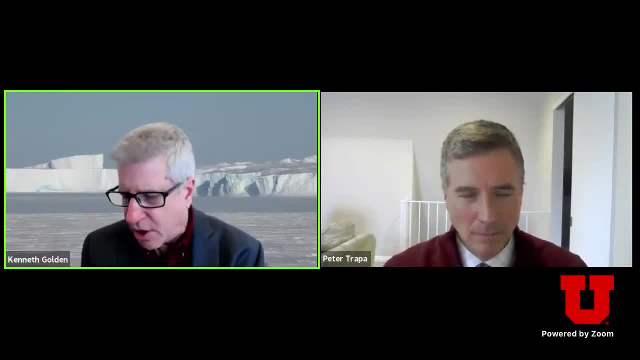 working by yourself. you're working for. you're mostly working by yourself. you're working for fact-checking, Fascination, turbo tailors. you're mostly working included in the physical imagination. you're doing what's called 멓, that and as a 첦. how do you deal with that right? 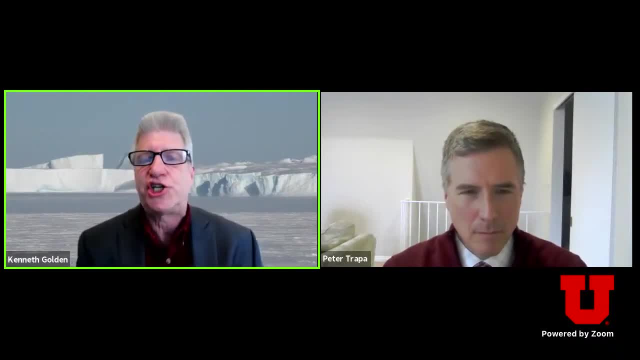 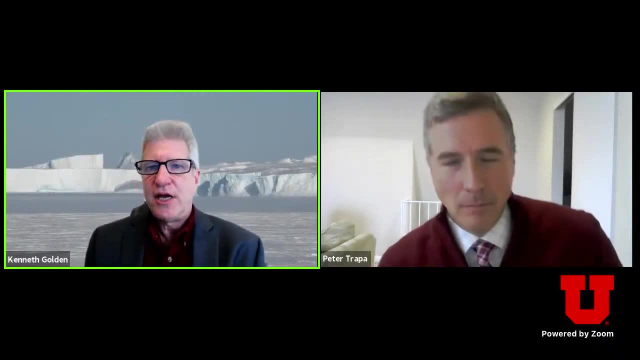 like, like the all the. so that was an interesting question for me. but, um, with hudson, you, you, your, your way of thinking i'm, as a mathematician, you're more water school student, i'd say, than the, the scientific inches of gaat. did you ever feel like you were just going on an arctic expedition? 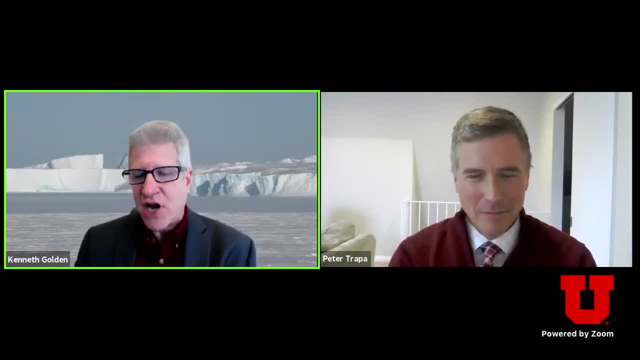 or did you work on an art? you did you work on occasion in? You know you're living. you're literally living, not just working with going- you know to go into work, but you are literally living with, say, 50 other scientists, physical oceanographers. 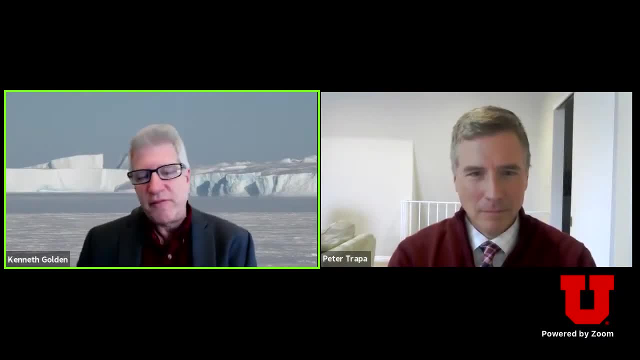 biological, oceanographers, glaciologists, electrical engineers, mechanical engineers- you know all different kinds of scientists- And so you start to get exposed to that kind of way of thinking and all this incredible interaction. And so then I guess, as I got more and more, 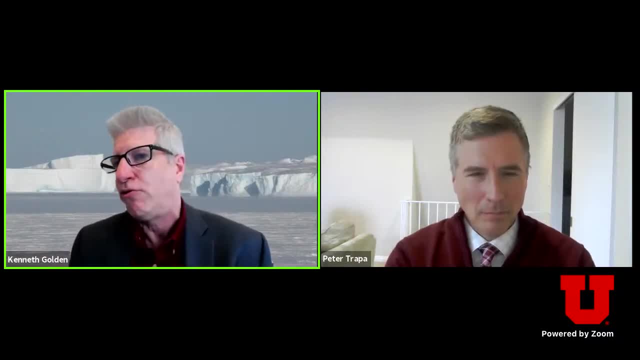 involved in sea ice. but there was also another critical step in my evolution in terms of having more of a group type of approach and being so highly interdisciplinary and working with so many other people, And that was undergraduate research. In other words, when we got the 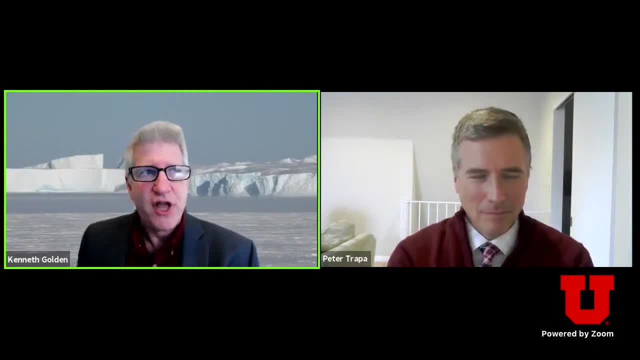 vigor. you remember that when we got the vigor from NSF, there was all this money for having undergrads, And so my first two were in physics and chemistry. And you know, and that started like hey, knock on my door. Hey, Professor Golden, I was in your. 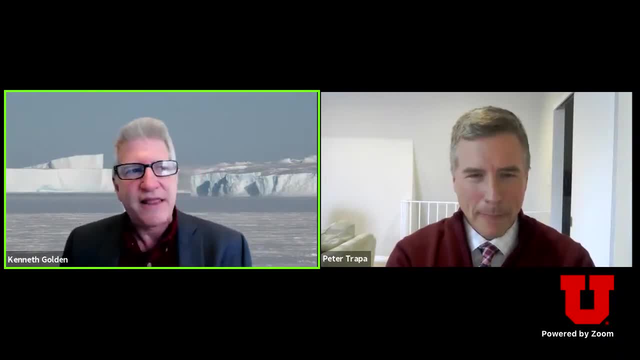 calculus class. Can I do some research with you? Yeah, sure, Let's go. And that started to get me thinking. it's like: oh, there's all these different facets to this research. We can have people working on this or that, or, you know, undergraduates analyzing data, or very sophisticated. 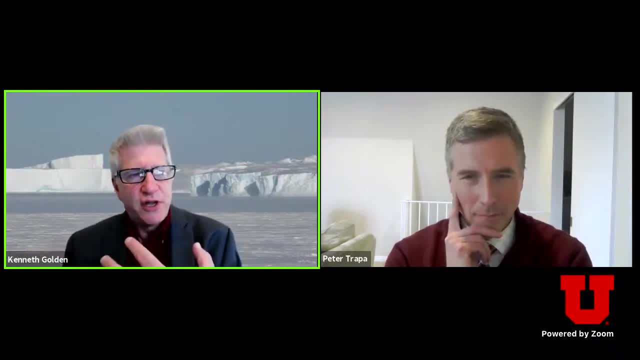 programming or very theoretical types of things, And so it started to become apparent to me that there were so many different facets of this, that. but then it started to grow organically. Then you know it's like: okay, hey, here's a natural thing, Let's, let's try to recover the brine volume. 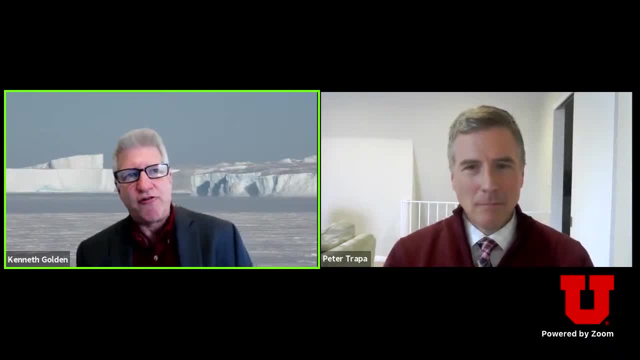 fraction. What's going on inside the ice, you know from bulk electromagnetic data. Well, Lena is a world-renowned Lena. Cherkayev is a world-renowned expert in this problem, as well as Graham Milton and my colleagues here at Utah. So okay, You know it just like hey. 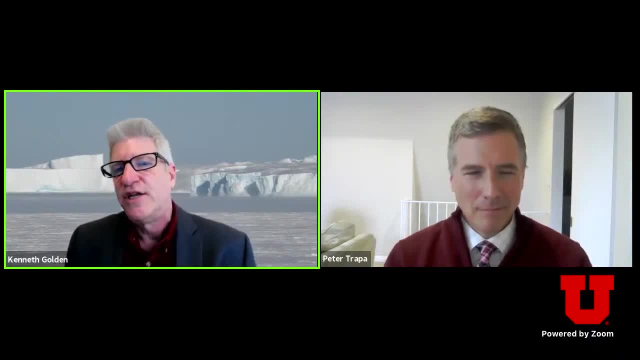 let's talk about it, you know, and then that just sort of evolves And so so it's been. you know, for specific projects, specific types of goals, then you know it might be okay. we have this specific place we need to go, So we want to. 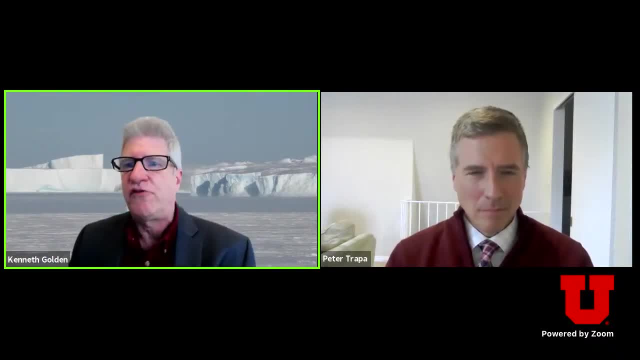 build a specific type of team And you know I've certainly been involved in that approach as well, but I'd say for my own career it's more evolved organically as you want to approach or type, attack a certain type of problem or, you know, do you know, do a certain area of research or get involved. 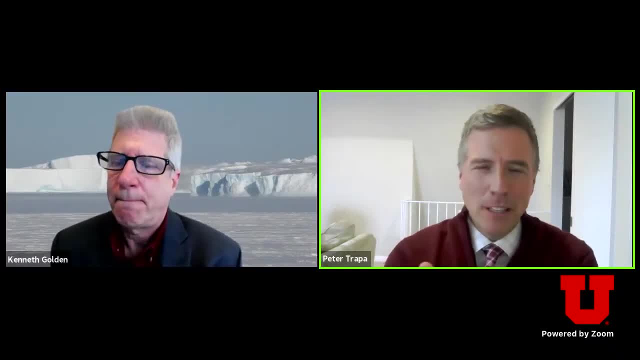 in a certain area of research. That's great And and you know I'm I'm so glad that you brought that up, that you involved in your research, because that came through your role as an educator came through so powerfully both in the video and in your slide top. And I want to spend a little. 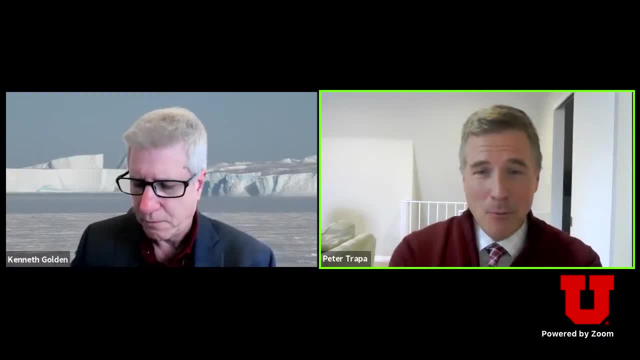 time on that. next for the: for the people who are watching this who don't know, I mean Ken is also very distinguished educator. He's recipient of our distinguished teaching award here at the FU, our highest recognition for teaching, And I do you know. the other day I was doing the. 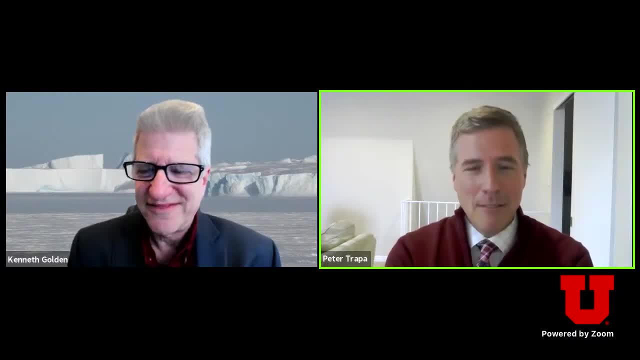 back of the envelope calculation of the number of students who've been through Ken's classes over the last 20 or so years, And it was. it was something like six or 7,000, because Ken regularly teaches these large sections of calculus and has has inspired. 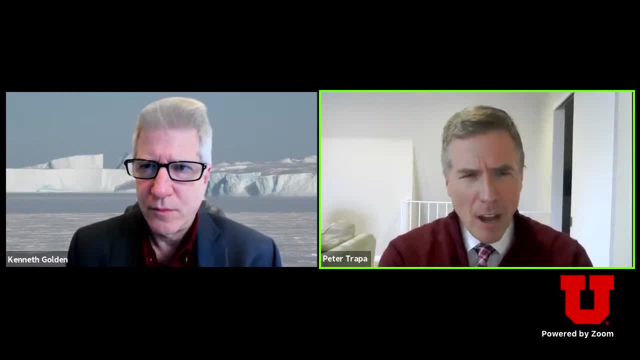 lots of students that way. So when you think about about your students and your role as a mentor and fostering the next generation of research in this, you know this critically important area. you know what. what is your philosophy about student engagement? 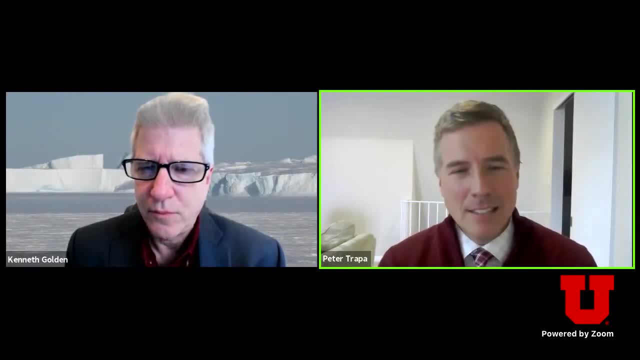 And mentoring, And is this a big part of your scientific legacy? the students that you're working with, say, in your research. Maybe you could talk a little bit to that. Well, certainly, you know, that is one of the things I'd like to be the most remembered for. 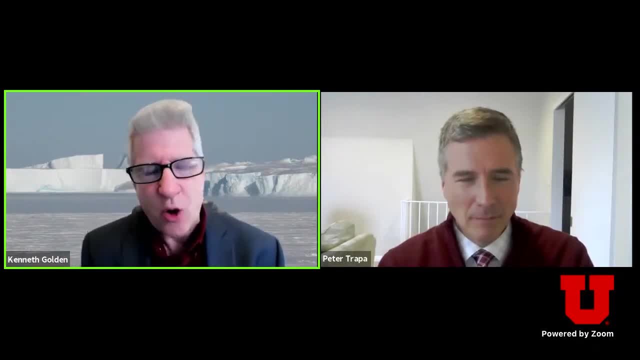 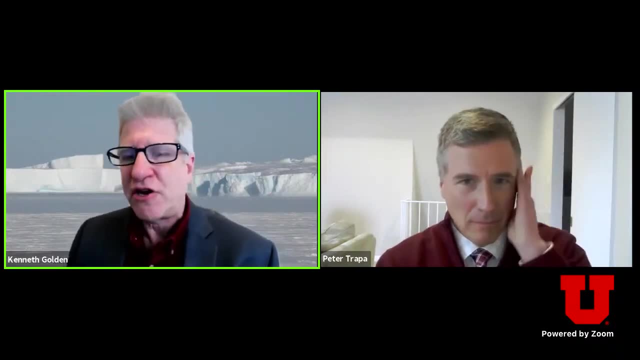 is helping lots and lots of students you know from calculus classes. helping, you know, students who might be afraid of calculus achieve their dreams of becoming an engineer or a scientist by, you know, getting them through calculus or something like that. So certainly, 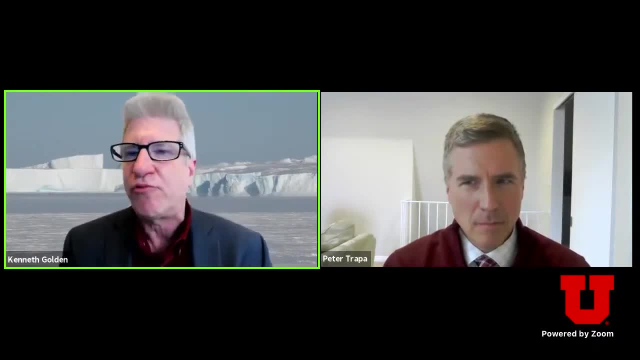 helping students achieve their dreams, but also in terms of getting them involved in research and getting them excited in research and showing them how interesting and fascinating and important, say, mathematics can be, even at these introductory levels, And so that's one of the sort of the first. 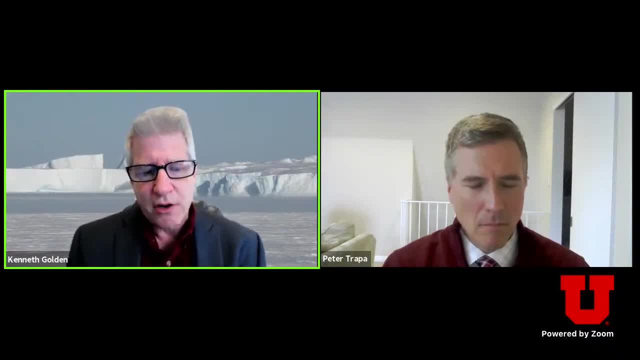 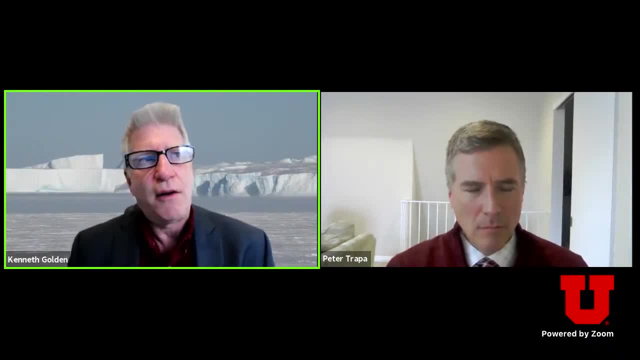 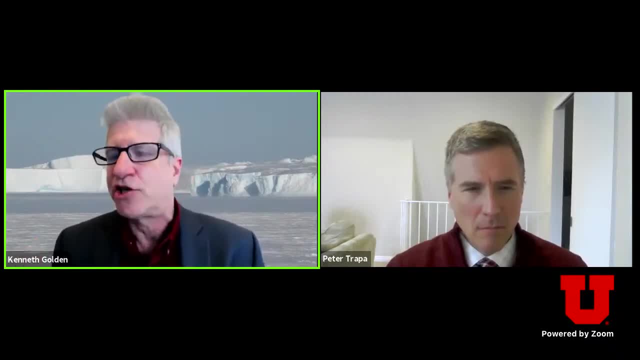 Antarctica, but also having that going on in the mathematics department, which is certainly somewhat unexpected, And I think that's important And I think that's really good for mathematics in general, And so I think that also is an incredibly important aspect of the mentoring process in. 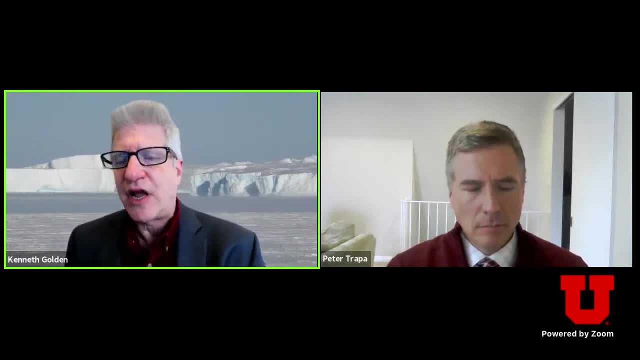 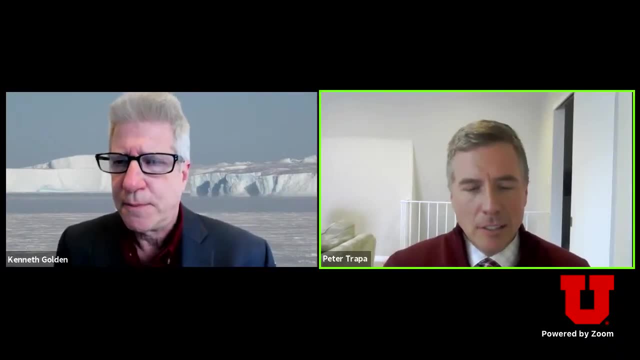 getting them to viscerally feel and see the things that they're trying to model and understand. I think that's- for me at least, that's an important component. Yeah, And you know, I'll just piggyback on that just a little bit, I mean the transformational nature of these research. 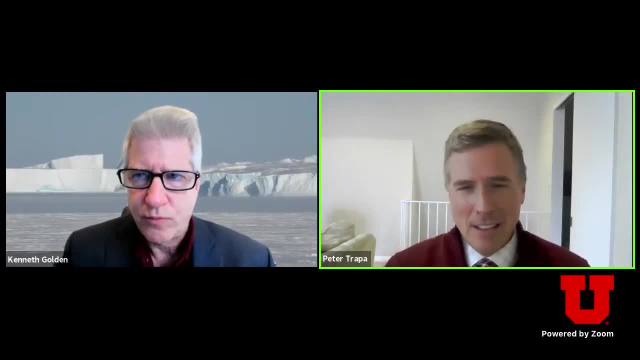 experiences that you're providing and many other investigators in the College of Science are providing. I mean, these are really so fundamental to the success of our students And you know there's a lot of hand-wringing about the future of higher education in the post-pandemic era. And one thing that is very 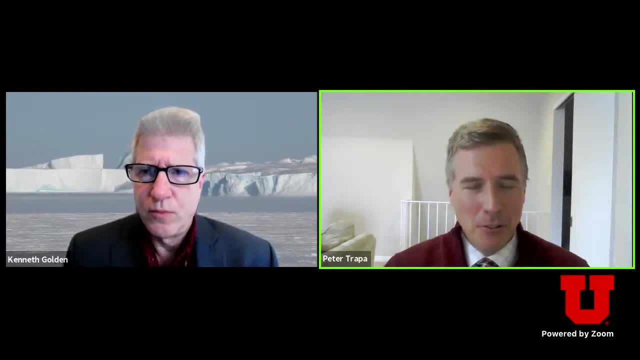 clear and very clearly will survive is that the experiential learning that happens in undergraduate research is one of the most important things for the future of science, and particularly the College of Science. That will never go away, You know. I want to turn to a question that came in on the 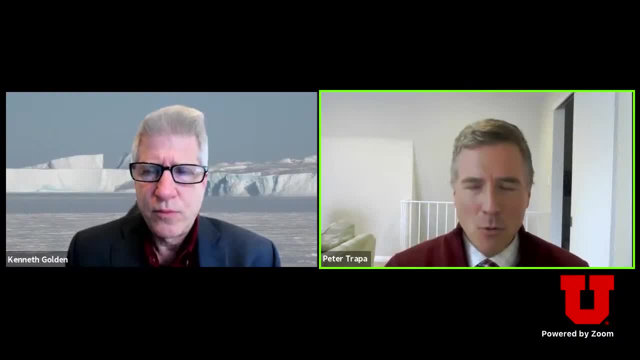 live chat. So someone was asking: you know what is the most important thing for the future of science, and not only for you but, you know, for your research group, And particularlyRES is asking how your work and the models that you're. 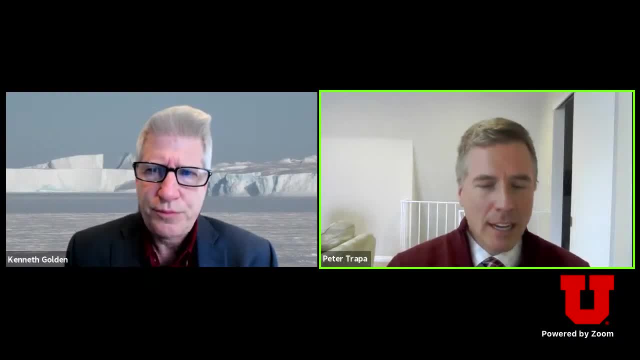 working on for sea ice are being incorporated into the climate models. You touched on that a little bit, And are you working on that directly, or is it the kind of thing that other researchers have picked up on your ideas and are applying them to climate models, or a little bit of both? 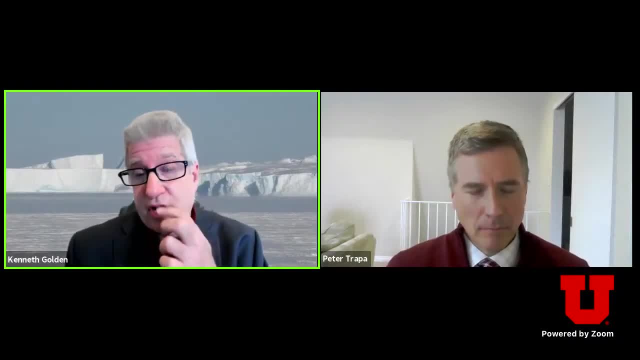 So maybe you could talk about how your sea ice research is being integrated in climate model research. You know we like, for example, our work on the fluid permeability of sea ice and these parametrizations and theoretical models that we've and these formulas that we've come up with. you know those are being used in melt pond, for example- melt pond parametrizations that are now being used in the most widely used model that comes out of Los Alamos. 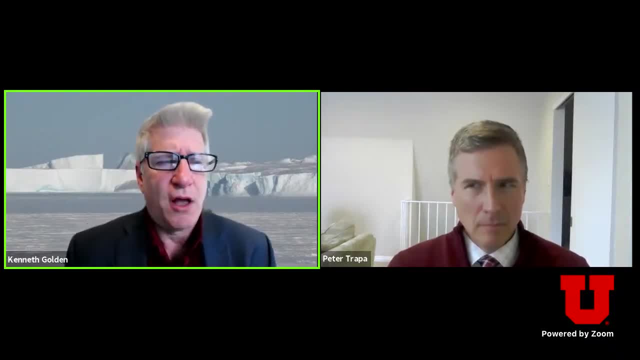 And so you know, but also some of our process studies, you know, have also been used in, say, other, you know. they then get used in other sorts of models of sea ice on, you know, on larger scales. 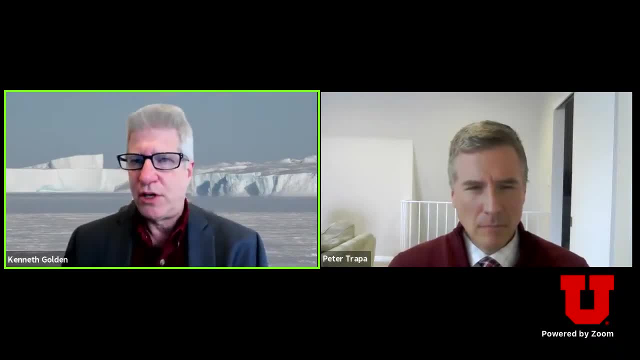 But also, but one thing in particular, this easing model. you know that we that I presented at the end, you know which is really sort of the these global climate models or the large scale sea ice models that go into the global climate models. they typically don't track where the melt water is or the distribution, which determines a lot of the aspects, but they're tracking the volume of the water.